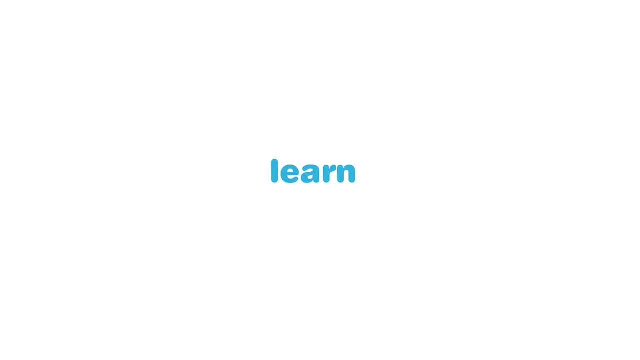 get started with the tutorial. So we will talk about an unsupervised set of learning algorithms. So you're going to hear discuss one of the primary methods of unsupervised. we're going to talk about what you call a K-means clustering approach. That's a very simple approach wherein we're going to try. 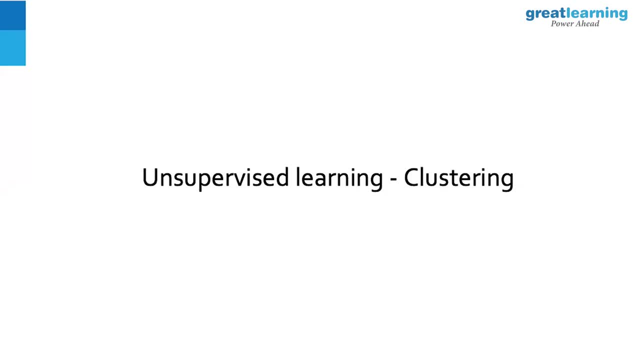 and objectively select a group of points that are closer and that are likely to be together. Right, That's the whole objective of K-means clustering, where we're going to try and put a certain set of points that are in patterns and put them closer together and set up the pattern. 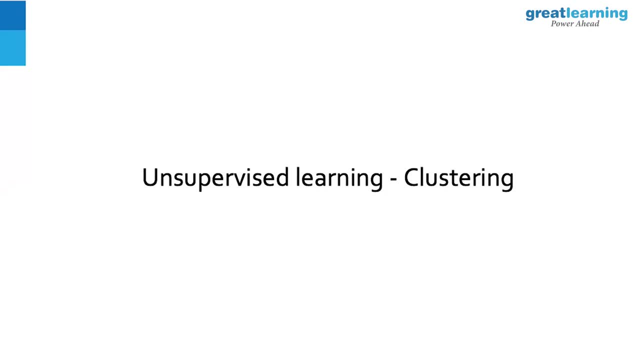 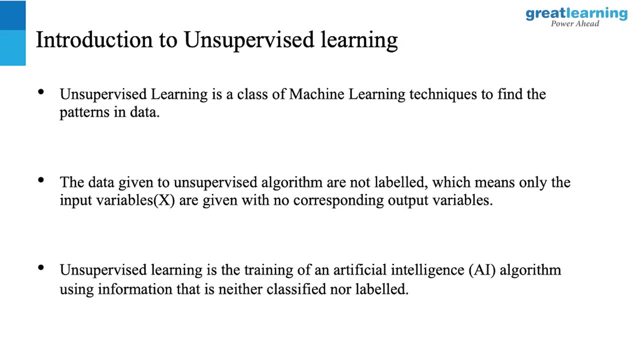 and say, okay, they belong to group one, they belong to group two and they belong to group three. That's effectively what we are planning to achieve, Right? Okay, Now, first up, when we have unsupervised learning, right, what's the primary and most functional, most? 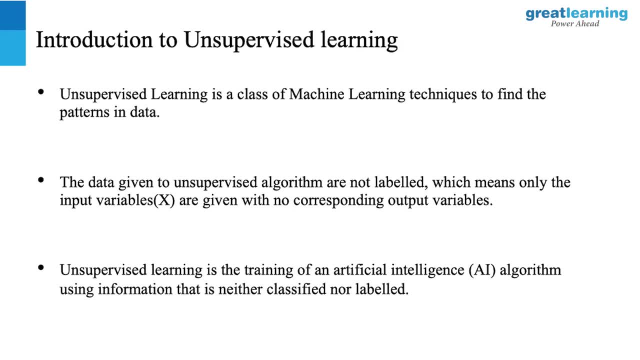 element is the fact that there is no target there either. Okay, Now let me give an example. Let's say we have data about students spending time in their respective subjects. Can I identify studious from the? from the weak students to some from the strong students? 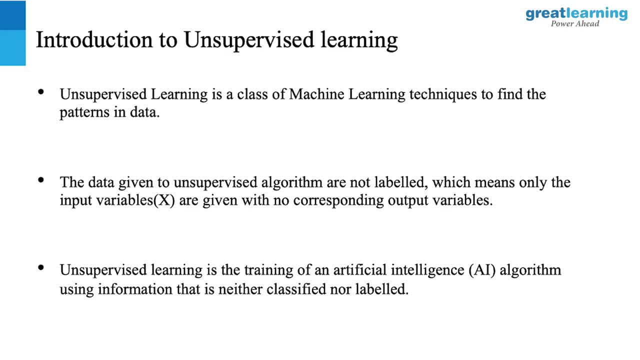 So that's an objective of K-means, that's objective of unsupervised learning. Well, I don't. I don't have a predefined target set, So what I have is just the time spent by students in the respective subjects. That's an example of an unsupervised learning. 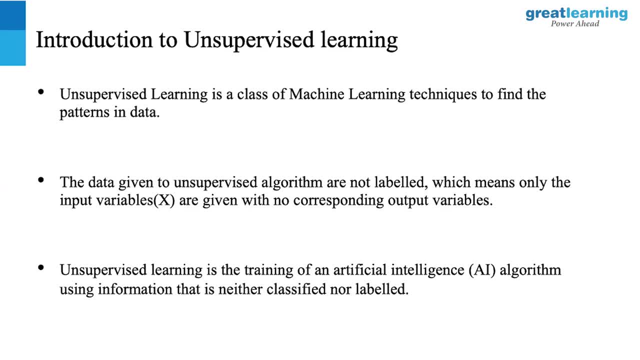 Another more commonly used example is: we have, in the marketing we call, a model that we call as RFM. It stands for Recency, Frequency and Monetary Values. Now, this RFM model is nothing, but how recently did the customer come? 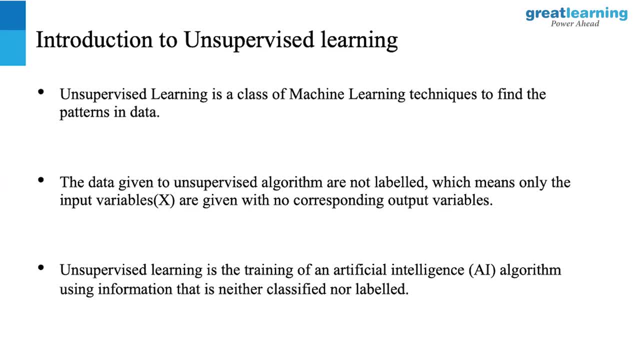 What is the frequency of his visit to my store And what does this monetary expense that he's spending on me? So that's an application. That's an application of unsupervised learning. So this is our cluster scenario, where in which we're trying to do a segmentation, not another approach. 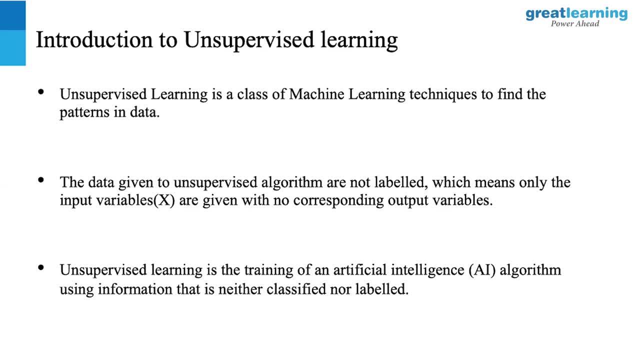 And we're also. another approach is a pseudo approach, where we're going to talk about image recognition is an unsupervised form of learning, where I'm not just trained the model to pick up information, but what I have is basically, I'm going to find a group of similar patches in data with a specific objective, with specific highlights in mind and clients, and cluster them and say, okay, they belong to this sort of a cluster of one which is a healthy or benign whom? careful when you're trying to make it? 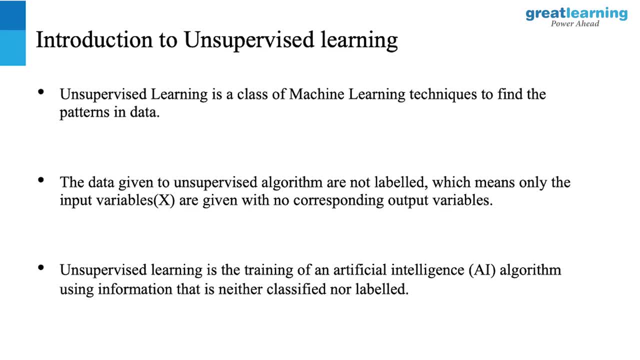 I'm going to find a bunch of these sort of stuff. I'm going to make it. I'm going to make it for you, Okay, Okay. So that's what we are doing. cluster now. so that's a combination of how unsupervised learning can be used for in multiple 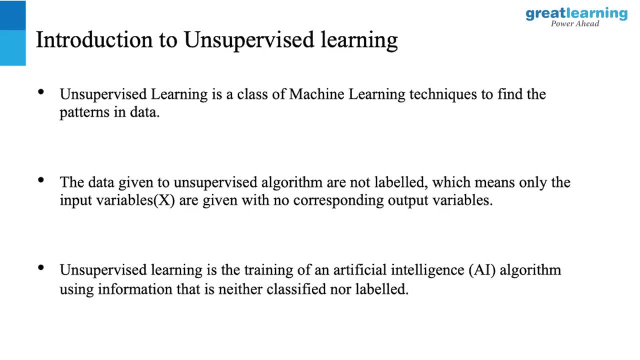 contexts right. the base is it's not classified or labeled. it's also where unsupervised learning will also talk about unstructured data. that's another level of complexity wherein we're going to talk about text-based analytics, so text-based information is also called as an unsupervised 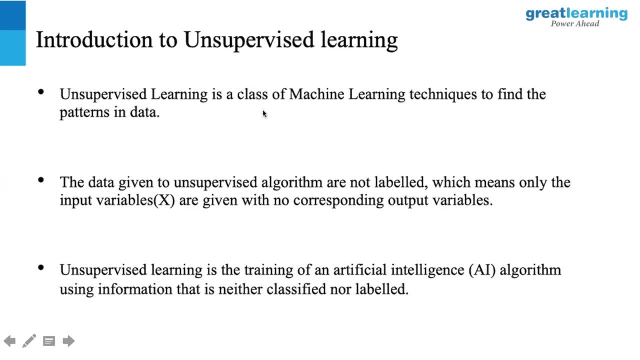 learning aspect. so anytime my target label does not exist, i call the situation as an unsupervised. so i'm going to find out patterns or groups in my data and then use these patterns and groups to implement. use these patterns or groups to identify these groups by a common center value and use my 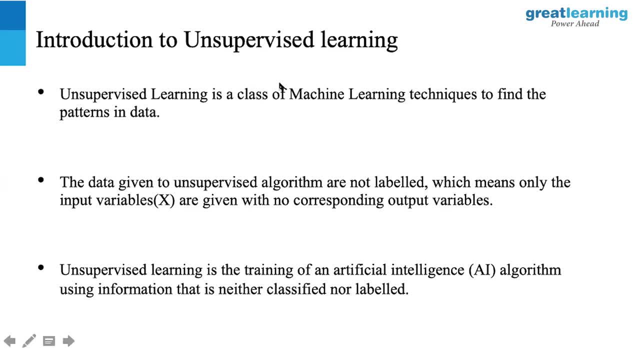 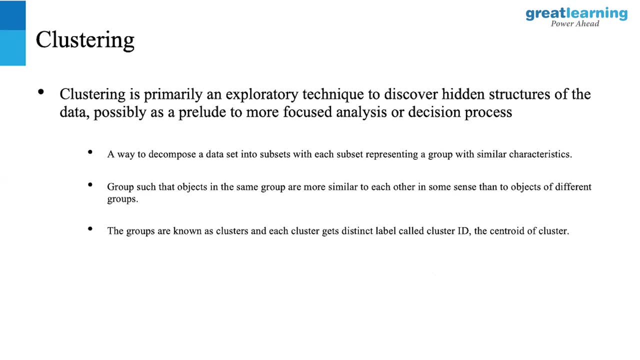 information around that center value. all right, that's. that's going to be my objective. now. one primary technique of unsupervised learning is what we call as a clustering technique. now, clustering is nothing, but i have group of data points that are together. i am going to group these points. 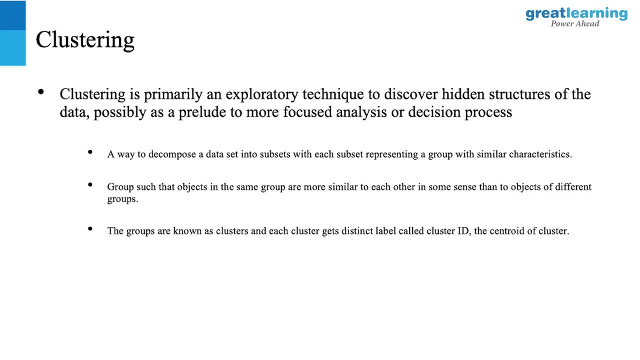 and i'm going to find a center value to these points and try and see if my entire group is responding or is a respondance of that group value. so that's a clustering approach per se. it's basically to fight to club or find out group of points. 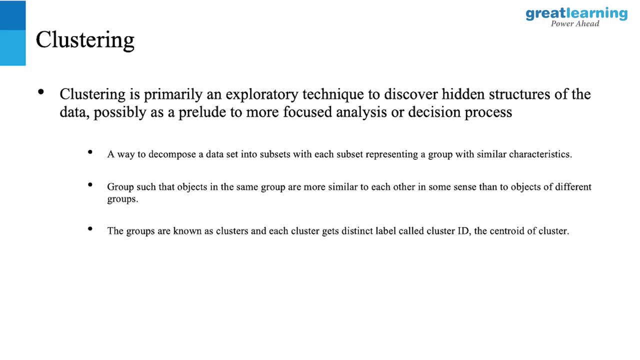 are similar together in terms of a pattern and put them together in perspective, all right. an example is: so let's say, i have data points here and i have data points here, all right, and i also have data points here. now i want to cluster these, these, these, these. 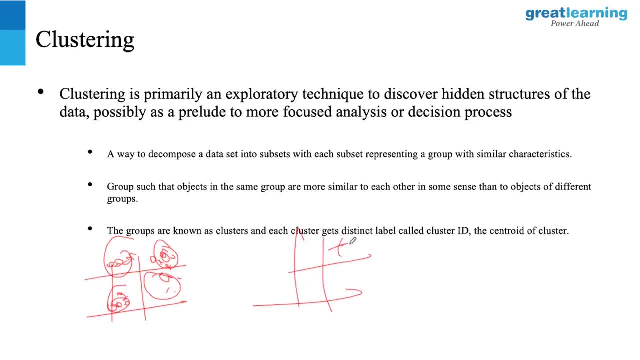 together in terms of my best and worst customers. i'll say top customers, i'll say weak customers, i'll say better customers. i'll say the best, the better customers again. so this is kind of a segmentation. can be achieved with my clustering technique. so basically take groups of data points. 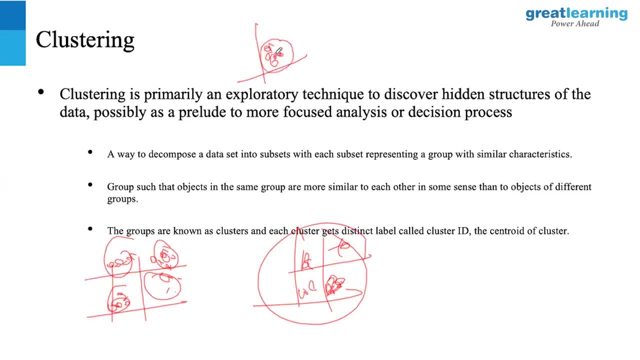 together and put them in a single cluster with the center value that represents the entire cluster. so group objects find similar objects, put them together, run this model. so that's what we call as a clustering approach. all right, any questions? just wanted to ask, like we say, that this is used in image processing as well as in. 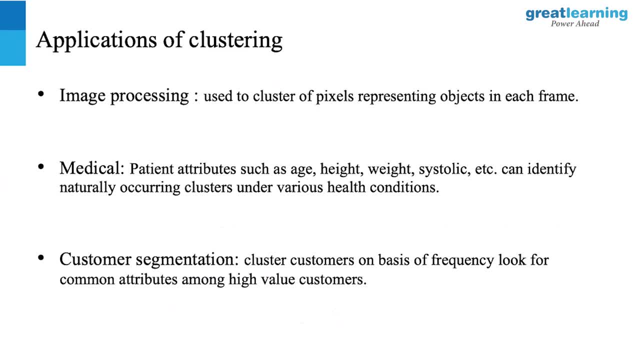 other other right. you just wanted to ask, like in image processing i talk about like, if i need to understand what the alphabet says and then i can. i have the whole set of data available with me so i can categorize it. but suppose, in case of i say that there's an 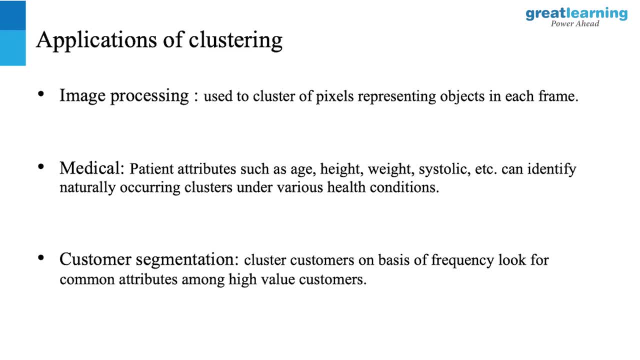 face recognition system. so then the the in production, there will be an unknown to it. so in that case, how it is differentiated? okay, so just one perspective to put into this. uh, nothing. so when you say image recognition, when you say alphabet recognition, so it immediately becomes a supervised learning. 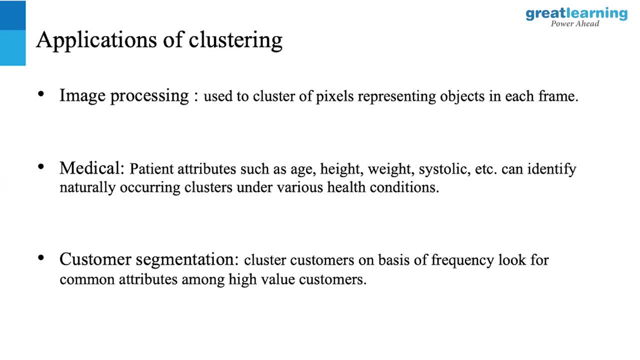 problem where i need to know that this particular design belongs to pattern a. now when we talk about unsupervised learning context, when we say image processing, basically i am trying to identify groups of objective points in a given data and analyze what they are. all right, i'm still have to still. 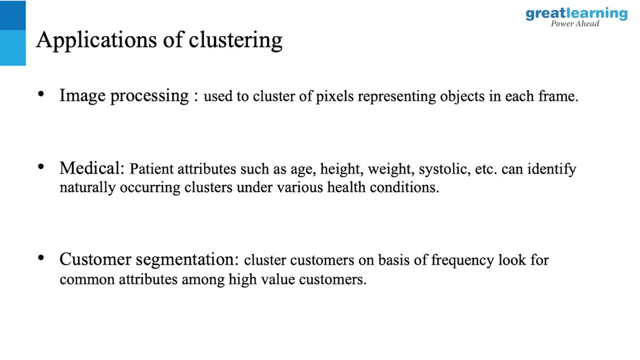 annotate them. what i am going to get from the clustering approach is going to identify. okay, these are the points that are similar together. what do they correspond to? these are the point. so, in in case of a medical recognition, medical image recognition, right? so if you have a tumor or a, 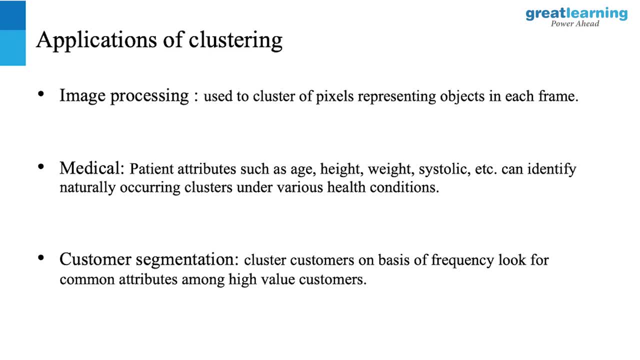 benign and malignant. so first let me identify patterns of objects that are together and then use that to see: okay, is this a benign, this is a malignant, how are they responding to? so first i didn't identify patterns and then work with these patterns. so that's what we essentially mean by. 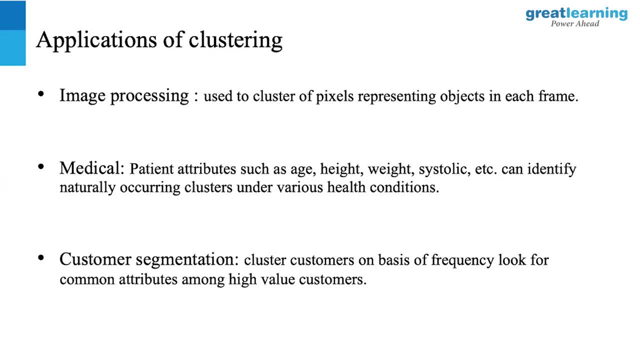 image processing or image recognition in a medical field. so for alphabet recognition it again becomes an immediate supervised learning problem. it's not more of a unsupervised, because i already have an information that this particular image belongs to digit a. i have this: this belongs to digit b. 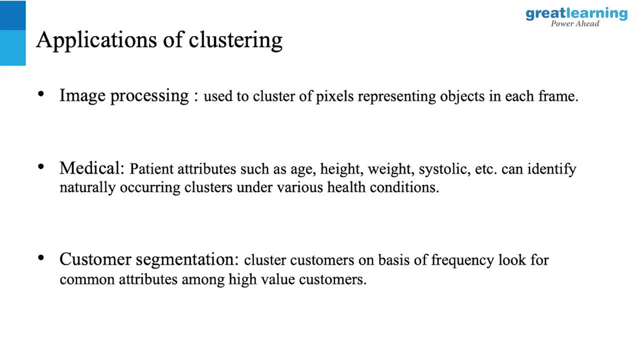 oh sorry, digit one, digit two. this belongs to alphabet a, alphabet b, so that becomes a supervised learning problem more than an unsupervised learning problem there. okay, just to extend it, like you said, that even in case of uh, like uh, the tumor is a benign or? 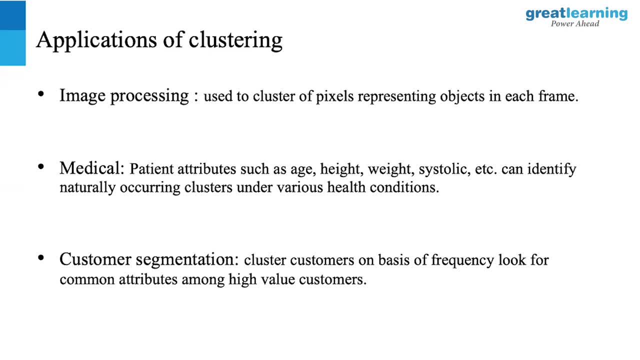 yeah, so even in that case, there is some kind of a pattern available to me. now my question is like: if, if you have trained it, say, to identify a particular person, so when you go into a production system then there will be, uh, new images to it, correct? how? how it will differentiate that? okay, so 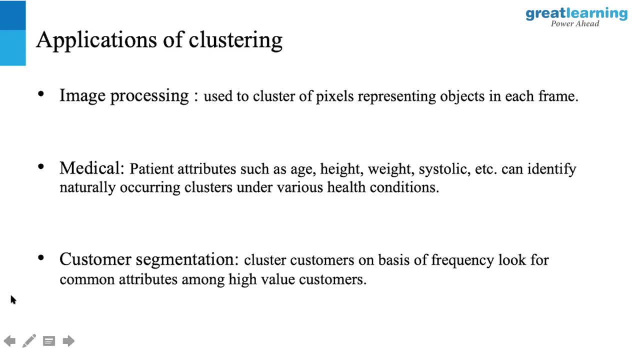 it essentially differentiates. so, uh, when slightly getting into technical aspects of image processing, right? so you, you're going to note this fact that when i talk about an image, i'm essentially, uh, going to talk about this aspect. so i'm going to talk about this: is an image, correct? 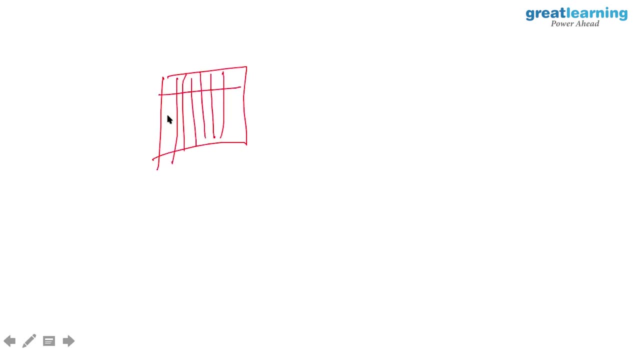 now, this image is nothing but a congregation of pixels. right now, each pixel is basically a shading. now, if i write the digit 9 in this pixel, if i write the digit 9 here, all right, let me write this multiple times. now, if you notice there are certain pixels that are shaded, well, all right for. 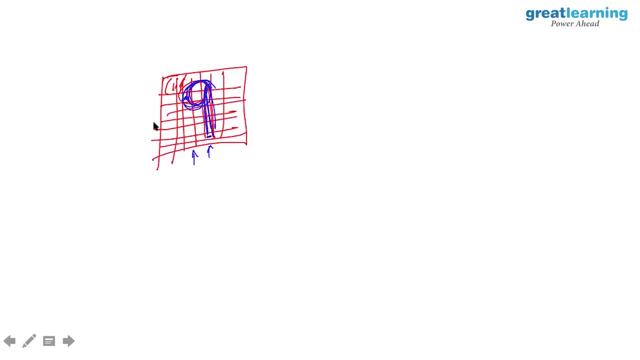 example, this pixel is shaded. well, this is not so shaded that much. so you will see this. there are pixel cells with certain intensities, so image recognition essentially is is: how much is this image intensified, how much is the color intensified? so that's basically another category of problem. 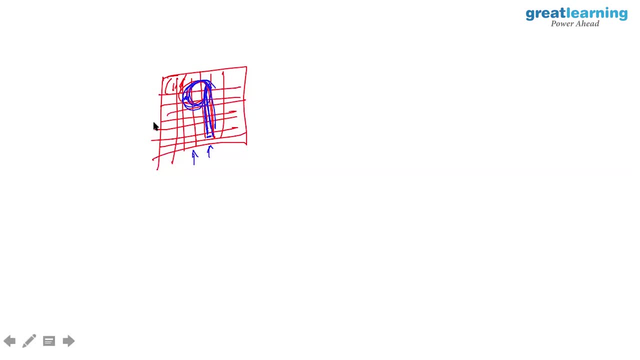 all right. so if you want to talk about production, identifying this. so basically this is my input. so my data set would look like for row 1: all right, i'll have some x number of inputs, so pixel 1, pixel 0, pixel 1, pixel 2, all the way up to pixel n, i'll have the responding shadings. 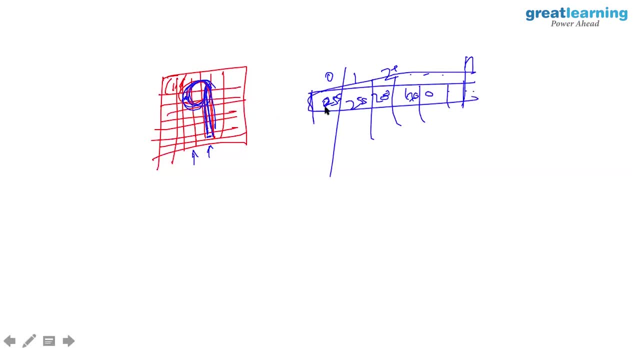 and this is. i will try to see which cluster does this belong to? does belong to a specific cluster is pattern that the digits are holding? Is there a specific pattern in the given input? So that's essentially what we call as unsupervised learning for an image recognition. 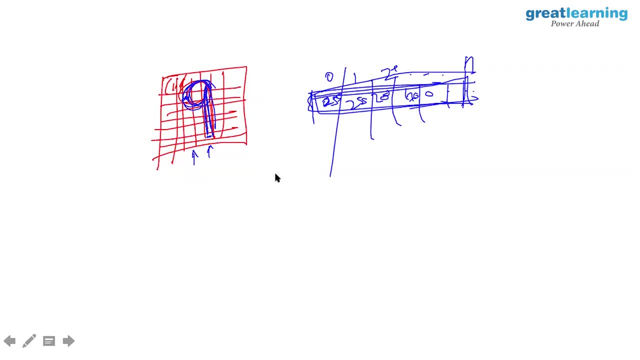 So just to extend it, now you have a 9. I have trained it on 9. So it will try to find out the patterns where it is 9 or it looks like it. I am saying that if it is not 9,. 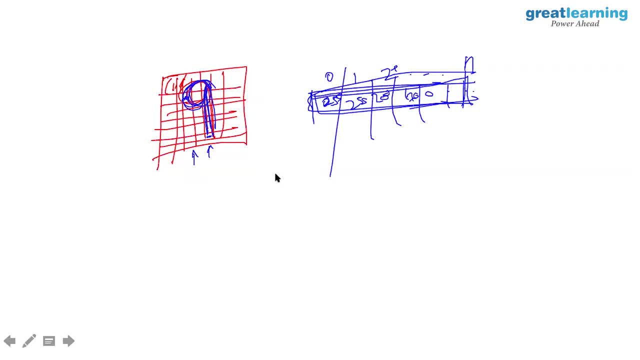 so how will it understand if I don't give it 0,, 1,, 2,, 3, anything as an input in the model? What it will identify is if it is unsupervised. what it will identify is that I have a set. 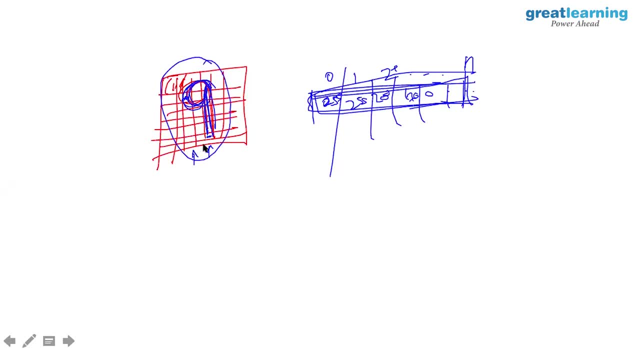 of shading along these pixel lines. Now let's look at this closely. I have a set of pixel shadings that respond to these lines or these boxes. It will try to pick this pattern and give me a separate value. What the unsupervised can tell me is not if it is a 9 or a 10, what it will tell me. 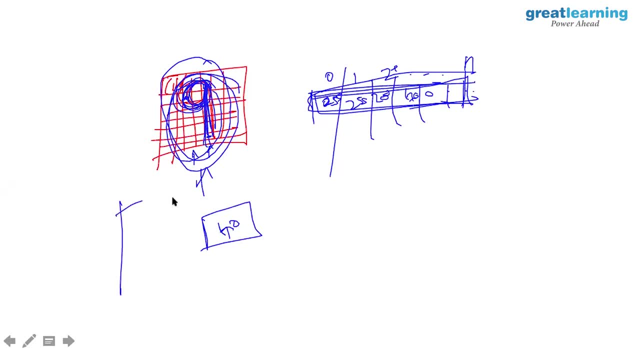 is that there is a pattern that has this shape. There is a pattern that has this specific shape. There is a pattern that has this shape. So what the unsupervised is going to tell me is identifying these patterns from the data and telling me there is a pattern that. 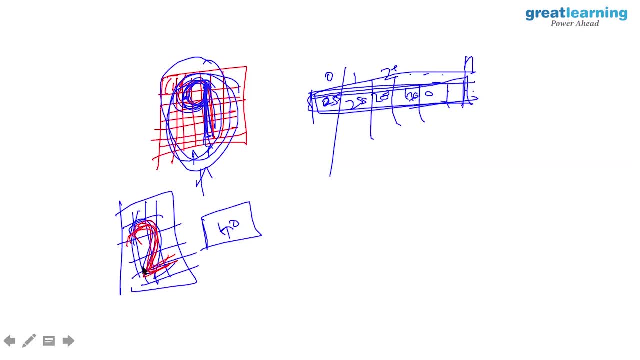 exists. There are so many patterns that exist. If you want to talk about clustering, there are so many patterns that exist in this cluster. So that's what it will identify. I'm going to throw a. So that's what, essentially, the k-means will tell you. does that make sense? 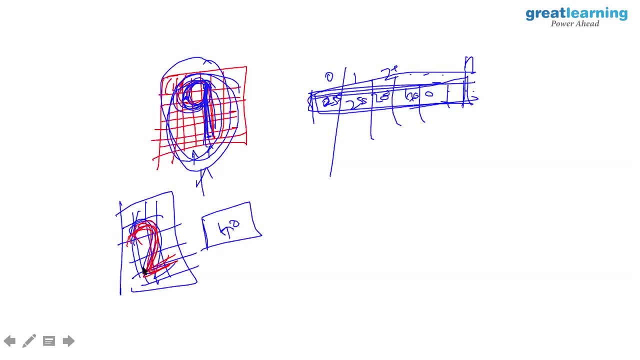 So when I have trained a model and I have given it multiple nines to it so it will identify across those patterns that, okay, it matches one of these and it goes nine, but I have not told him what two is. So what happens is it will try to put two to the nearest. so if I don't have two in, 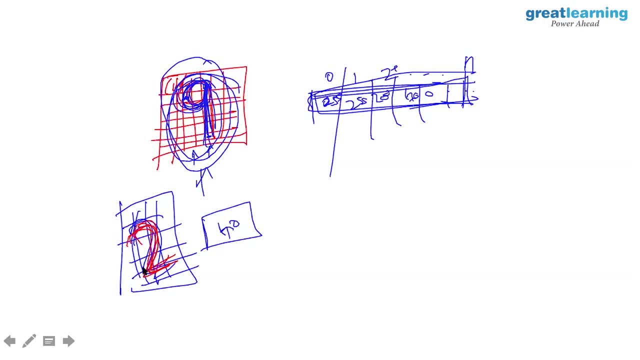 my cluster. if I don't have two as a centroid, it will try to put two to the closest object it can find. K-means will essentially work on a centroid algorithm approach, So it will try to put two to the closest objects it can find. the closest centroid, the value. 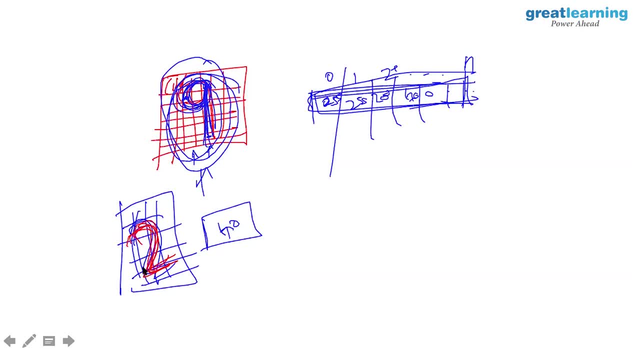 of it corresponding to a closest centroid that it can find. There will be misclassifications in the context. So when you're training it, your unsupervised is going to pick patterns. it's going to pick that nine has these patterns that they have a centroid of the value corresponding to. so 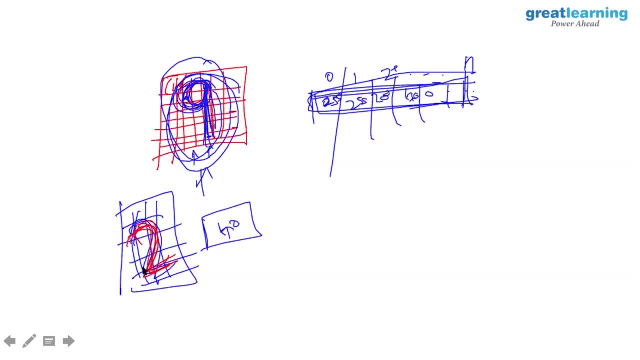 on, So pick that, Pick some shadings. two has a centroid that is corresponding to, so on, so pick the shadings. So the nine and two are something that me and you define for the machine. it's just a pattern. 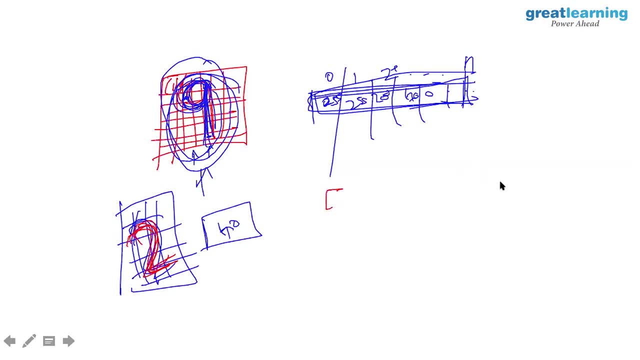 It's a pattern of shading. Okay, Yeah, So let's say this is my input, right? So if you understand K-means, it will tell you that dimension one- D2, variable two, variable three, all this So you'll have a respective shading, correct. 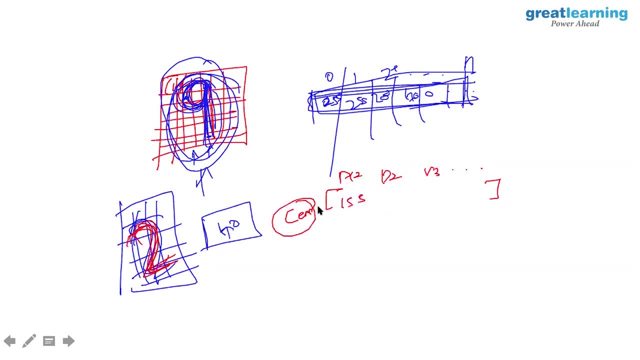 So you'll have a centroid, correct? That's how the K-means works. Yes, With me. So the K-means will have a center. So objects that are closest to the center are back to the centroid. So you will have some, if we talk about a two dimension, right? 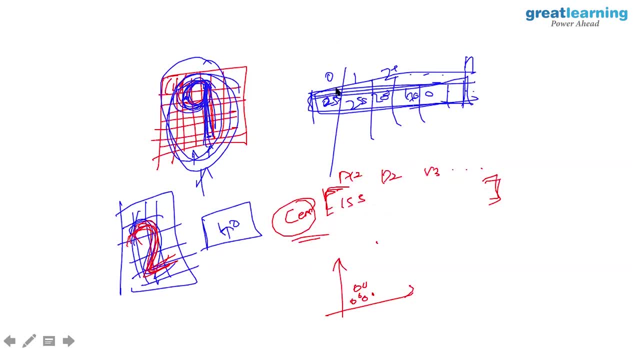 I have these points and I'll have another set of points here. Correct? Yes, So a centroid will be here. a centroid will be here. Another centroid will be here. Yes, Right Now. what does a centroid essentially comprise of? 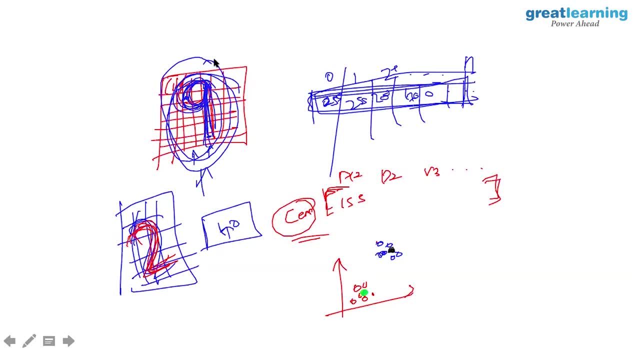 The centroid is nothing but in these two dimensions, for these two dimensions, So centroid one will be for these, for this dimension, for this dimension of one and two. what is the average value of X1, X2? that it corresponds to say a hundred or 200.. 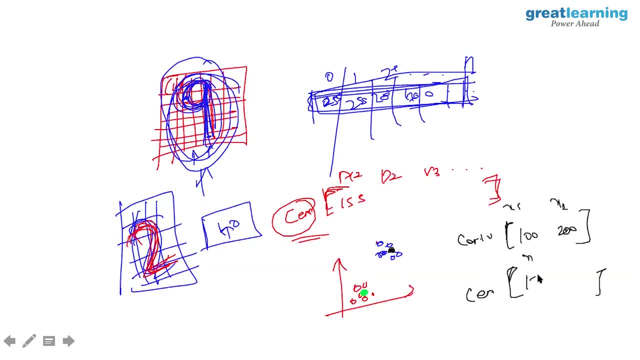 Okay, Centroid two again will represent X1, X2 with, say, 150 or 20 and 10.. Okay, Okay, Okay, So I can identify this pattern has a centroid right. Similarly, this entire problem is broken down into an end dimension. 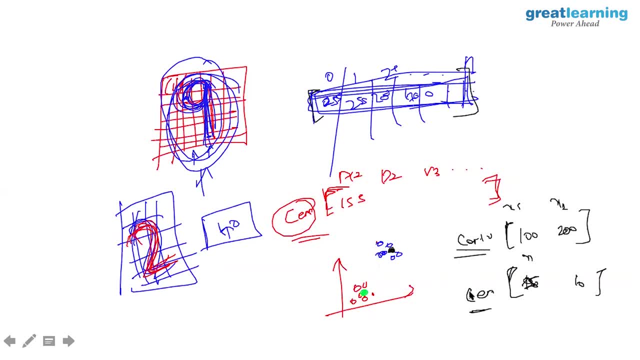 I'll have end dimension. The centroids of nine will be different. The centroid of two will be different. centroid of three will be different based on the input patterns that it sees. So it will try to identify the pattern of input that it essentially sees. 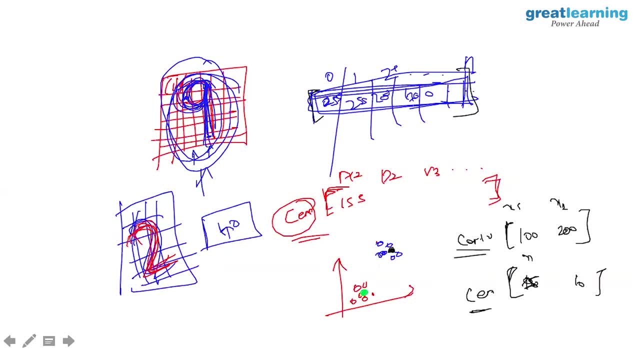 That's how the algorithm functions. Yes, I understand that. So your question is: what if it doesn't? what if it doesn't? My question might be some I might be wrong in something, But I don't know. My question is slightly different. 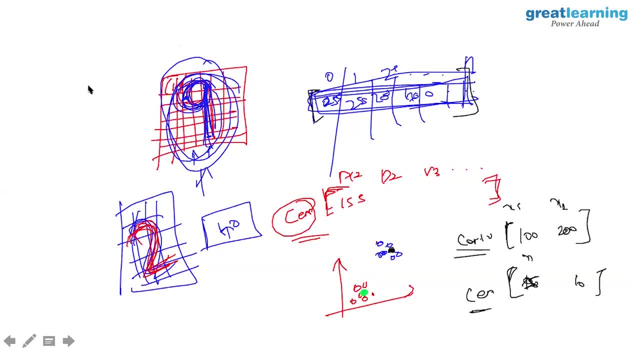 See, I understood that nine. it has a pattern. We are identifying that nine as a pattern. My question is: when an unknown comes to it. Okay, So something. let's say I have a three coming in, Yes, So now what it does is: how does it categorize it as an unknown? 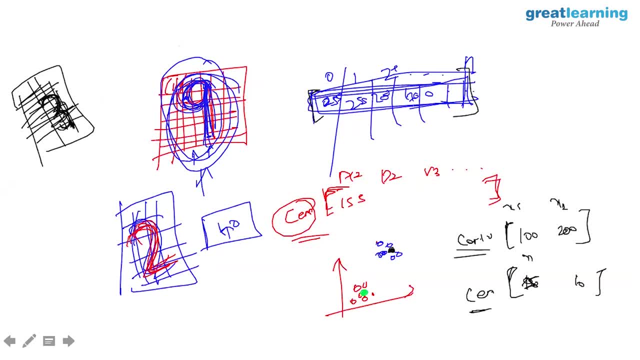 It puts three for the unknown. it completely does not see right. It tries to put this three to the closest centroid it can find. So the input value to the closest value it can find. it will place this object to the closest centroid it can find. 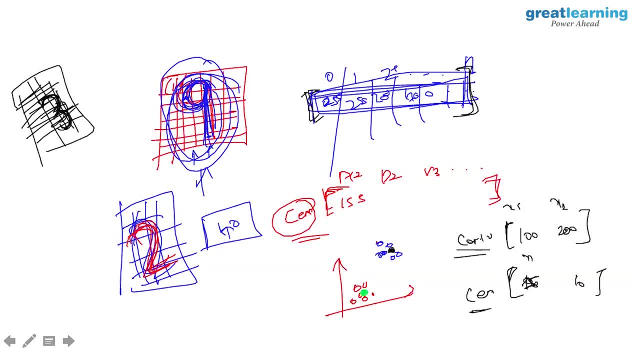 That is how it works. So how does it takes into account that- okay, this is. these patterns are not available in my data and that this is a new pattern which has to be categorized For unsupervised learning? there is no specific pattern. 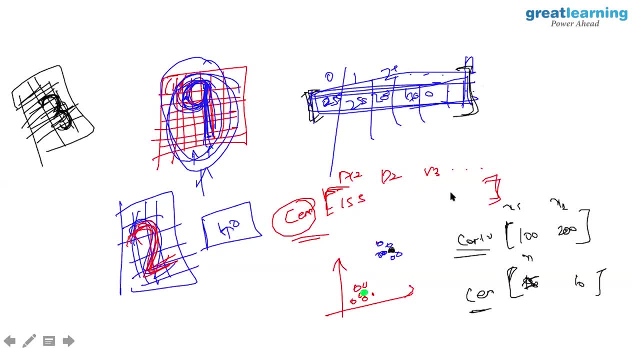 So it just has a value. It has a centroid. So you will, when you train it right, When you train and K-means algorithm, So you're going to create these centroid, Okay, So you're going to create these center values. 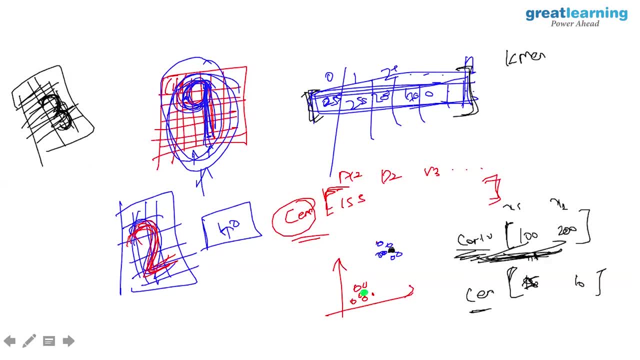 Correct With me. Yes, Right, So K-means when you train it, it's going to create the center values. Yes, From the center values that it creates. Okay, Any new point that objectively comes in is going to have some input. 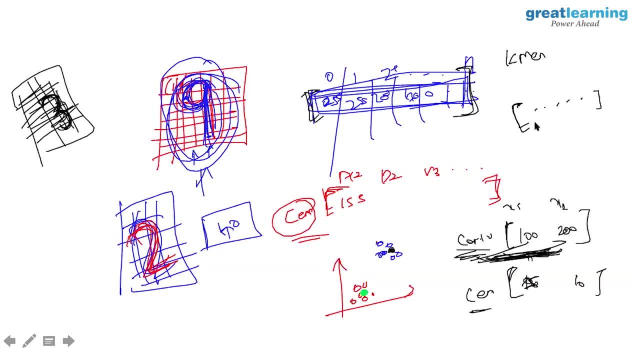 Yes, It is going to compare the distance between this point to the center and to the center and to one more center And tag it upon And tag it appropriately To the center that has the lowest distance. Does that answer your question So? 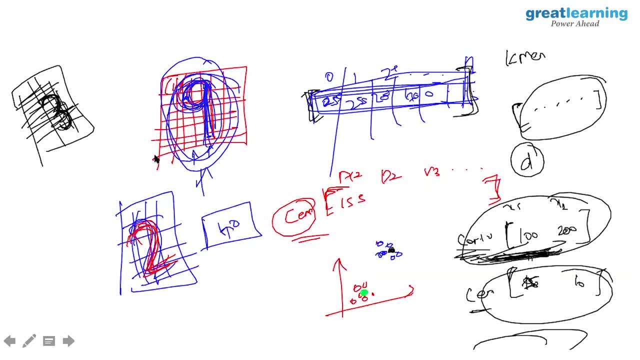 We train label here. There is no pre-training that says this pattern is belonging to group three. That becomes a supervised learning. So what K-means will identify is a new point. For example, this image three. or let's take an image four, for example, right. 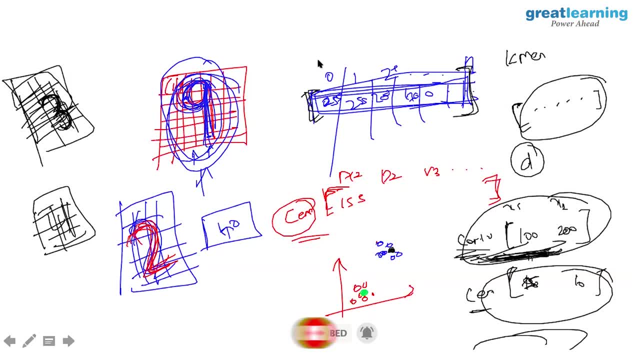 It's going to have some pixel shaded, So it is going to have a data input that looks like this: Correct, You understand this input, The input I am tagging here. Does this input make sense in terms of pixel shading? Can you tell me something about unstructured data? 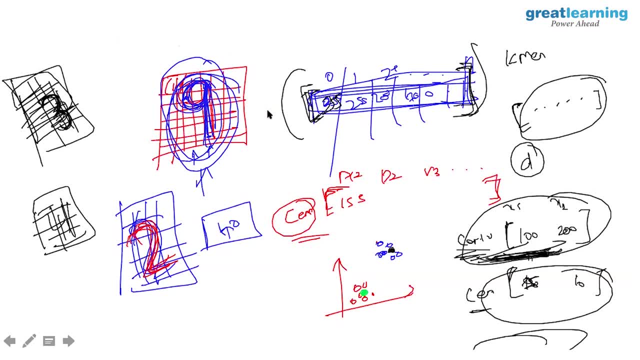 In ML terms what it means. It doesn't follow a pattern or something like that. Not precisely. So when you say unstructured data, text is an unstructured data. When we say text is unstructured, So I can say this is an input. 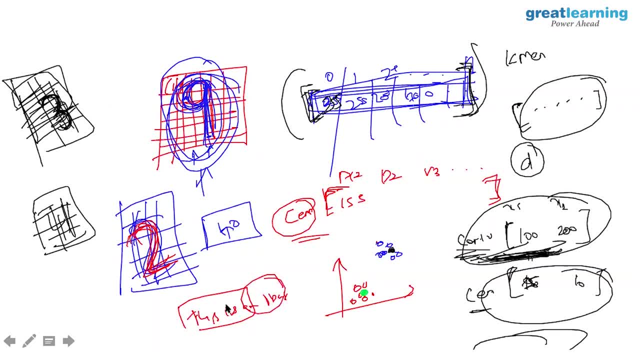 Right. So the machine has to understand that this is an unstructured, because if I give a direct text to a machine, it cannot understand anything. any input as part of it, There is no information it can correspond it to. So this has to be converted from a text form to a machine readable numeric or a number. 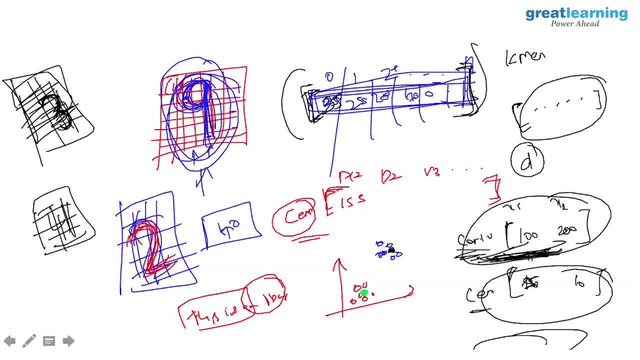 based form, That is what we call as an unstructured. So image is another example. So image directly. The machine cannot recognize an image without understanding what contents it has. And even if it understands the contents, how will it understand these contents? 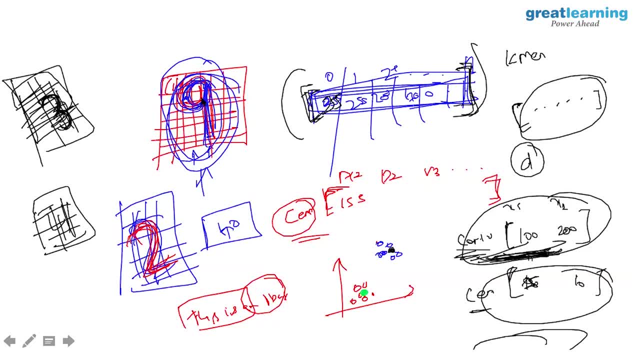 The same problem that me and Nitin were discussing. So if I have a number 9 here, how will it recognize this number 9 as number 9? Right? So the question, the way it essentially does, is it has to break this number 9 down in terms. 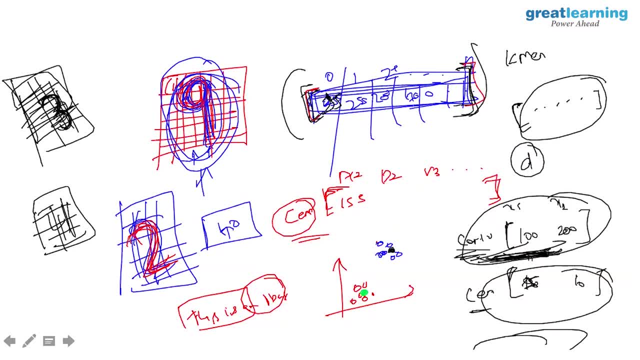 of a pixel shading And from these pixel shader values it will. It will train and learn that if these pixels are highlighted, then this corresponds to the probability of number. 9 is so, and so It's a number. It will rank the probabilities from 0 to 10,, 0 to 9 and find out which is the highest probability. 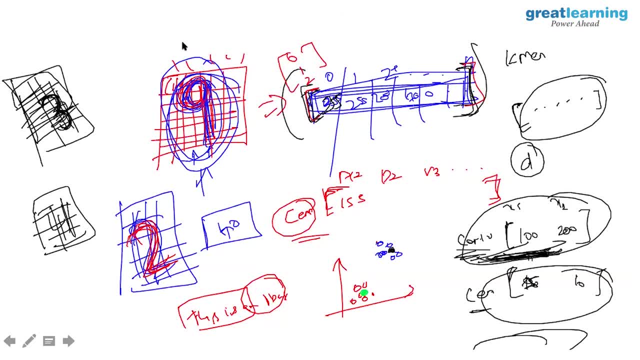 closer to this. So I think what- maybe, Nitin, you can correct me if I'm wrong, but I think what Nitin is trying to ask is that since in the unsupervised learning we do not have target labels, so that means that when I'm 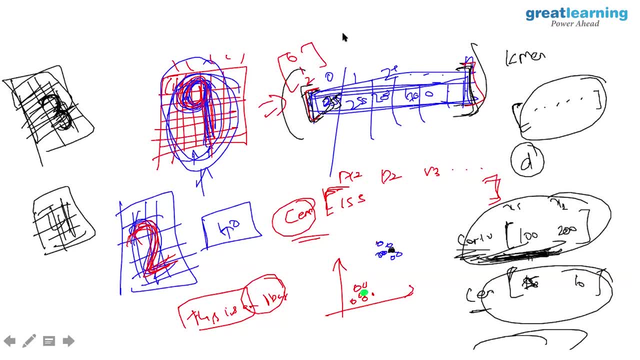 When I have training in the target, When I have training in the training data, you do not know that. what are the exact number of labels would be? For example, if you're talking about the digits, then we do not know that. If I'm going to have 0 to 9 or much more than that, 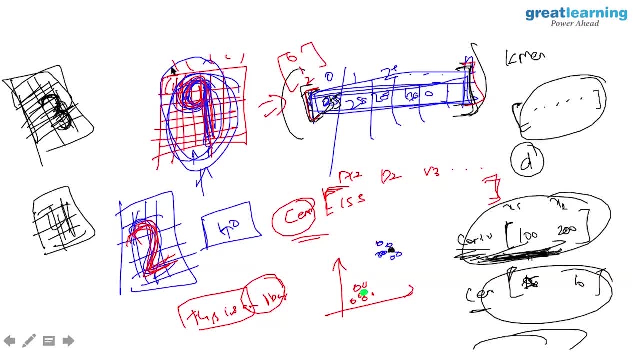 Or just 0 to 8 or 0 to 7, something like that. So since label data, it is quite possible that your training set do not have a pattern line at all. And now you actually deploy that model into production and you get an image which is actually 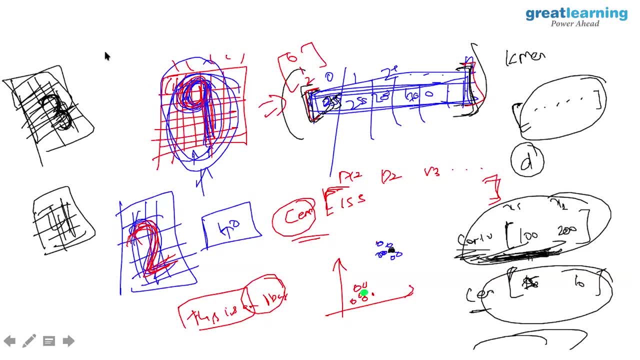 representing 9 in that case, Right. So if it is representing and if the actual deployment has a number 9 as a representation, right When we train the data. So if you get a number, let's say I'm training on number 9, I'm training between 0, 1, 4. 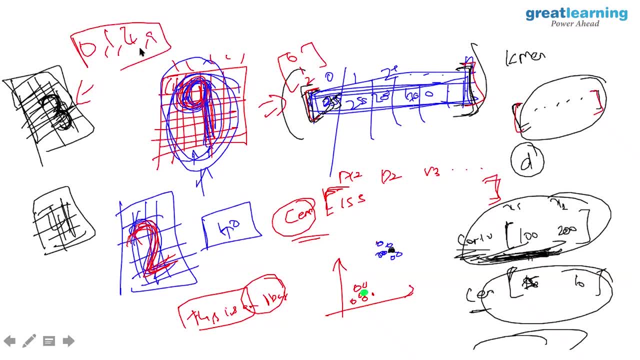 and 9.. Right, And let's say I'm training on this and I get a number 3.. All right, So the shading or the pattern that number 3 exhibited will be different, will be completely different to any of this that I've seen earlier. 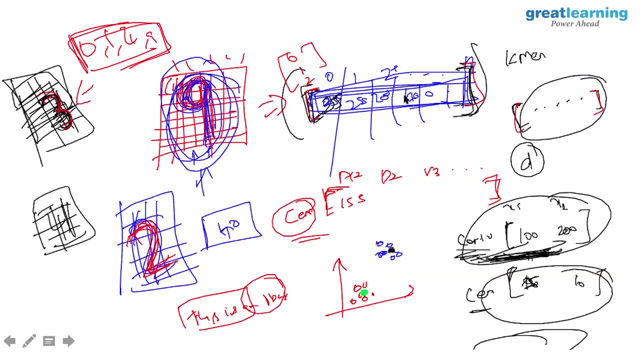 Correct Right. So what K-means ideally does is when I'm training it, if I say there are four patterns in it or there are more than four patterns in it- there are more than five patterns in it- it will create appropriate number of centroids. 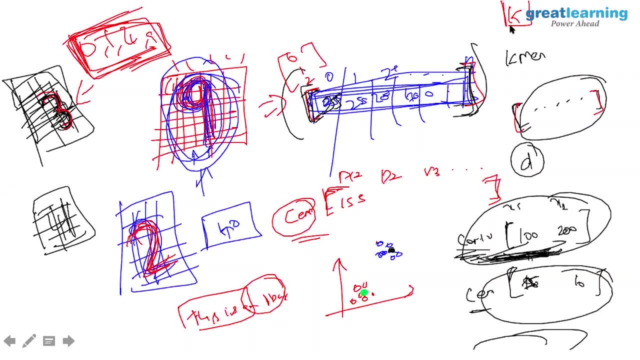 Right. So that is what we call as a K. K is the number of centers I'm defining in my data. Either I choose the inertia to choose ideal centers. I either choose it based on the elbow method or I just randomly choose an arbitrary number. 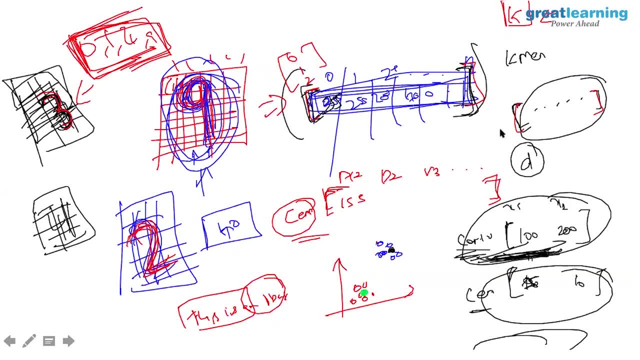 of K that I want and I set it up Right. So when I define that my model is going to be in my data, my structure is going to have some K number of centroids, Right, Right. So in my production if a number 3 comes in, so the number 3 is going to correspond to. 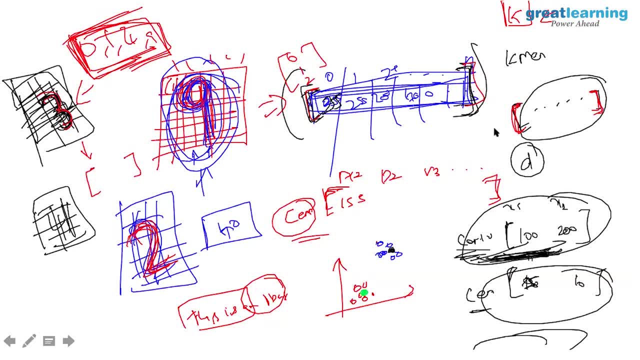 an array of values. So this array, the distance that this array has With all the centers Right, And it will be misqualified depending on Yes. So it will be misclassified, Definitely there will be a misclassification. So that's the problem with unsupervised learning. 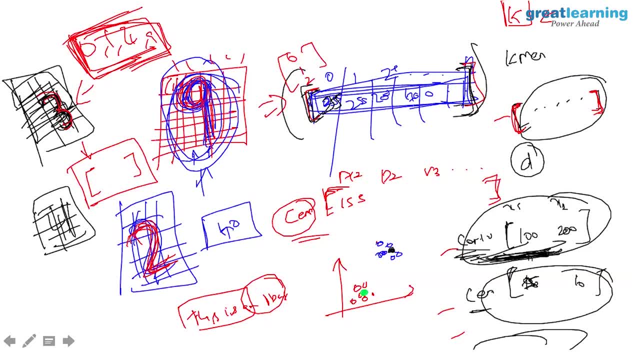 I don't have a specific target to measure it against. There is no measurement index to say this is accurate, this is inaccurate, So it is basically a pattern. So I was just asking that because it means that it has to be kind of a continuous feedback. 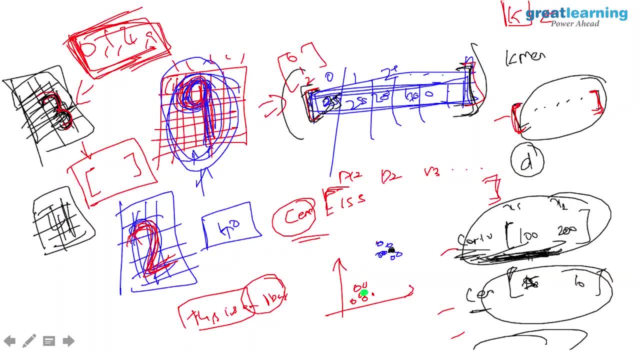 kind of thing where you Right, Qualified few things, then you actually bring this new set of data to your training data. Yes, So this is what we just talked right now. So what you just spoke about right now, Rohit is what we call as the neural network models. 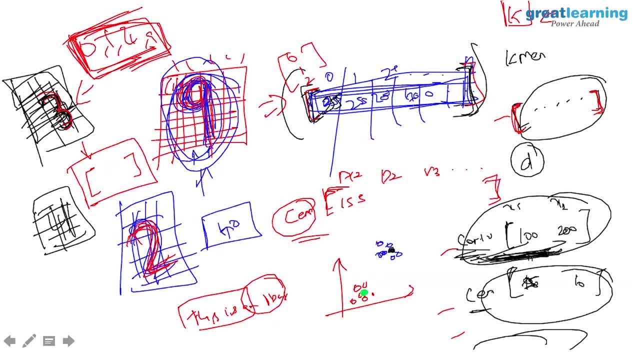 or a structured neural network or a recurrent neural networks or things like, where there is a feedback loop. Okay, So we call that as a reinforcement learning, where there is a feedback that goes from the input output back to the input in terms of how classification accuracy has been created. 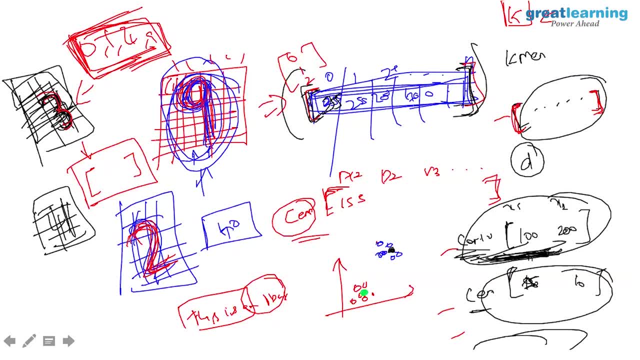 or not? Okay, That sort of feedback becomes a deeper neural network architecture. We call it as a reinforcement learning model. Okay, So, Chitra, one point to add on your note. right, So you say you mentioned that the number is a structured form of the image. 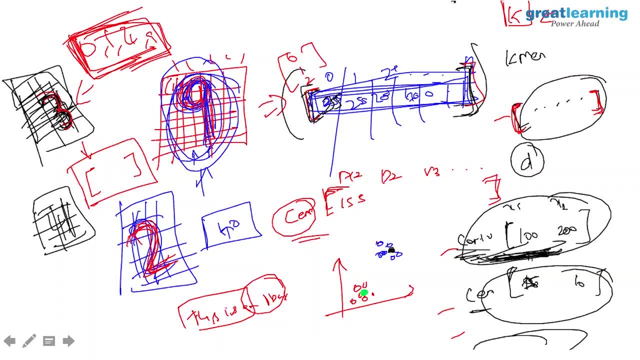 So I beg to slightly differ in that point, Chitra. The reason I say that is the number is so I as a user, I as a human or you as a human or a user, can understand anybody writing nine in different ways. I might write it nine with a broken nine. 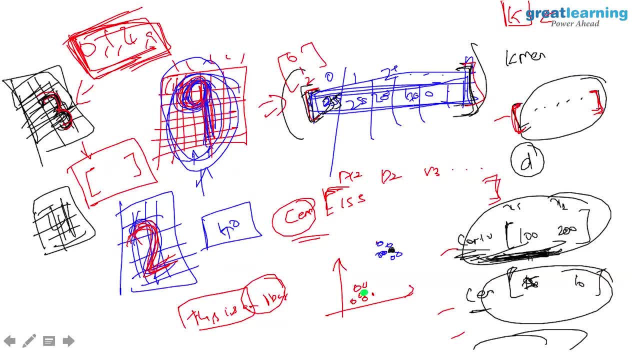 I might connect them as loop. I might not connect the loop right. So what happens there is, you can read it. You can read the image. You can understand this image. Now to the machine. it's nothing but a mere input of patterns of the respective cells. 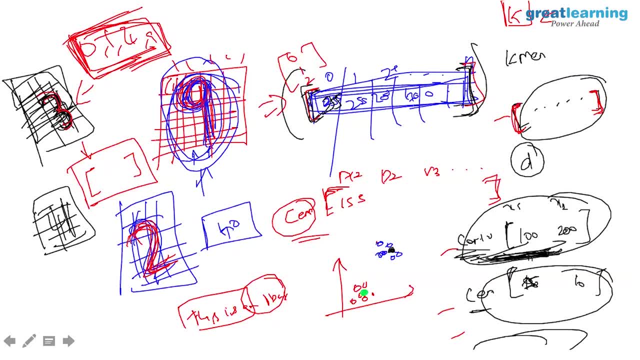 of pixels being shaded And that pattern per se is what is being understood By the machine to say okay. the probability, if I see this pattern, is 70% towards nine, 10% towards a one and 10% towards eight. 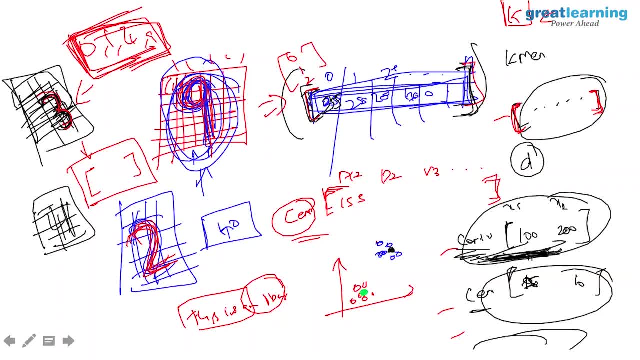 Reminding, this person is just split across the other numbers, So that is what the pattern is essentially corresponding to. So that is still an unstructured problem that we are going to define. So the data is unstructured, which means that I cannot natively use an image to an input. 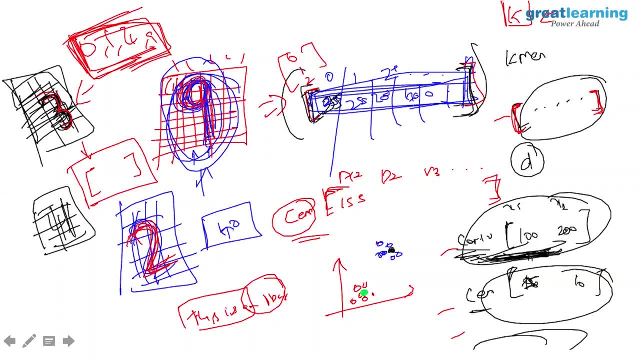 and say, okay, learn from this and and the machine can work from it. So there is. there has to be a set of inputs, There has to be a set of input steps that converts this image into a reference value, And then that reference value has to be learned by the model to make an actual prediction. 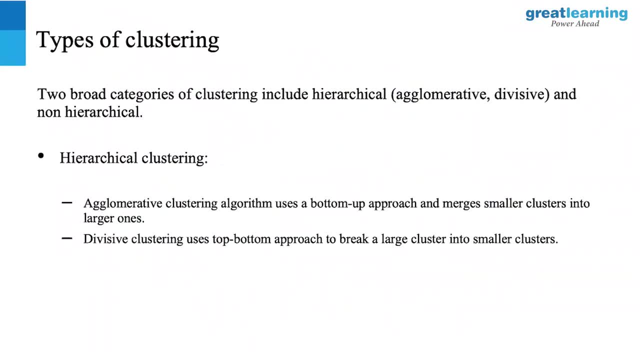 Right. Does it make sense? Does it answer your question? There are two types of clustering per se that we essentially look at. One we call as the hierarchy clustering and the other we call as a K-means clustering. So hierarchy clustering is an agglomerate. 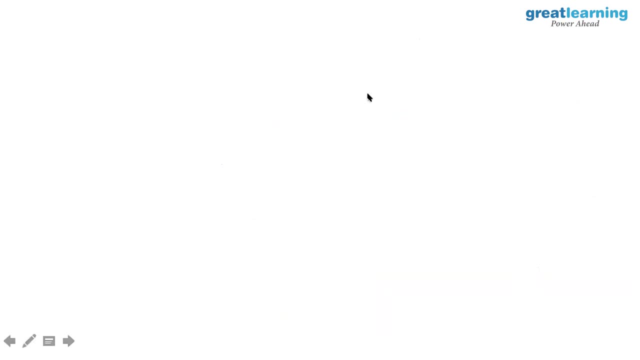 Basically it's nothing, but it's an aggregate based clustering. So if I want to talk about hierarchy very quickly, it's part of your discussion next week. So hierarchy clustering basically starts with every data point as a cluster and then slowly aggregates up back into a single cluster value. 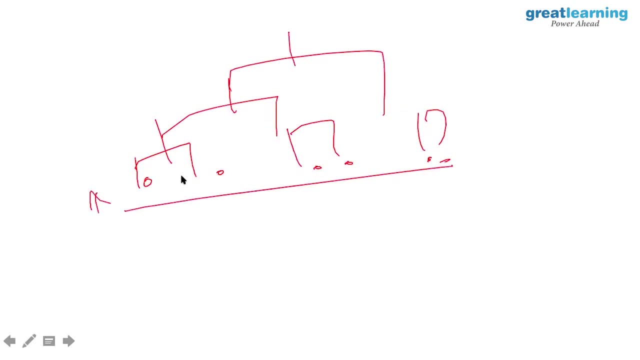 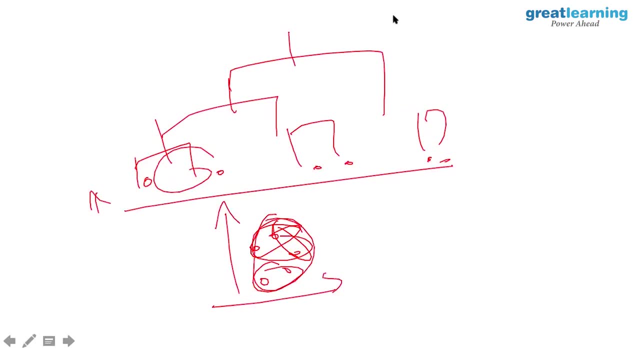 and then the entire thing. So the hierarchy clustering is that kind of an approach. K-means is a little more different. K-means is an iterative algorithm where it starts with random centroids. K-means will start randomly assigning some centroids across the data point. 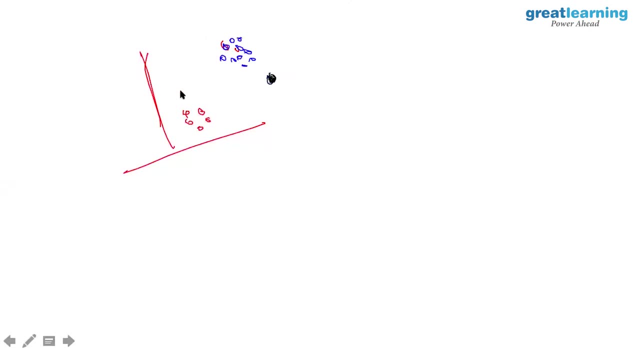 So it has a random start to the entire algorithm approach And iteratively it will try and converge. It will iteratively try and converge from this to the center, Again from this point to the center. So it will try to converge and center. 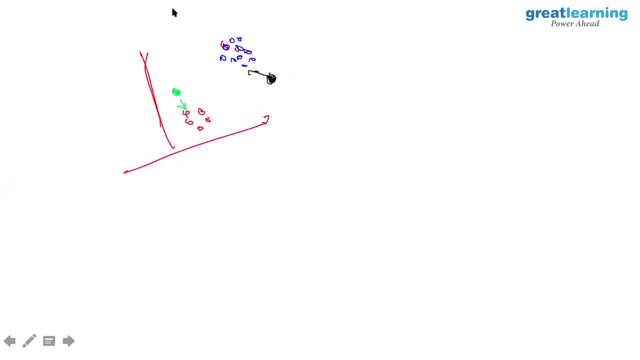 Which is the closest to the actual value. So the K-means is an iterative algorithm which basically converges on an iteration, So it will first start from a random start point and then try to initialize and then check the cluster that it is closer to. 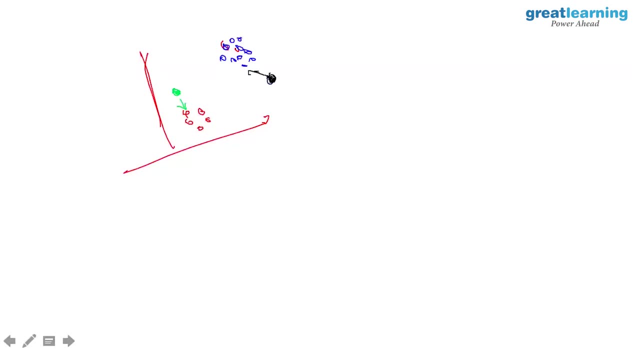 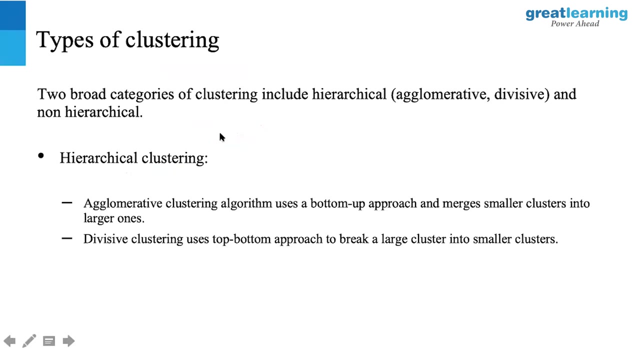 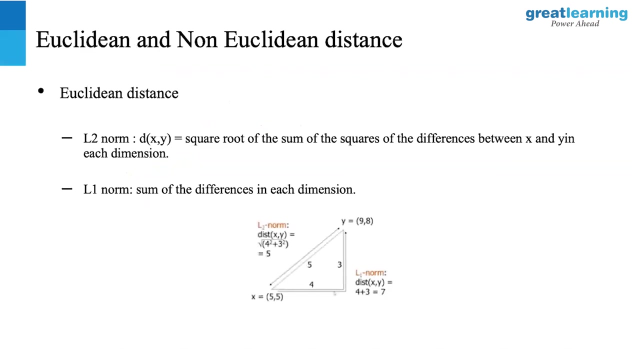 Check the distance of the cluster and then converge more closer to that cluster. So that is how it effectively works. This is your K-means approach as a hierarchy clustering. Now we are going to talk about different distances being used. So one of the most common distances we are going to use is the Euclidean distance. 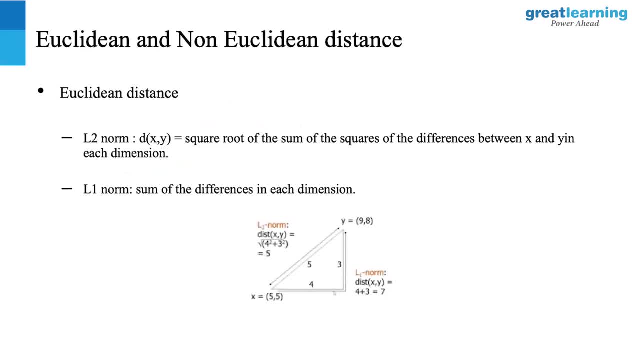 Now, Euclidean distance is the square root of the sum of the differences between x and y in each dimension. So that is basically, we are going to measure x2 minus x1 to the whole square, plus y2 minus x1 to the whole square, plus z2 minus x1 to the whole square. 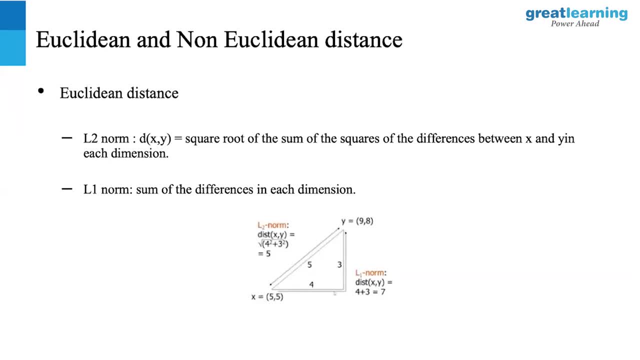 So, based on n number of dimensions, That is the L2 norm. The L1 norm is nothing but just the sum of differences: x2 minus x1, plus y2 minus y1.. So that is basically your L1 and L2 norm. 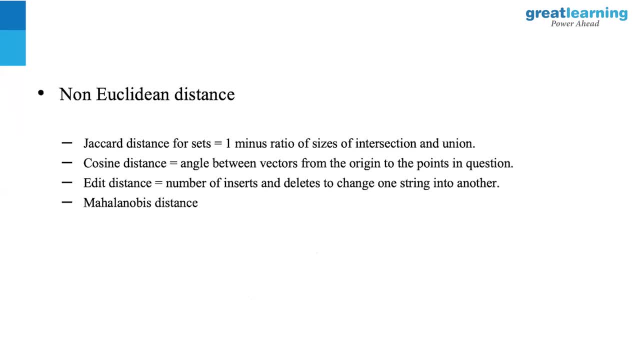 Euclidean distance. So jaccardian distance is used to find out objects in similarity. So we use the jaccard distance. It is 1 minus ratio of sizes, of intersection and union. So basically you want a ratio of intersection So the number of objects that are closer to that are matching it. 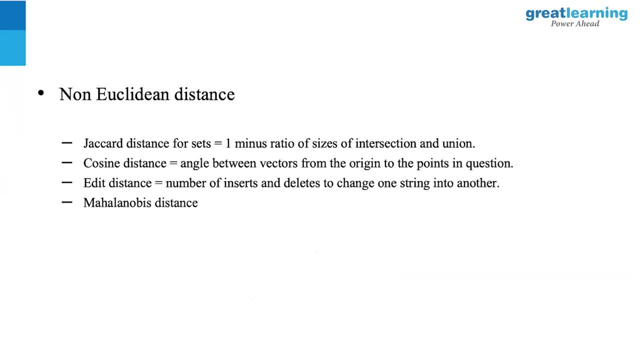 Divided by the union. So number of objects are the complete entire set, So 1 minus the ratio of that size. Now jaccardian distance is used there. We are going to have talk about The vector recommendation engine. So that is another distance set that we are going to use in recommendations. 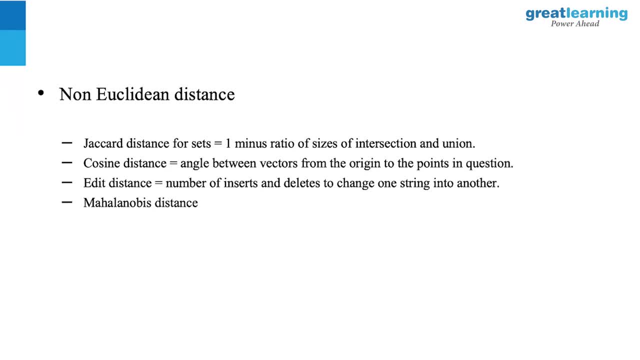 So for movie recommendations we use the jaccardian distance. Now cosine distance is another mathematical distance. It is a cos theta angle distance. So cosine distance is defined as a dot b. So it is actually a vector Magnitude of a into magnitude of b. 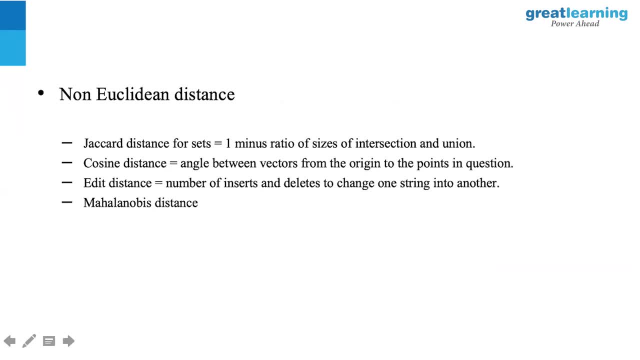 So this is what we call as a cosine distance. Okay, So cosine distance is used again in. It is another application in word similarities, Chitra. So, for example, you have this package that we call as glove or word embeddings. So if I want to find out a word that is very similar to its nearby objects, 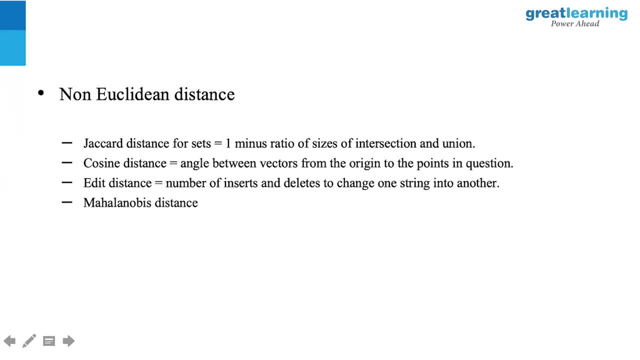 Or very similar to words that are closer to it. We use a cosine distance. So we say, okay, this word may be closer to this word based on these aspects, So based on the cosine distance, or cosine similarity is what we call it. So that is a text based similarity. 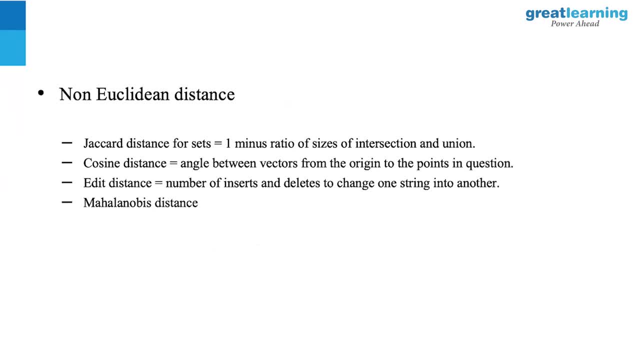 Again, most of these distances that you see, the jaccard cosine edit, Most of these are predominantly used in text corrections and text management. So we use word vectors, word vector embeddings to do these spell corrections, Edit distance. cosine distance comes in specifically there. 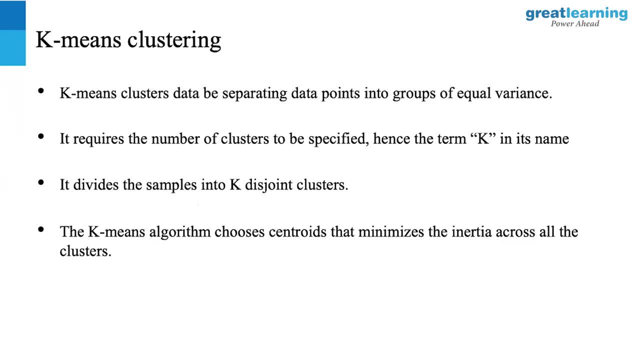 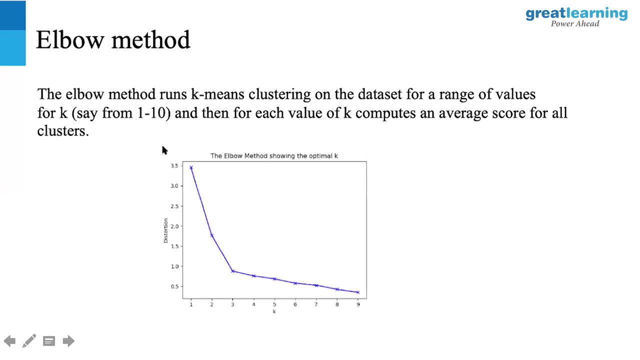 Alright, The k-means clustering is what we were just talking about. it We were going to talk about k is the number of centroid that we choose. Now, ideally, the number of centroid is to be chosen by what we call as an inertia. So inertia is nothing, but let me just explain this concept of inertia here. 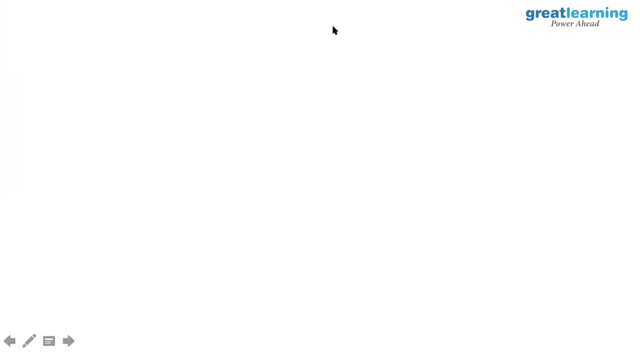 Okay. So let me just try and explain the concept here. I will see if you can make as much of sense. Let us say this is my point. Okay, Now, this is my data clusters. Let me draw this here first. Now let us say I am going to draw the elbow method here. 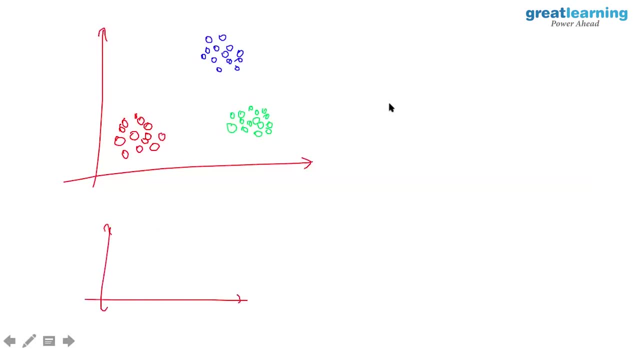 Alright, Now. the elbow method uses what we call as inertia, Or, in other terms, we call this as sum of squared distances. Okay Now, this is nothing but a very simple fact, that okay. Now to this data, to this set of input. what do you think is the ideal number of cluster size? 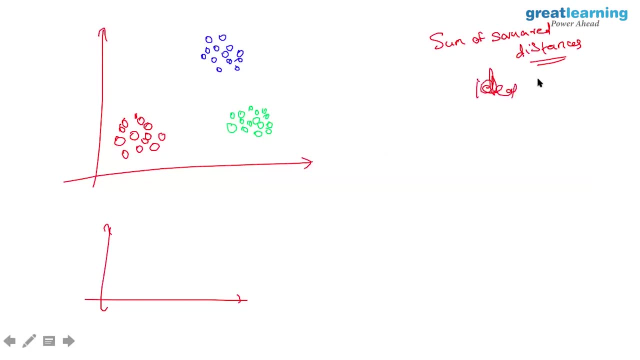 So ideal k is 3, because this is only a simple two dimension and I can easily see it. What if this is n dimension? So what happens to the sum of squared distances? Let us say I set only one centroid. Okay, Now let us measure the distance of this point to all the objective points in the cluster. 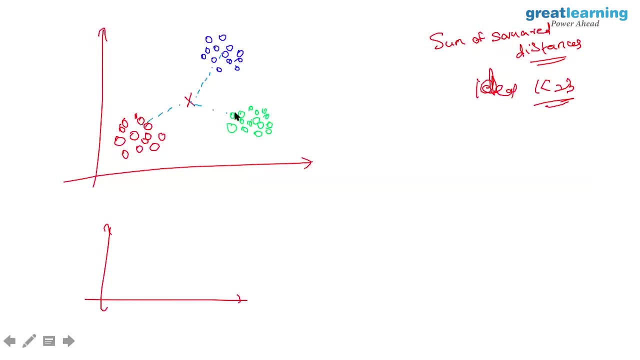 So what do you think will be the sum of distances? Just let us say, if I treat the entire data as one cluster, if I just have one centroid, what do you think will be the distance that it carries? What happens if I set the number of clusters to 2? in this context, 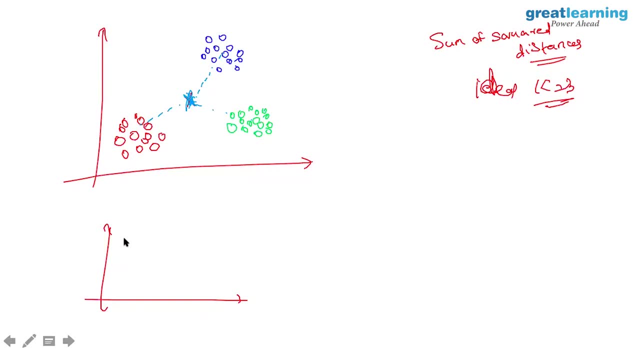 Let me say it starts with a very large value. What happens if I set the number of clusters to 2? The sum of squared distances will be 1.. Okay, What happens if I set the number of clusters to 2? The sum of squared distances for, instead of one cluster, if I set it at 2, what is going? 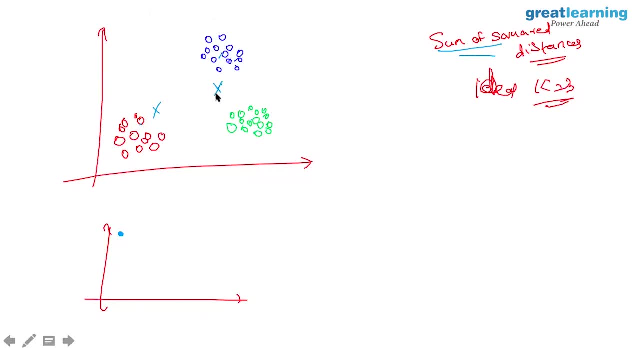 to happen to this. If I set 2, maybe this is maybe the point, This may be the point- The distance, the sum of squared distance between this object to this point and this, to this point, will it come down? Will it not come down? 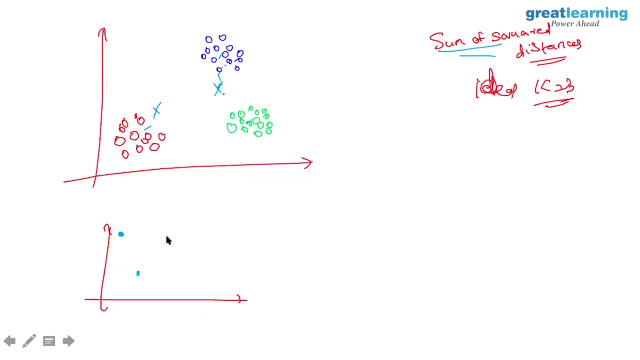 So I am going to have a reduced distance. What happens if I set it at 3? It is going to even further come down, But beyond 3, the sum of squared distance is not going to come down and it is going to start tanking. 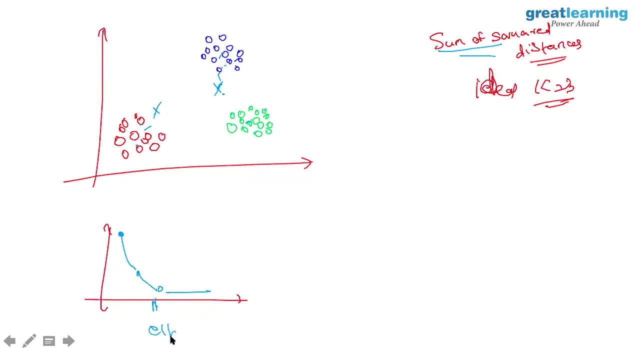 So this part is what we call as the elbow. Elbow is a point at which, where the sum of squared distances is the solution, where I find a steep change in the sum of squared distances value. Does that make sense? That is what we call as inertia. 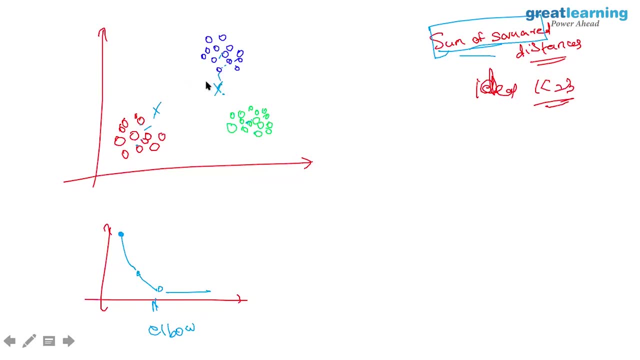 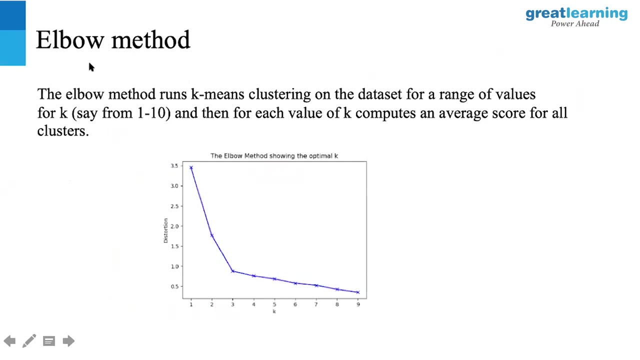 Inertia is nothing but the distance. it carries the sum of squared distances. it carries to the centroid, specific centroid. Now, this is the elbow method. I have Alright, Now I am going to go ahead and we are going to start. We are going to start implementing a quick cost string approach to a data point that. 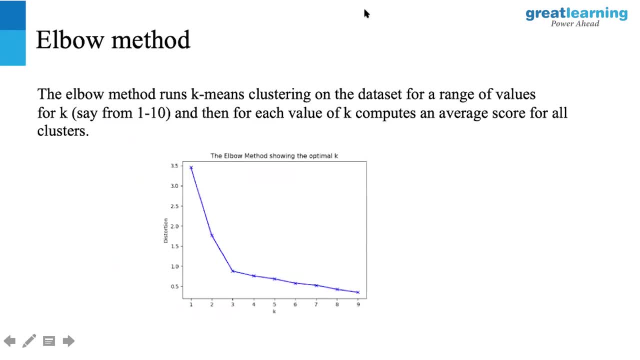 we have Alright To a data set that we have. Now this data set is going to be about. it is a psychological study. The data set- if I want to give you a prelude to the data set- it is nothing but a psychological. 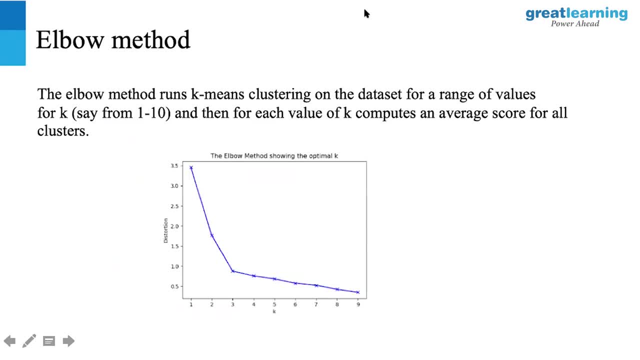 study. Okay, It is a psychological study that effectively talks about what is the fatality rate of somebody's thought process, What is the simplicity in thoughts that somebody has? Now, simplicity, here is a brain. Simplicity here is a black and white distinguishing thought. 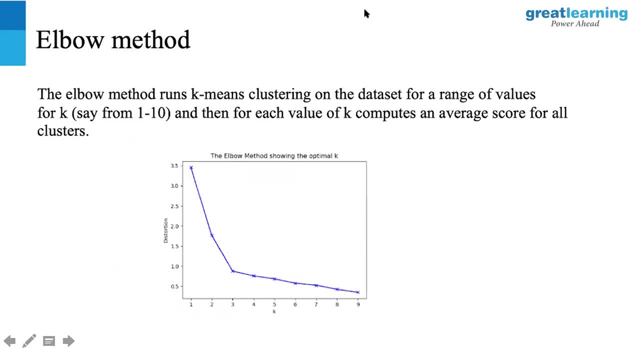 So am I looking at black as black? Am I looking at white as white? And what is the depression quantum somebody carries? So these are all three things that ideally is looked upon in a psychological study. Now we are going to analyze this data. 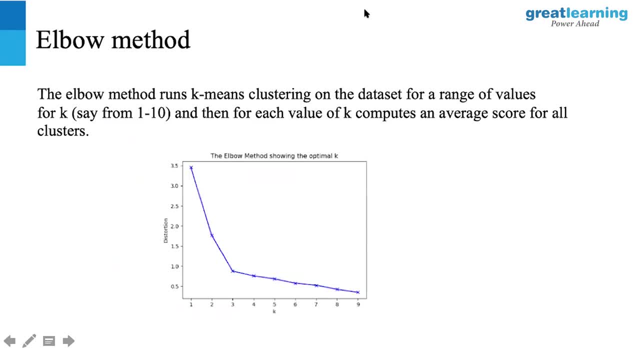 Now, if you understand this, none of this data, none of the metrics I told you right now has anything to do with the target. So I don't have a specific target to say what psychological state this person is. This is a very simple point. where it says there is no target variable. 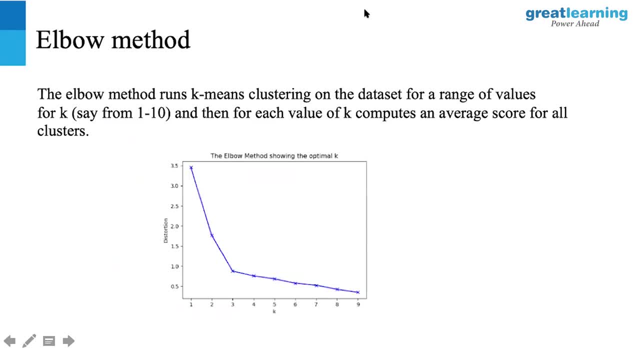 But we are going to find out what are the groups of people that I have. How many groups of people are ideal? What are the groups of people I have in my data? Okay, So that is effectively what I am going to set up on and do. 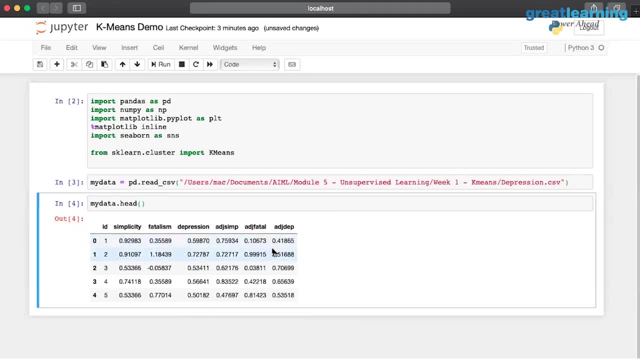 Now, if we notice, this is my data, So I am going to have this simplicity, fatalism and depression as the key inputs. This adjusted simplicity, adjusted fatalism and depression are not going to be my key inputs right now. I am not going to worry about those parameters. 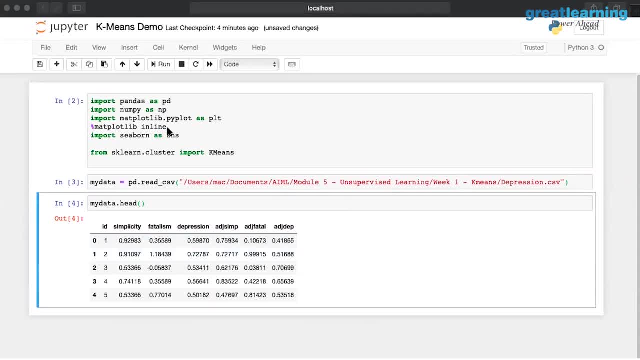 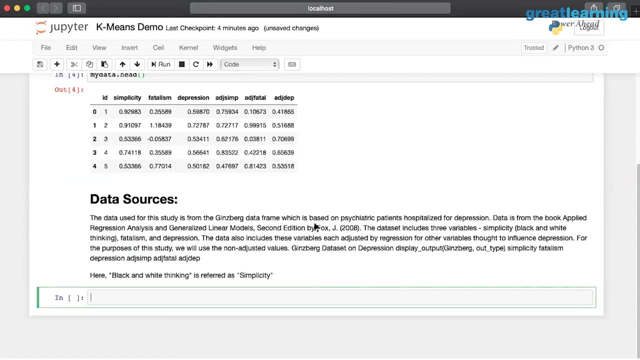 So if I am going to give you a little more context about this data, I am going to give you this piece of block that I have Now. this is the data source. So, basically, it is used for black and white thinking, where we call this our approach to. 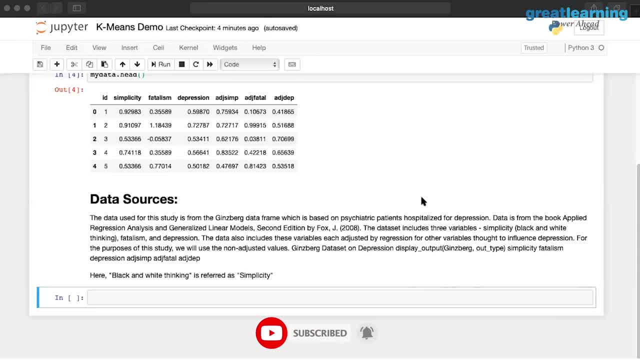 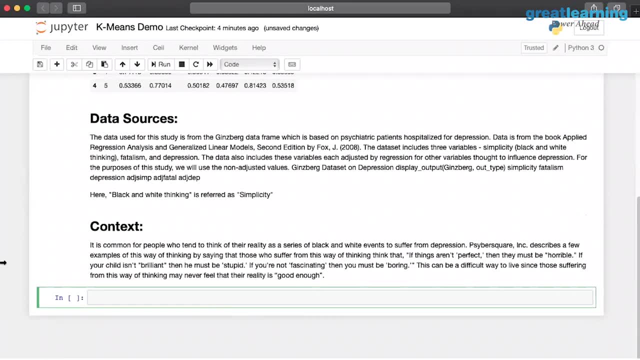 somebody's approach to simply saying how are they perceiving things right Now. this is also the quick context of the story. It is common for people to think as black and white events, to suffer from depression, cyber square, etc. This is a new way of thinking. 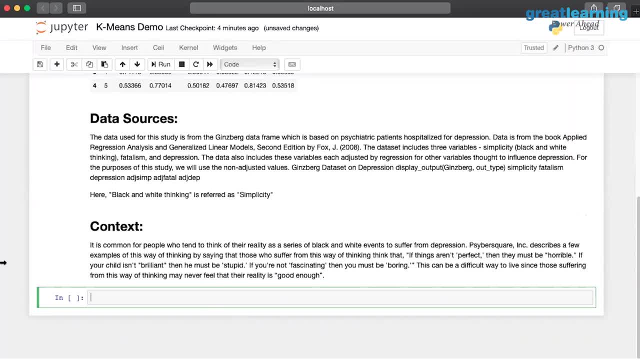 All right. So what I am going to find out is find out groups of people that are similar together so that my treatment can be as appropriate, or my approach to this, So the problem that they are facing can be appropriate, or different ways of essentially handling these people. 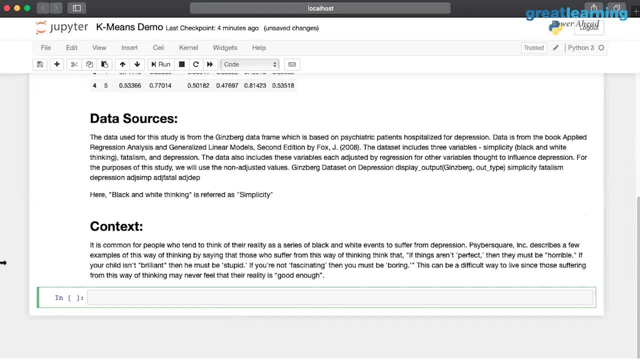 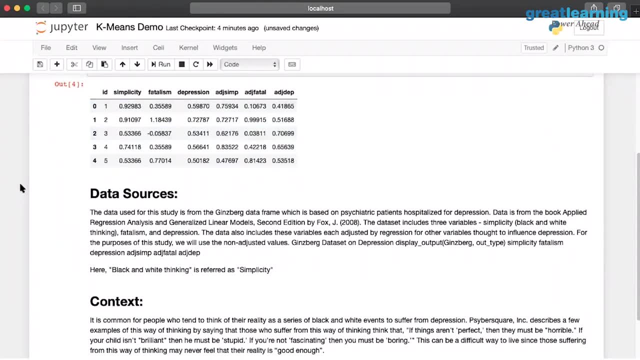 So that is what we essentially look for in this model. So I want to find out from my data about how can I use this simplicity, fatalism and depression parameters to look at these people and say, okay, can I look at this, Can I solve this person's problem? 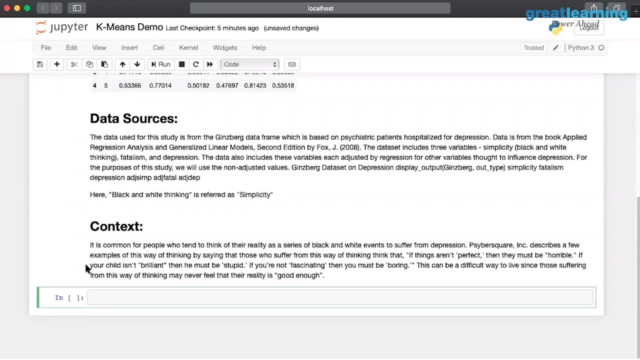 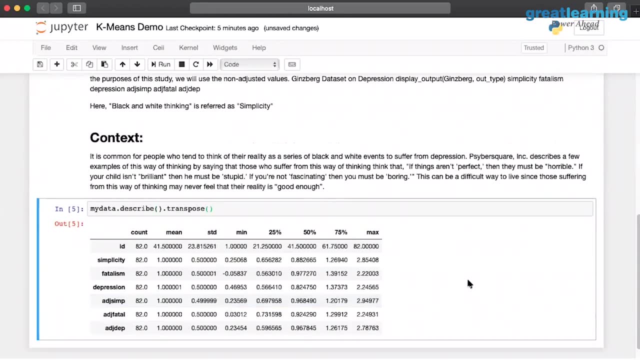 Can I solve this person's problem that they have? Okay, Can I first identify who these group of people are and then make my relevant inputs as appropriate? Now, one thing I want to quickly draw your attention is information. If you notice, there is something very different about this. 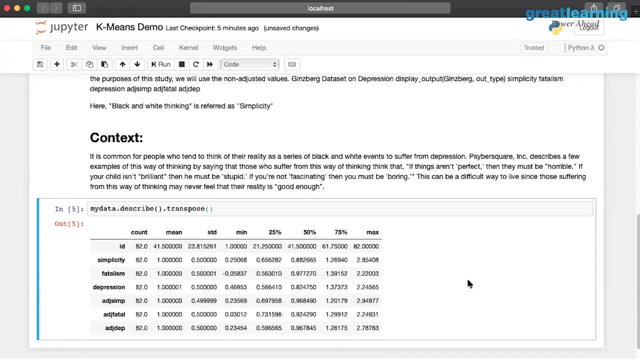 So your mean and standard deviation, for simplicity, fatalism and depression are exactly equal, right, So that's another quick question. Okay, So the next point I want to add to key means. if your data has a different mean to each of its column and the standard deviation is different to all the columns, then we must: 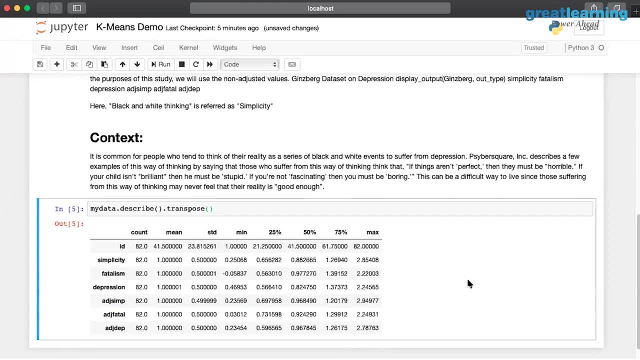 normalize or standardize the data before we proceed towards the model building aspect. All right, Okay, Now my columns, my parameters in my data. Just one thing: When we call, when we say it's different standard deviation, so what is the deviation? 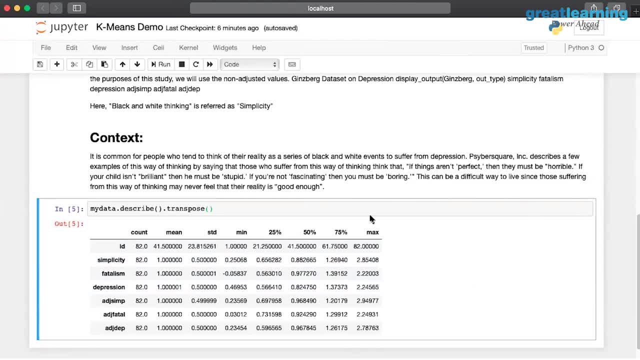 that is considered Okay. So the deviation can be any value. Nathan, just to quickly put the same answer to both questions, Both of you are raising the same question. The standard deviation or the mean can be any value, but the mean of all my columns. 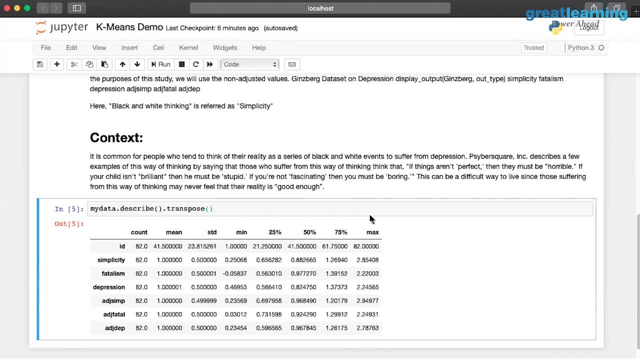 must be an exact, more or less an equal value, or- and my standard deviation of the columns- must be an equal value. It can be 0.5.. It can be 2.5.. It can be 10. It can be any value, but it must be a constant value. that is precisely the same. 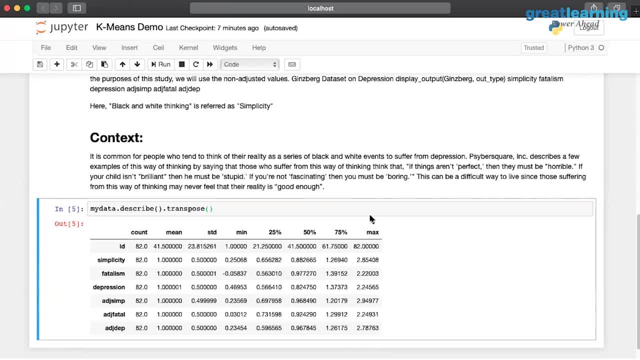 If it is not, then the data must be standardized. Now, if you notice, the standardization is a property. If I talk about the standard normal derivative z, it is nothing but x minus mu by sigma, which will convert my data to have this property of mean equal to 0 and standard deviation. 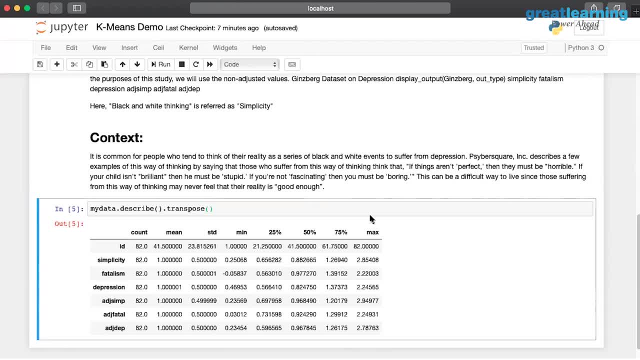 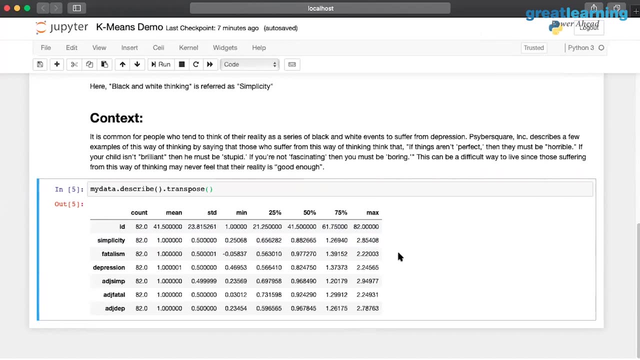 equal to 1.. Right, So that's something that I have to apply. Does that answer your question, Nathan and Rohit? Yes, Can you explain that again? Are you saying that the mean for all the attributes has to be same and standard deviation? 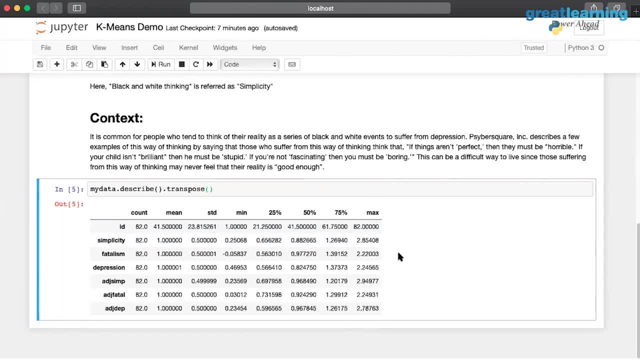 Yes, No, The mean has to be the same. The standard deviation has to be the same constant value. That's the undertake that you have for k-means. That's an expectation for k-means. Okay, And how do we actually? is there any library that actually help in standardizing? 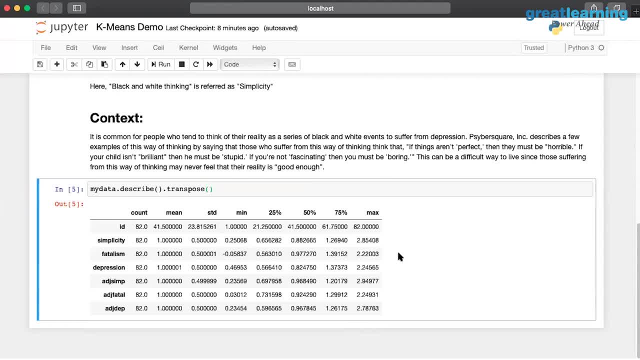 Yes, Yes, So you have this standard scalar right. Yes, A standard scaling. A standard scaling will convert the data to have the singular property, where the mean of all my values will be closer to approximately 0, the standard deviation will be 1.. 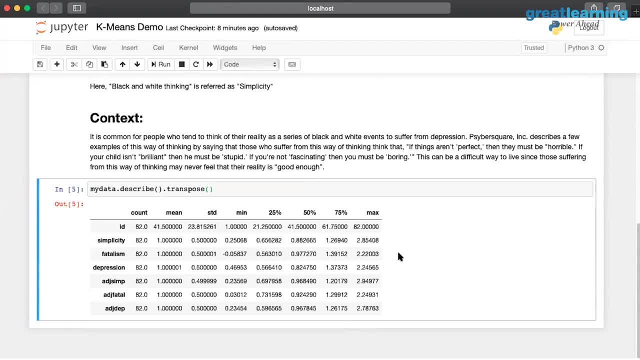 Right, That's a feature- scaling- So that can be applied, Shyam. Yes, Nathan, I think I tried to use standard scalar library but I was not able to use it. Can you just show it over here in this dataset? 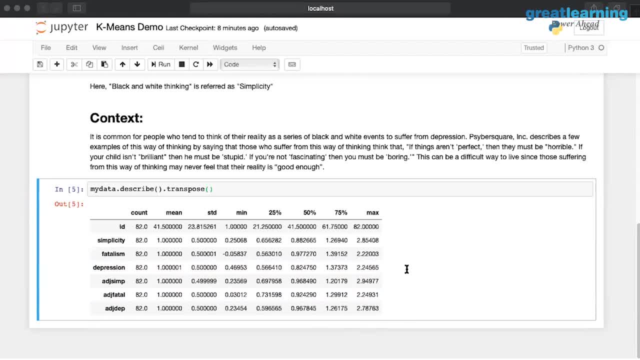 Okay, This dataset is already standardized. but yeah, I can surely show you the standard scalar here. Also one more thing: You said that if your standard deviation is different and the means are different, then you need to use this standardized data. 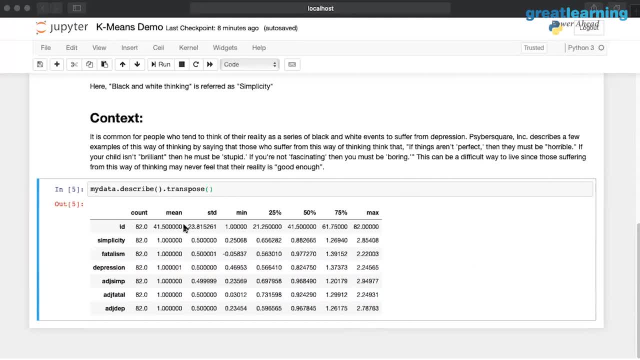 Correct. So just wanted to ask if this, because I was going to ask this question- I had used- I think, first of all, is it model dependent? or it is model independent Because I had used just logistic regression. Okay, Now, without it had a different data which was having a different ratio. 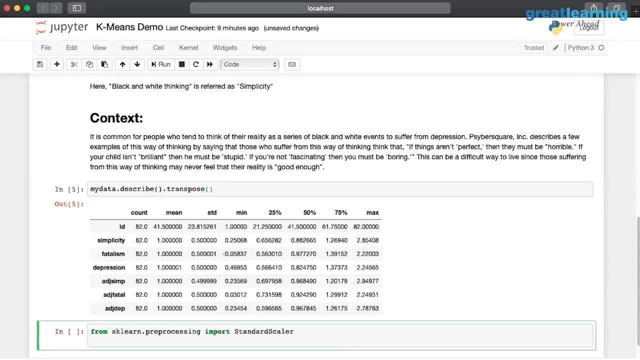 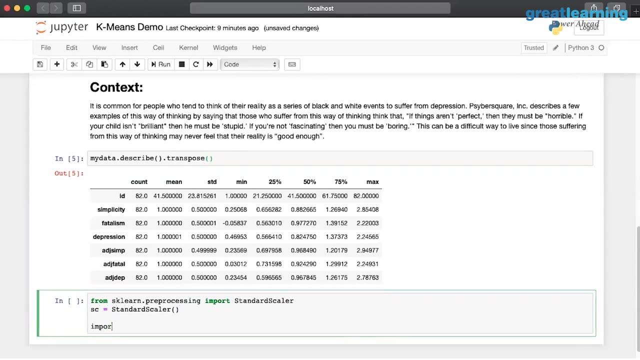 So might be. one was between 0 and 1 and other was having a range from- might be 200 in the range of the other attributes or in the range of that kind of a data. Okay, So if I try to use a, if I didn't use any kind of a scaling or any kind of a standardization, 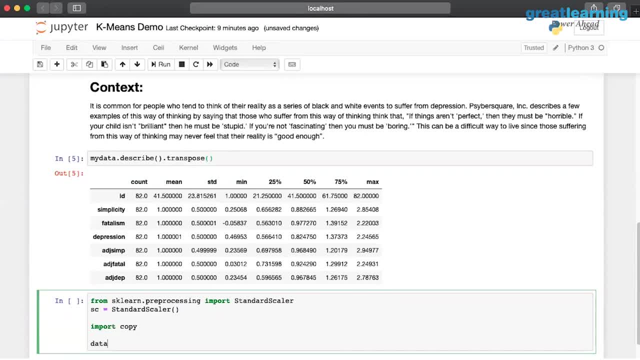 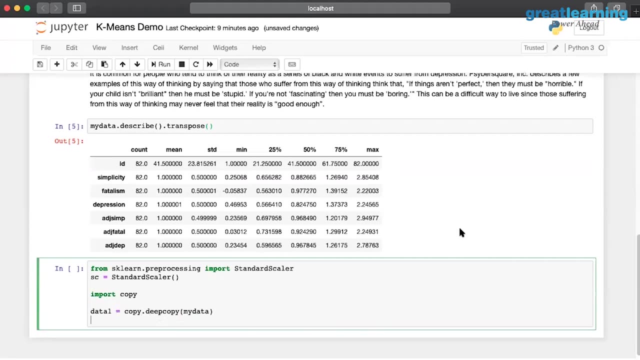 on that data and I use when I use build the confusion matrix on the based on the recall and the precision value. it was not varying in the sense that if I use the standard and scalar, only it was getting worse, not improving. 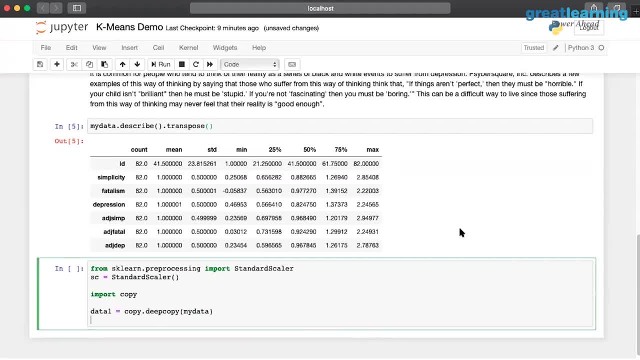 Okay, I think I remember you sharing this point during one of the project discussions, correct? Yes, Okay, So, Nitin, can we just take this offline? I just wanted to look at the data and the solution that you provided. Okay, 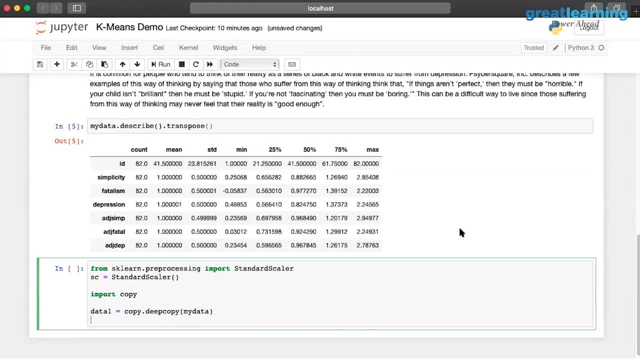 So before I make any specific comments on this, can we just look at the data and then look at the solution for this? Sure, So, basically it was. is there any kind of a definition, like you shared over here, like that standardization has to-? 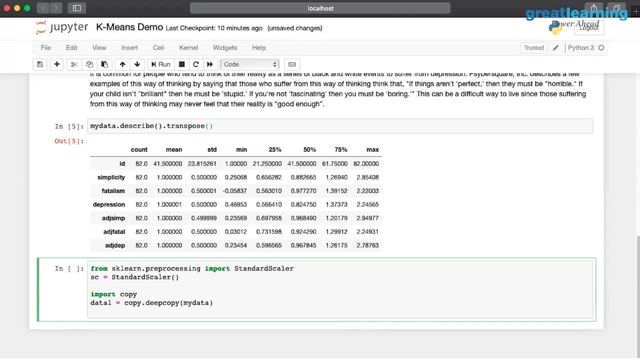 So for logistic regression there is no specific input that says the standard deviation has to be one. So that's specifically what came in. Only very specific algorithm have this expectation. So the regression algorithms expect that the target is able to be normally distributed. 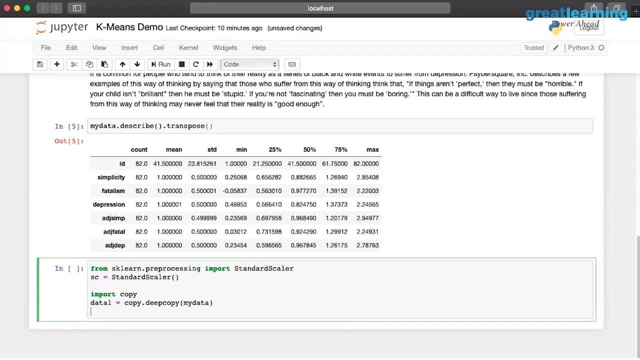 So that's pretty much it. There's nothing else that I'm going to specifically insist on that parameter there. So when you standardize the data, the mean will be approximately or closest to zero, All right, And the standard deviation will be one or in the third or fourth decimal. 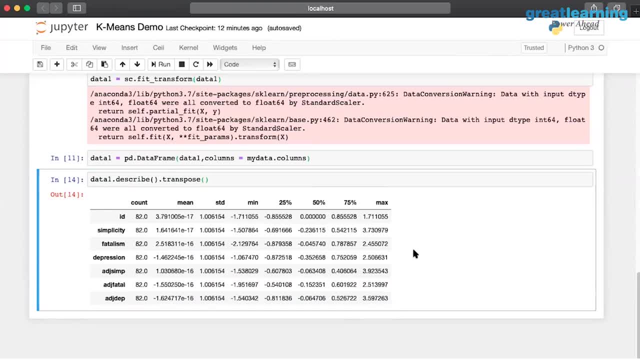 We usually don't worry about the third decimal, So we look at this. the property of this data as a standard, deviation is one and mean is closest to zero, So there's a constant value. So that can be used to build this table. 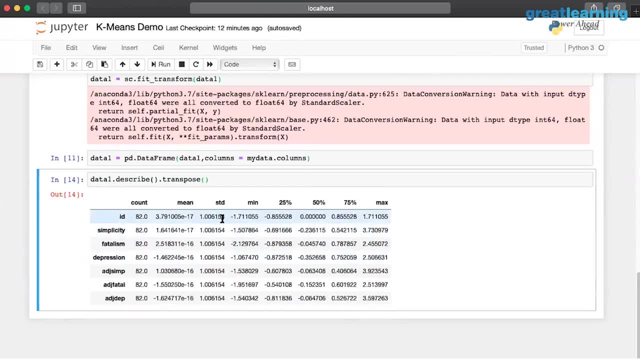 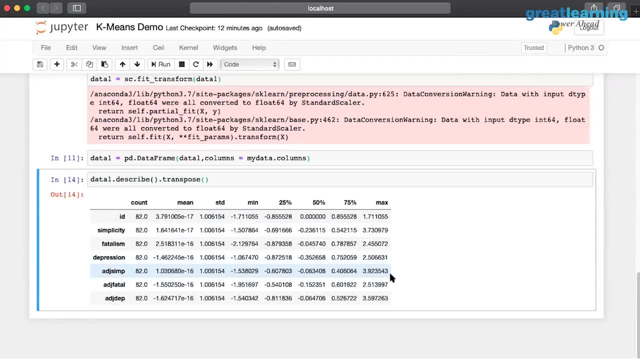 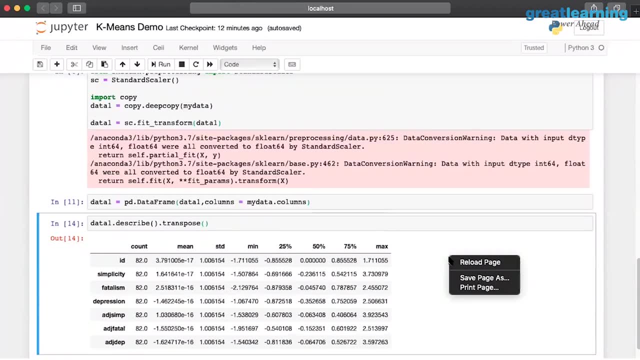 Okay, so that can be used to build this K-means algorithm on top of this data. So in other sense, standard deviation is basically the area under the curve. So we are just trying to get, say, the number of samples for each data into an equivalent. 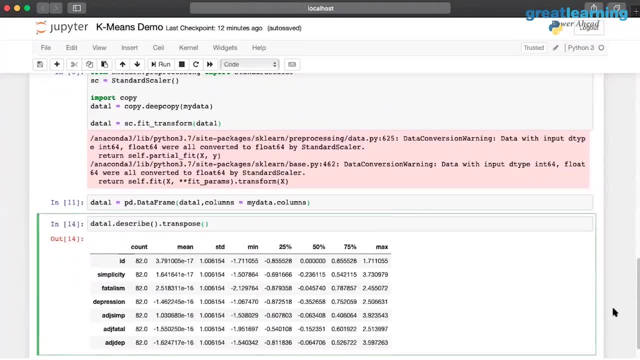 category Right. Yes, So standard deviation is not a standard deviation. if I talk about a normal distribution is a dispersion between the dispersion between the mean. So how is the data distributed around the mean? So I'm trying to get that dispersion as a constant value. 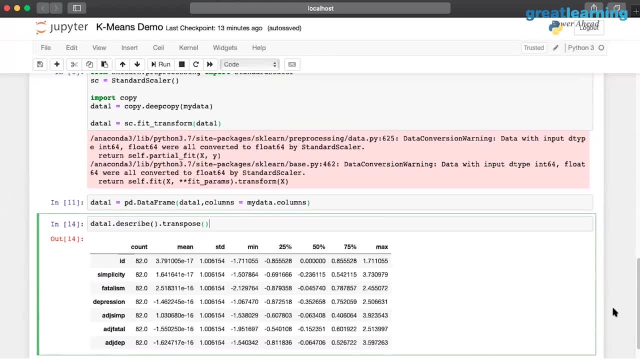 to all my data columns in such a way that they are ensuring that the calculation that I am doing. so it's basically Euclidean calculation, right? So the Euclidean calculation essentially takes care of a value that's very precise. That's the reason we do this. 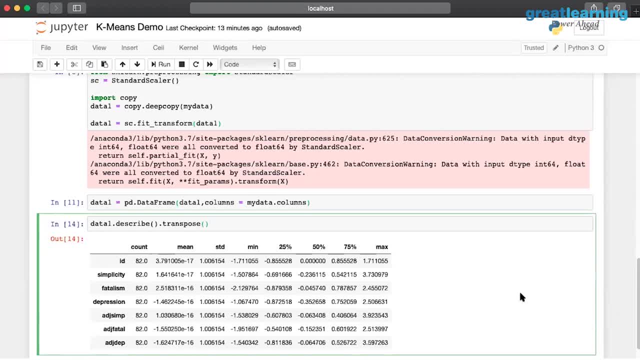 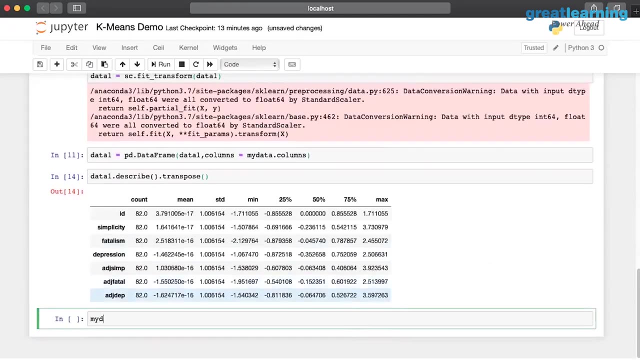 So we are just getting the means to a common value so that the calculation is more appropriate. there The calculation happens within a specific range. It is not dispersed or diverging too far away. So what I'm going to do is I'm just going to 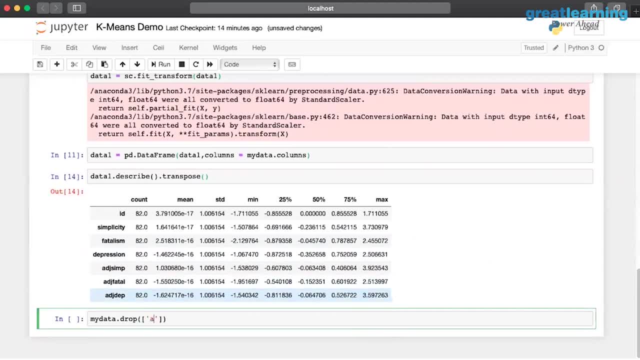 drop this other columns right now that I'm not going to use. So I'm going to use adjacent simplicity: I'm going to drop. adjacent fatalism. Adjacent fatalism: I'm going to drop. and adjacent depression: I'm going to drop. Now my data. 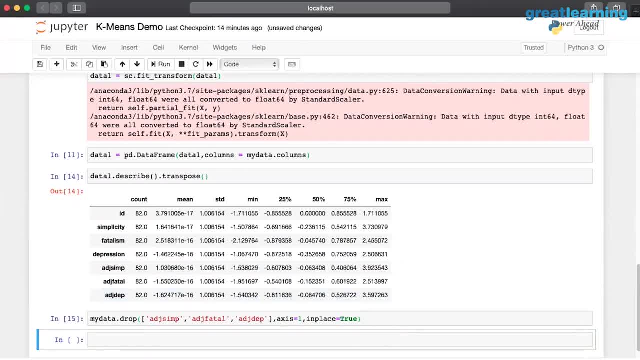 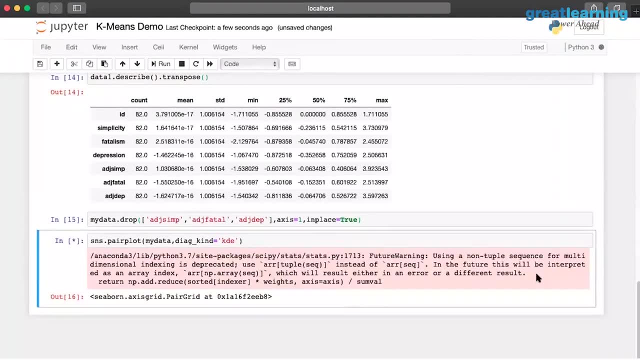 is ready to go. So a quick check. I can either use a KDE or a histogram Here. I just want to look at a KDE for a current density estimation. That's it. This is my diagonal for this specific model. So if you notice, 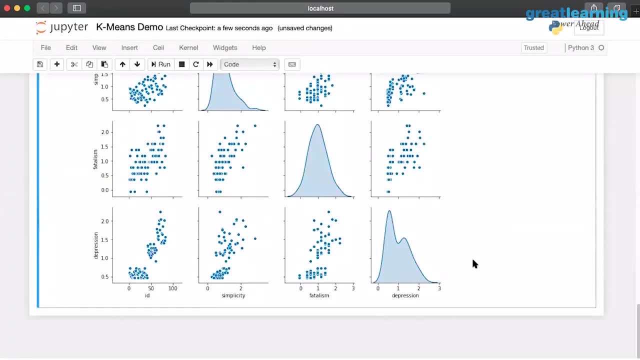 there's a relationship between what simplicity has with fatalism and fatalism has with depression and so on. So this is nothing but a grid where we can look at each value. Now here's a part where I'm going to calculate the ideal centroid. 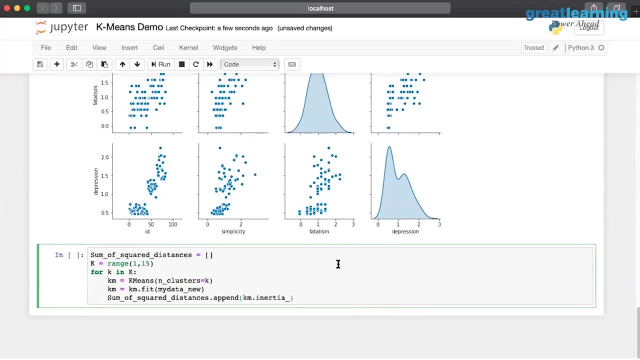 So I'm taking for 15 values, I'm taking for range of 15.. I'm diadrating between 1 to 15 clusters or 1 to 14 clusters and I'm getting the, let's say I'm getting the centroids of this. 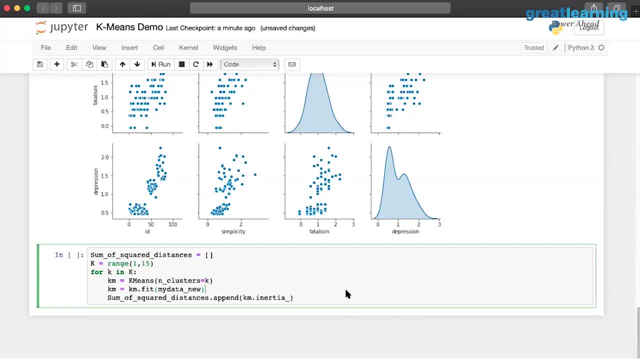 and I'm calculating the inertia. So inertia, remember we tell this is sum of square of distances. and I'm just calculating the sum of square of distances. here to now, my inertia is calculated. What I'm going to do is I'm just going to simply do a scatter plot. 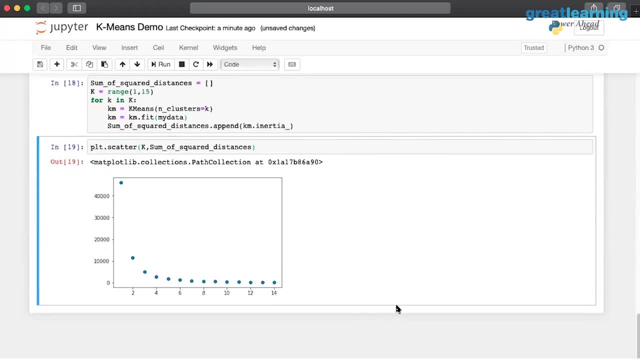 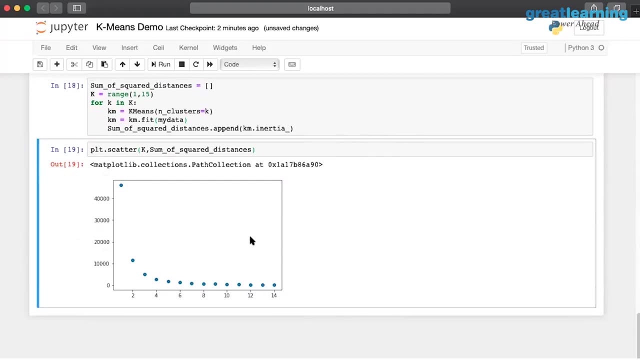 and I'm going to look at this bound Now, if you see that it ideally is either two or three clusters, beyond which I don't see a significant change or significant decrease in the number in the centroid values. Remember the same problem I told you earlier. 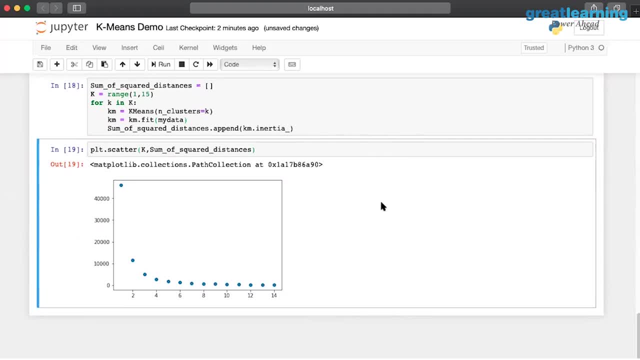 I just showed you an example where I have to have more than two clusters, more than three clusters, more than four, beyond a certain point, the sum of square of distances is not going to decrease at all. Now, that's something that we have to remember in that essential model. 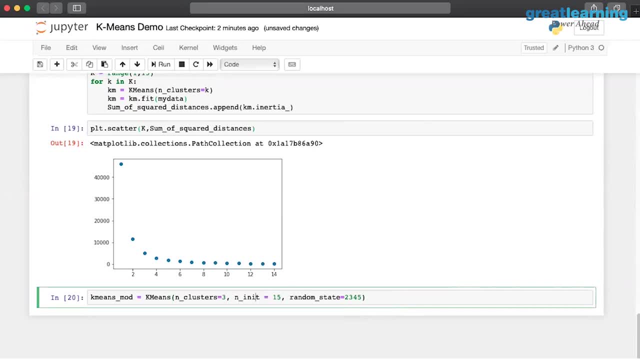 Okay, doesn't make sense, Okay, so here I'm stating that three clusters is ideal. Let's go with three clusters and using this n in it- and it is the number of initial centroid points that I want to start off with- and from these centroid points calculate, try and converge to a 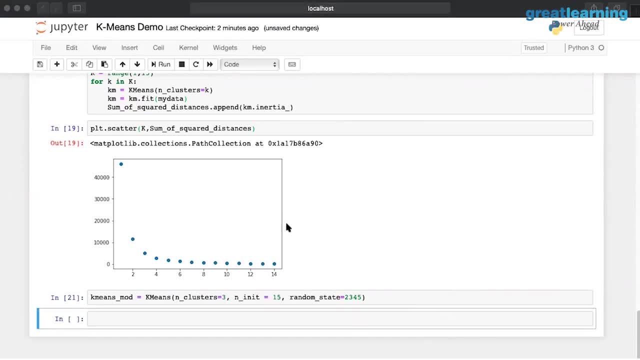 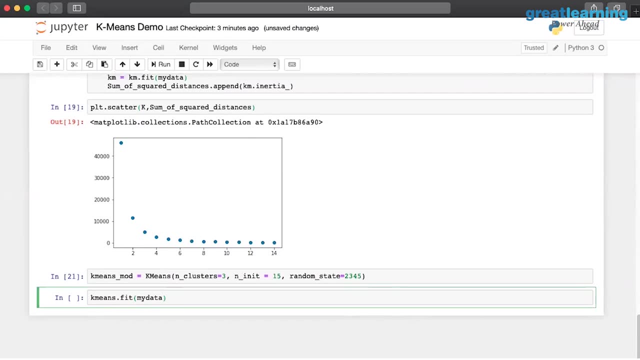 specific value. So I'm going to take a certain number of iterations to do it and I'm going to essentially achieve this model there. So I'm just going to fit my data here and to the fitted data I am going to now. now I'm going to open. 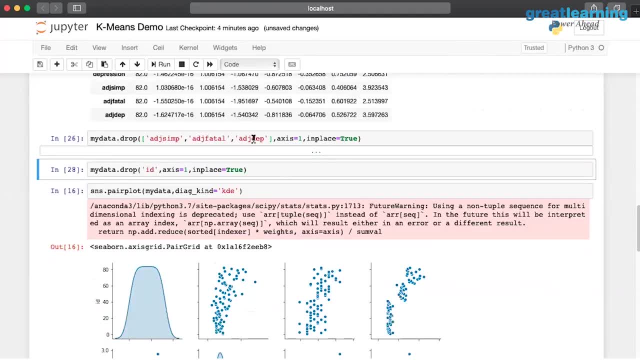 The error earlier was because the data did not have. so the error if you're talking about here in the previous line, number 26 of Chitra, because I've already dropped adjacent important, adjacent fatal and adjusted depression, so that's not going to exist in my key. 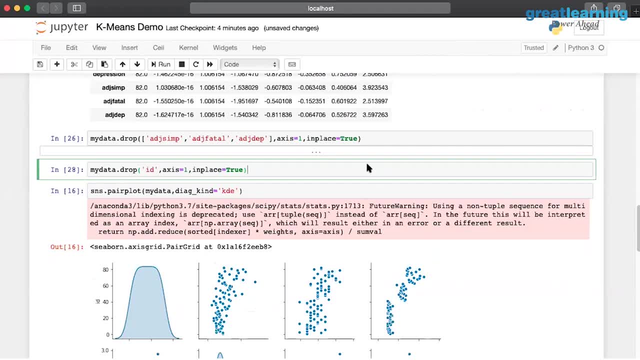 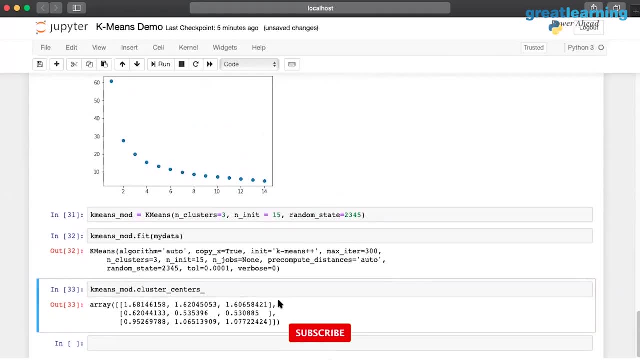 So the Python will throw an error saying that that key specifically does not exist. That's the reason it threw that error. And these are my cluster centroid right now. All right, so three, and even up to four, I will say, is agreeable. Two: 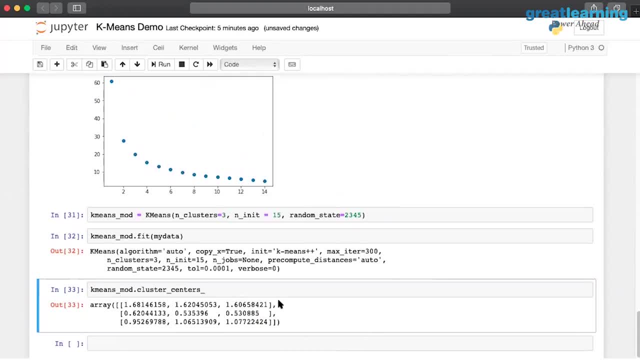 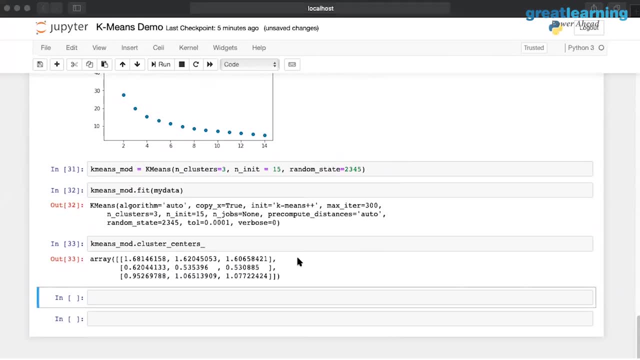 one and two as a major jump two and three as a jump three to four. I will still consider. so that's still acceptable, right? so I'm going to say three clusters and I can be right or wrong. Let me be honest here. I can be right and or wrong. so that does not mean anything here, because 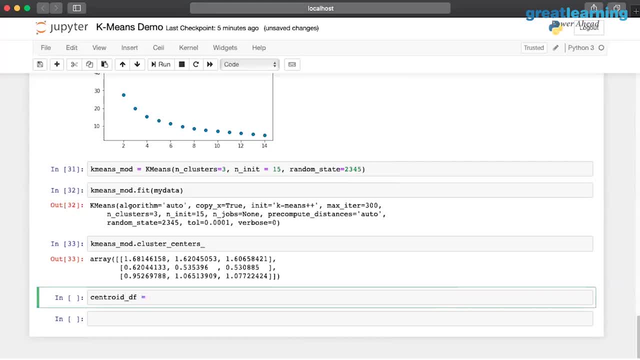 I'm essentially giving you this point where I'm saying two or three, I don't know which is the correct answer. I'm just hoping that the Elbow method is giving me the ideal cluster size. so I'm going with that aspect and saying that: okay, I understand that this is how it works. 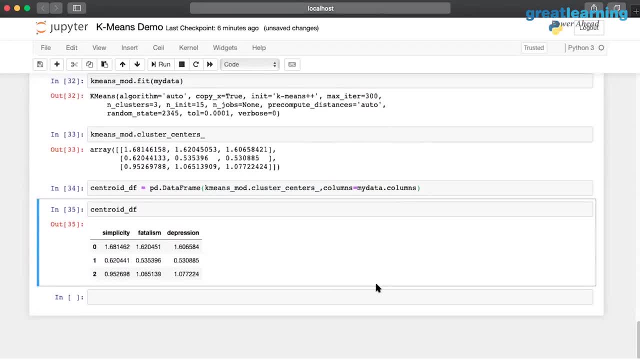 This is what we have. okay, Now, this is the key part. This is the key aspect of gaming. So you're going to look at the centroid value to maybe name, label or come up with values of a cluster. So, either way, there is not a problem there. 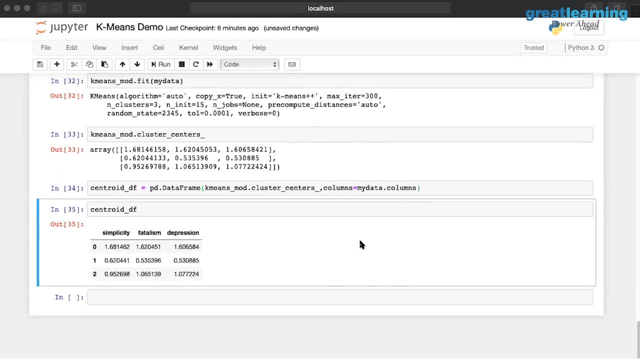 So you can just label or value Set anything that you would like and go with it right Now. what I'm going to show you next is how to insert this label into your dataset, and just going to show you how to insert this data In: how to insert this label into this dataset. 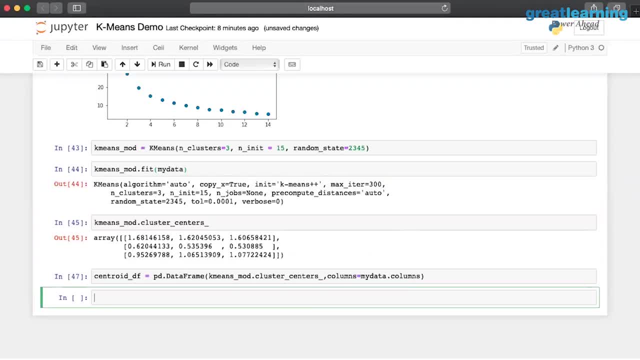 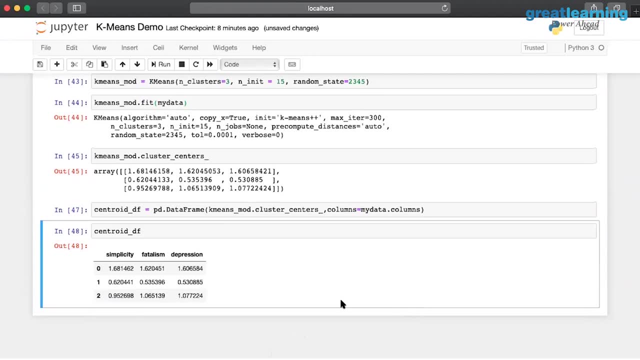 into your data set by adding as a separate data thing right now, if i print this centroid df. you understand okay, so now i can. i know that there are three groups or three patterns in my data, right, and i'm going to use these three patterns and i have three such patterns in my data. i know. 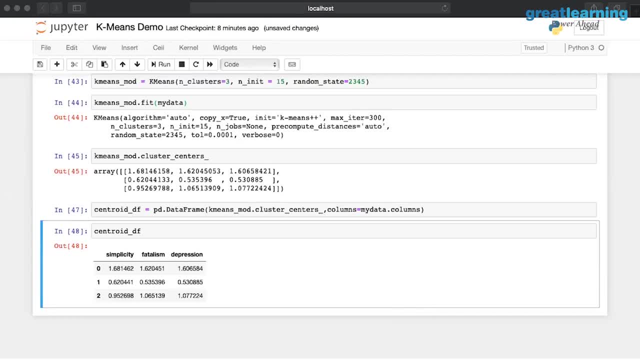 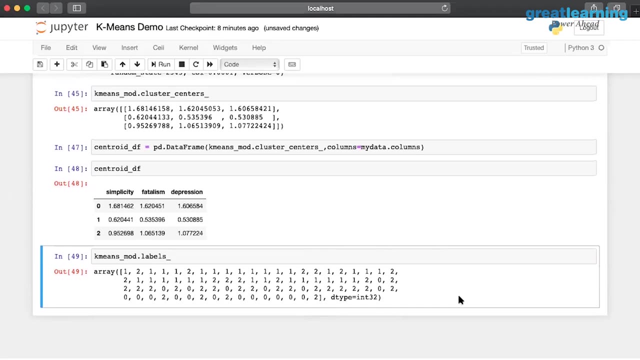 that this is a group, okay, but what to name them, how to name them? that it is up to left to the subject expertise: okay, now, if you notice, every, every target here is labeled based on the point, based on the centroid that belongs to. so i have 82 data points, all 82 data points, right now tagged. 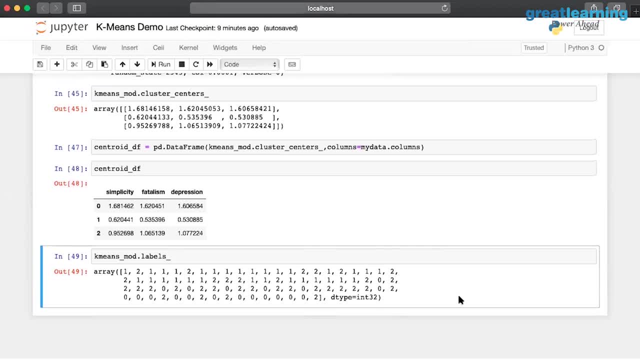 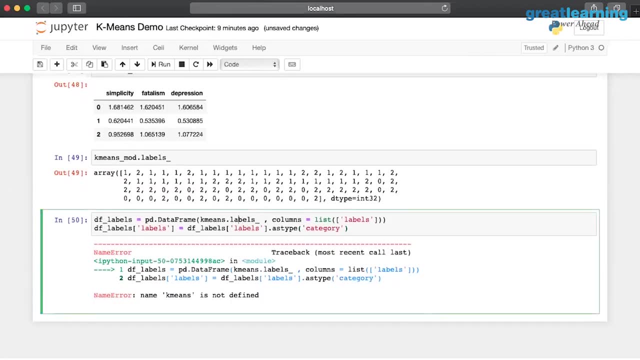 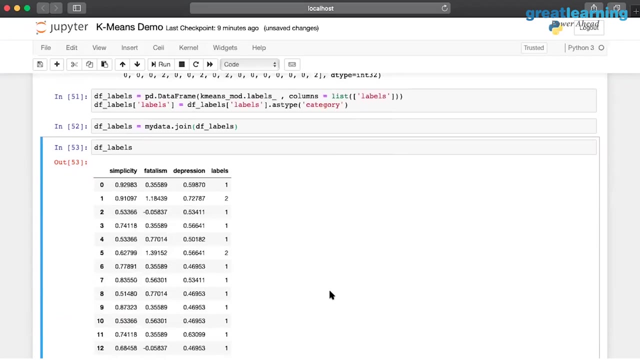 to one specific uh label group that i have. so i'm going to now create a data frame and i'm going to join this data frame there. okay, this is your final output, you, that you're essentially going to take. so i have each group, each observation, tagged to a specific. 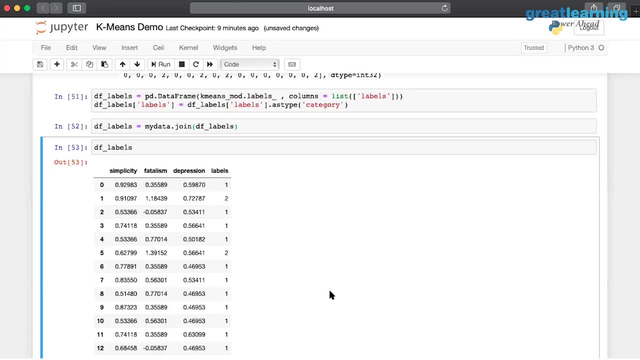 group and i now can analyze now from here, from an unsupervised perspective. i now have a group value, i know what each group average value is, which means that what is it representing? which group, where does it belong to and how does this specific observation, how to tag or name it that i can leave? 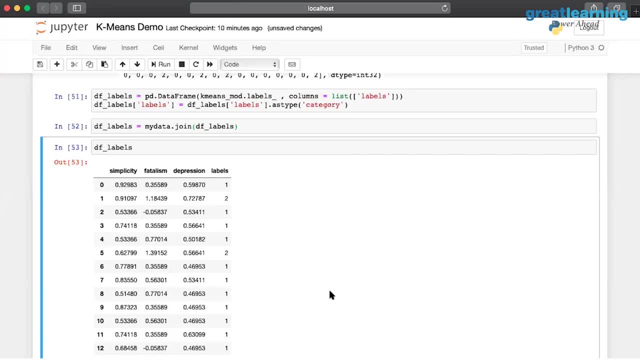 it to the expert subject matter experts. but i now can understand. there are three patterns, three to four patterns in the group, or even two patterns, and i can work with creating these patterns in the data point. all right now, this is what i had in store for you today. any questions we can? just i just missed out. can you just explain these values? 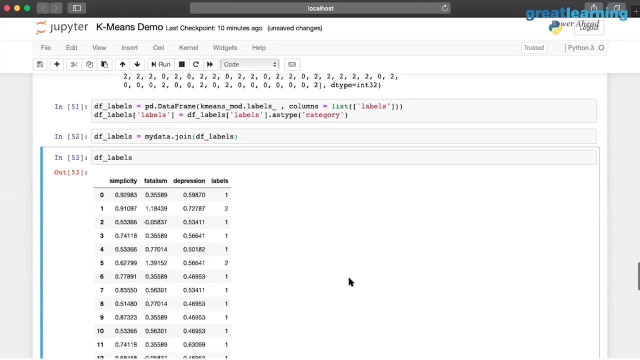 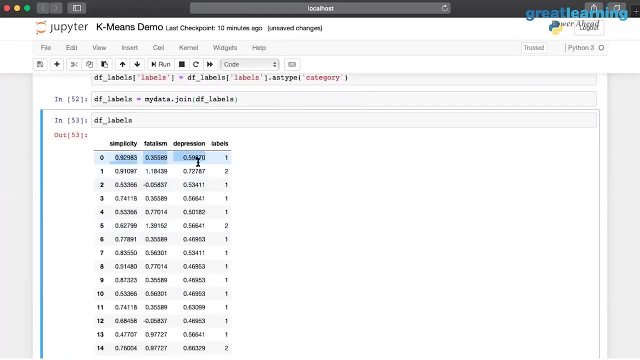 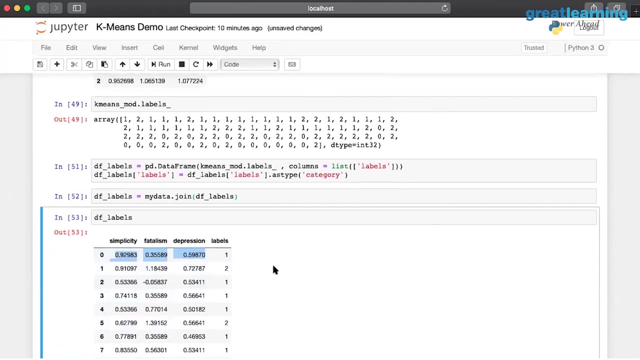 that were coming out in each data set. can you record 0.9 to 0.359? yeah, this one, yes, yes, yes, you mean this one. i either of them, because i think they are related. yeah, this is the raw data. so what you see here is a raw data. uh, nathan, so this is this is the actual data frame, and the k means has. 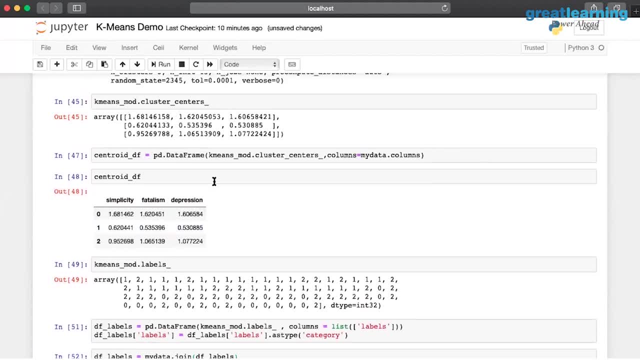 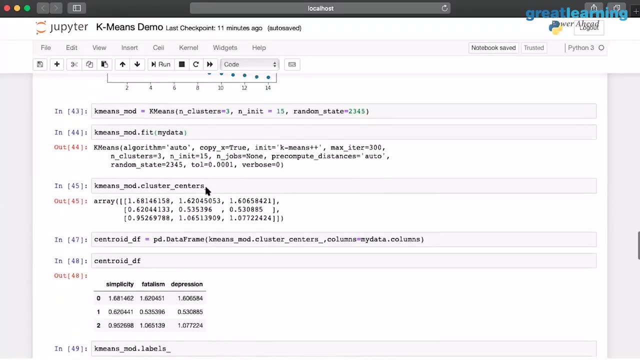 essentially tagged, say, based on the center, i told you. it calculates the distance, it creates a cluster and it tries to set this point in the middle of the cluster, correct, yes, right. so it has now calculated that this specific data point is closest to the first cluster, right? so that is how it is tagging it, basically, when it is training it. 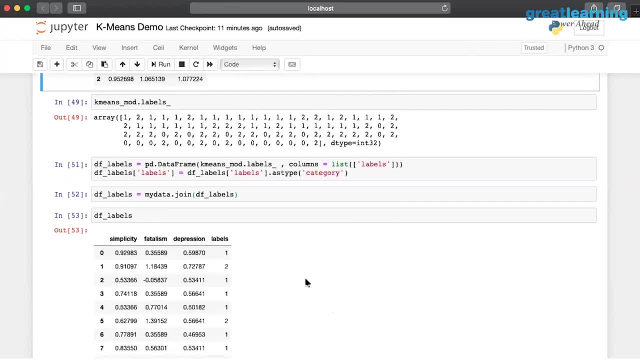 is tagging based on euclidean resistance. it will create a centroid, find out groups in the data and merge this information to the centroid group of the data point. that is what you see here as values, so it's the raw value and which group it belongs to it. it it is showing the distance of. 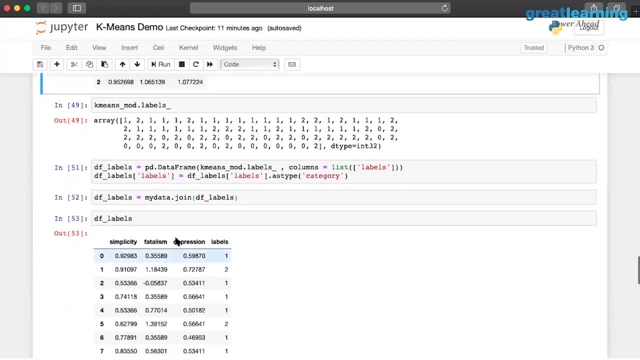 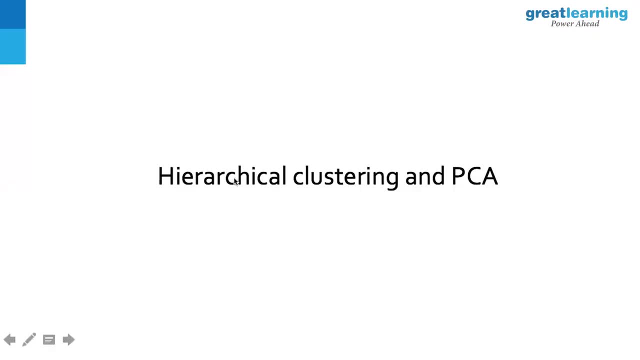 from simplicity, uh, cluster and the raw data. what do you see in the raw data? okay, okay, this is the data values for each. yeah, this is the actual data value, the absolute data value. all right, so a couple of things. we're going to talk about what hierarchical testing is, and then we're going to 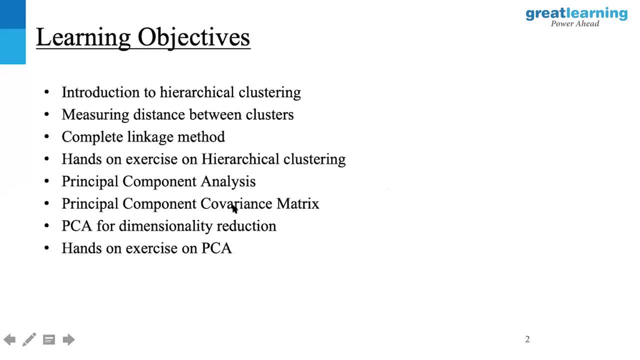 look into what pca is. all right, so pretty simple stuff. or hierarchy testing is probably one of the most simplest algorithms. so what we have is: let's say i have, i'm going to talk about a clustering approach that uses a complete data and i can, i'm going to choose only the cutoff based on the top. 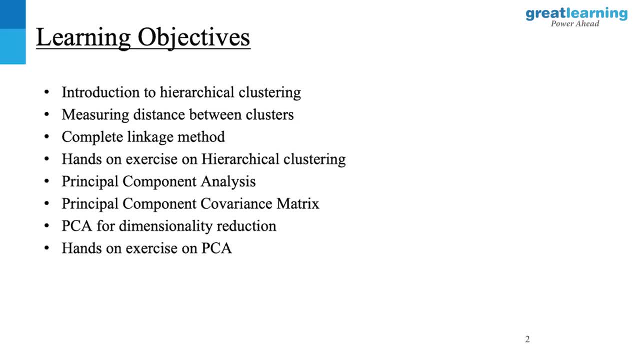 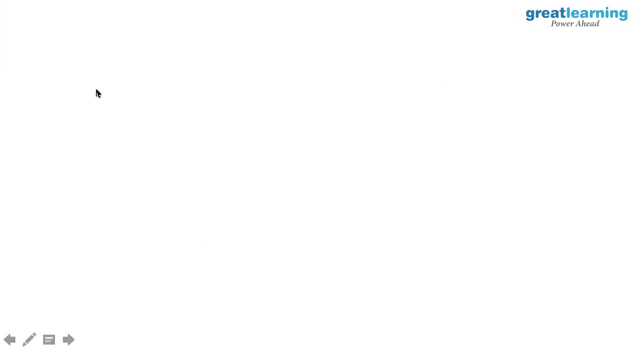 end features. i mean a top or the hierarchical list that i have. okay, now, what do i mean by that? it's very simple, okay. so let's say i, let's say my hierarchical thing treats my entire data point as a single, unanimous value, so it ideally treats the entire data. so let's say i have a data point that i have here. 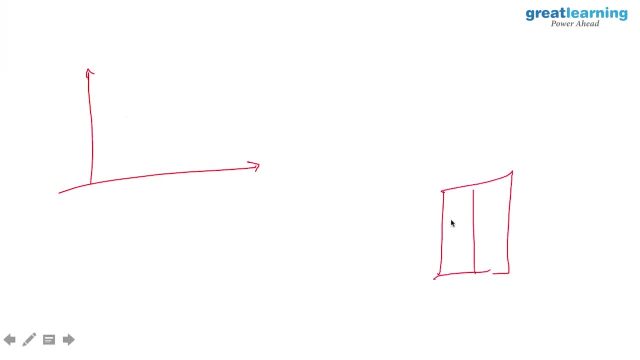 now what let's say. i have a data that's like this, and hierarchical testing is purely based on the distance. now it is going to calculate the distance from this on this objective point to all the other neighbors, from this point to all that neighbor. so ideally it will be a distance matrix by where it's going to be. uh, row number one, row number two, three, four. 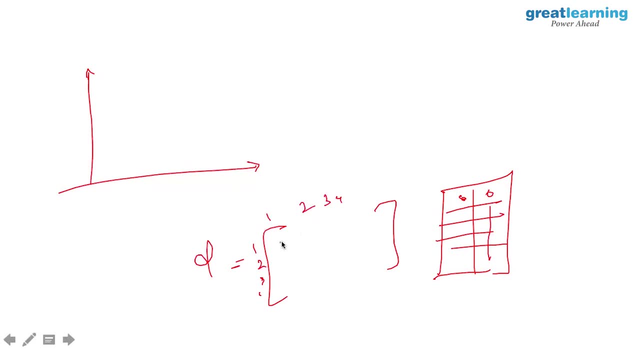 one, two, three, four. so it's going to calculate what is. it's not going to calculate one to one, but it's going to start calculating what's. two to one, all right. and not two, two, two. so it's going to be two, three, five and so on. it's gonna just fill this matrix now. based on this, what's gonna happen? 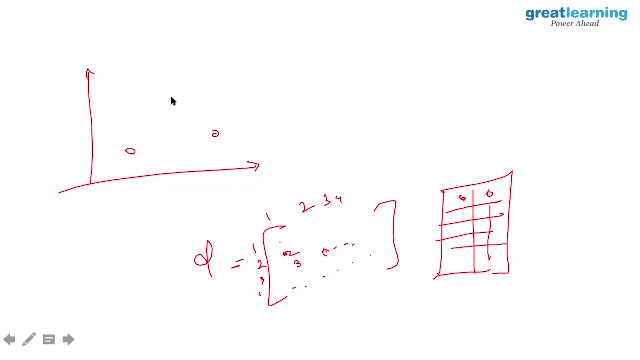 is that all my individual points are treated as a cluster themselves. okay, now all my points are initially treated as cluster themselves. so what happens is it's going to start combining clusters and the map of it is going to look like this and initially the uh hierarchy testing map. 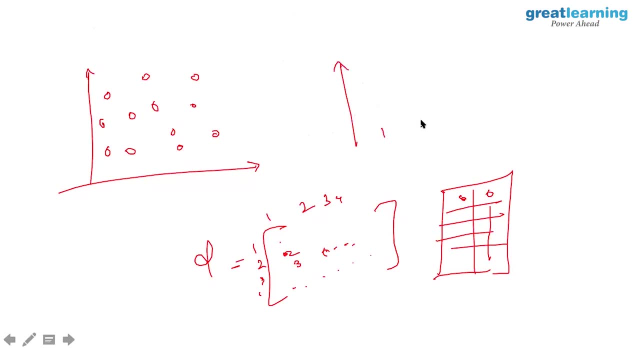 with its ls, with the height, is going to start looking like one, two, three, four, five, six and all your points. it's going to combine one and two. it's going to combine two, a three and four. eight is going to combine whatever next the nearby objective. so if it's nothing, as well it's going to 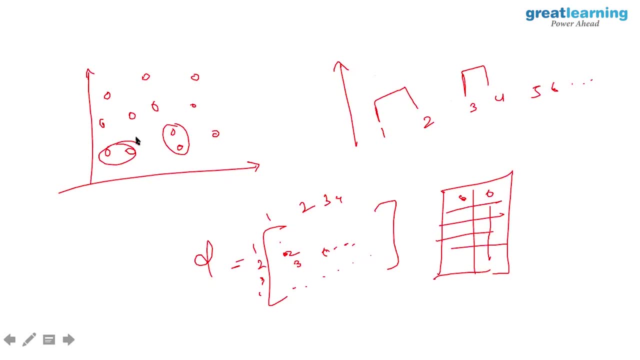 stop this. and what it is also going to do is next level. it is going to now combine the next set of nearest objects, like so, in the next level of distance value it's going to combine objects. so all right, so it may combine, say, uh, five, and 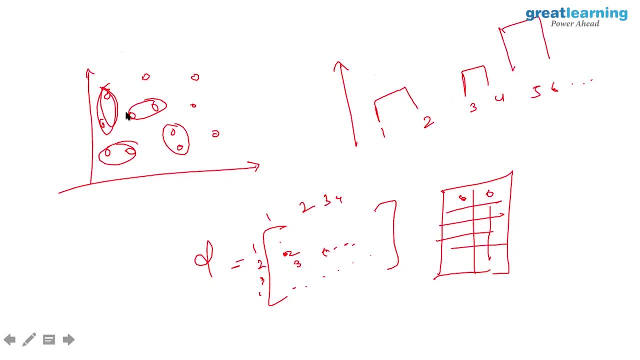 six here and so on. so it from here. it is now going to start combining or creating a single cluster value by joining these two clusters together and the, or rather, which are the next two, next two that are closest to maybe, these two together and then these two clusters. 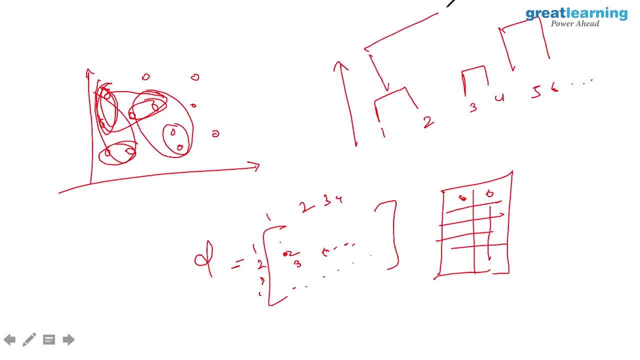 together. so it is now going to combine, say, one and two with five, uh, three and four, and then five and six to this. so it is going to keep combining individual data points at back into clusters until it reaches one single whole cluster. that is what we call as a hierarchy testing. so this is a hierarchy. last thing has top-down and 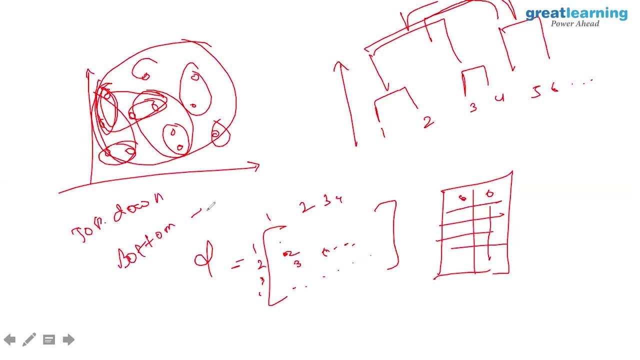 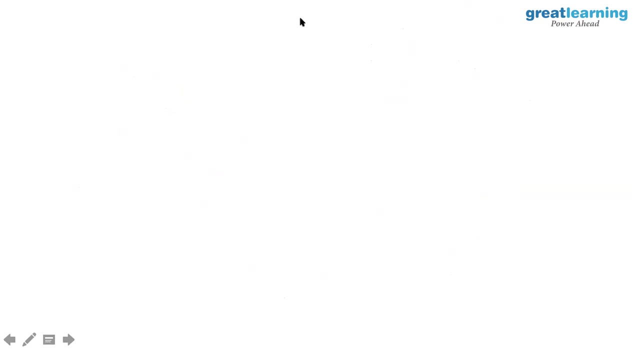 the bottom-up approach. so this is what we call as a bottom-up approach. so basically, we're going from the bottom, from every individual element to the final most value. so this is called- and this is your hierarchy, clustering in a nutshell. so it just calculates the distance from these objects slightly. 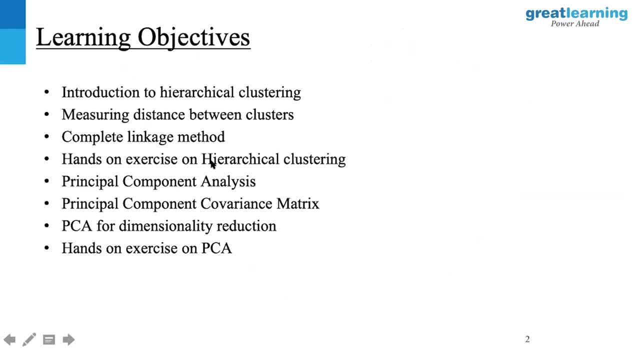 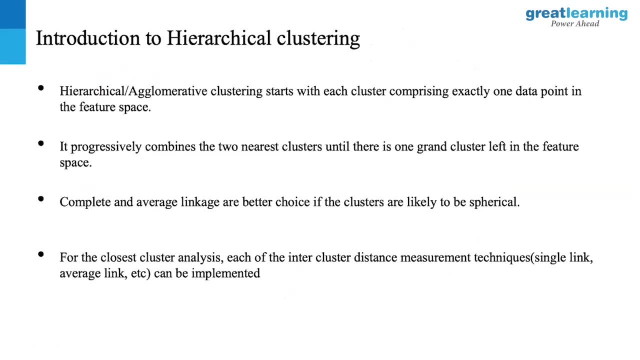 differently. so we have the linkage method, so you have the complete linkage or we have the median, the average of the linkage. so all around these different things, and it essentially works around that way. all right, so this is what we essentially say- is your hierarchy clustering method. so when we have the 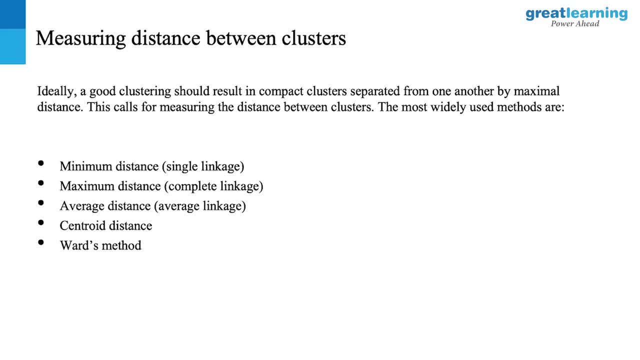 measuring distance between clusters. we have what you call as a minimum distance. there is a single linkage of value that we can look at and the maximum distance, which is the complete linkage, the average distance between the, the distance between the points, if I am, if I'm clustering more than one right, if I look at I'm gonna. 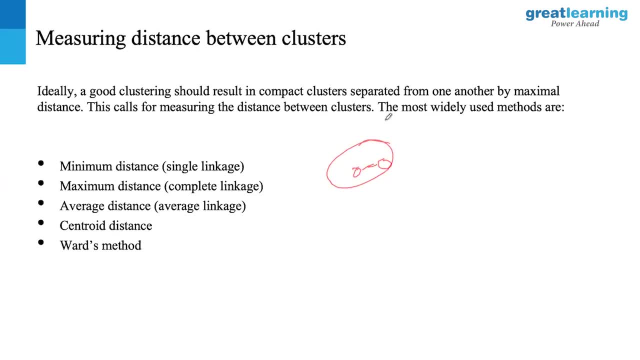 cluster more than one. so what is the average between these two? combine that with the next nearest objects that have the similar distance and then put them in the map together, so this is called as average, and centroid, which is nothing but the center of this entire cluster segment and the watch method. these are: 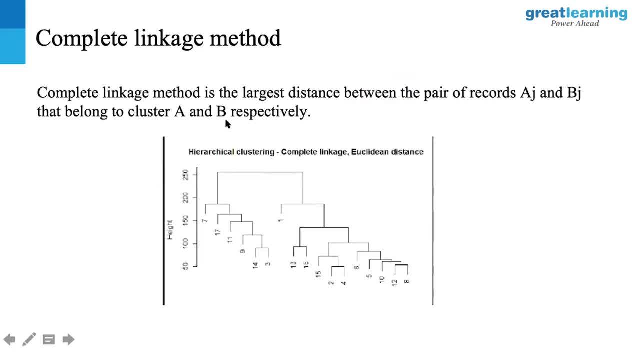 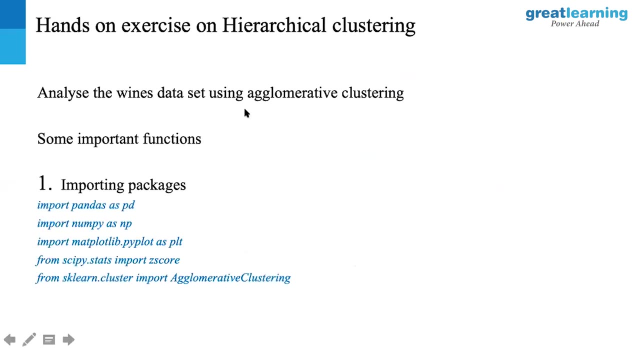 all different cluster linking methods that we have the complete linkage method. it just can find the largest systems between the pair of records a and B and combine to a and B respectively, so it kind of joins. as I said, the height of it is nothing, but how it kind of joins them together is about how to implement it. so 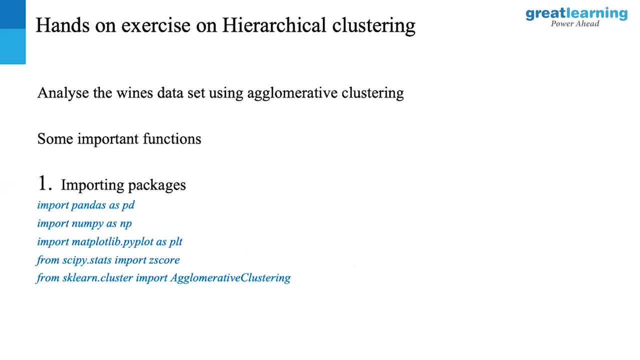 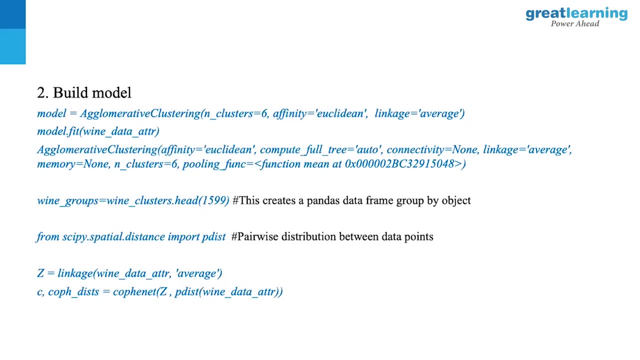 you have, inside the cluster viewer, imported canines last time, so here you are going to use this agglomerative clustering package that gives me, okay, the number of clusters I want to create, the affinity it should be pleading distance and the linkage can be right. this can be. it should be equal to the number of clusters that I want to create. 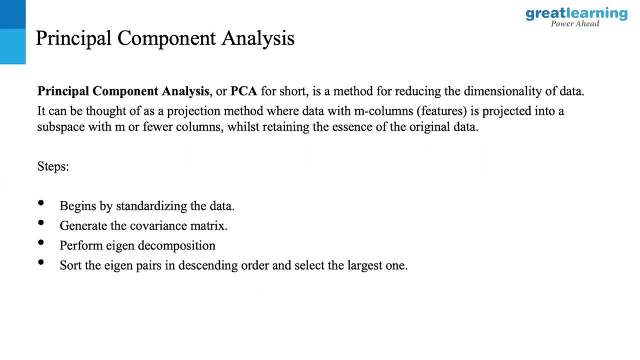 average or whichever I'm essentially choosing. So this comes your principal component analysis. it's a very, very interesting technique. It's a very, very complex technique, but it is also a- Yes, somebody has any questions? scaling is basically converting everything into a. 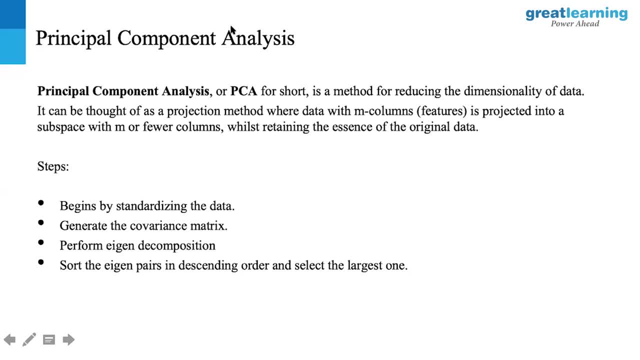 uniform distance, where it can have a scale of 1 to 100 or 1 to 1, but everything on this scale. So you change it, one unit will be equal. equivalent for everything. Correct Normalization is basically converting a Gaussian distribution, converting into a Gaussian. 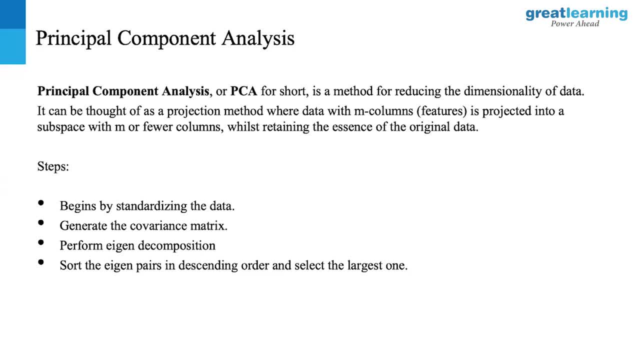 distribution. So my question is: we can use either of the two for this or it has to be scaling. And second thing I wanted to ask is suppose we are using a PCA as well as some model building. for, say, at an initial level, before PCA, I want to build a certain model which uses 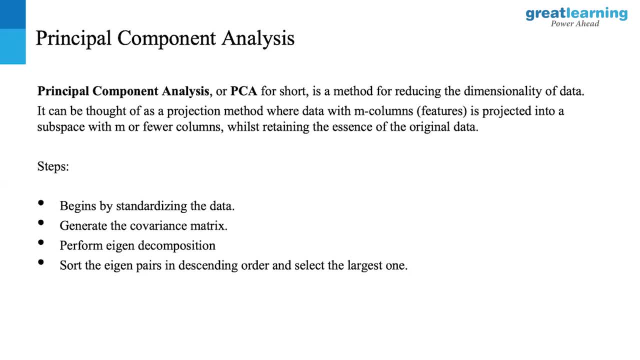 let's say k-means. So when I use k-means I might do a scaling feature on this data set Right. So now do I need to normalize the data while using a feature, say PCA, or vice versa? 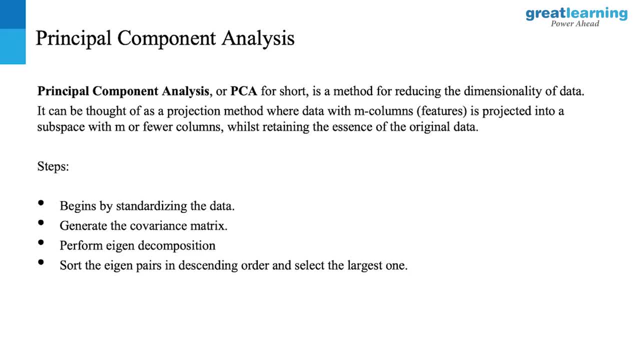 So my question is: So when you use standardization already, do you want? should I normalize the data? Yes, yes, yes, Ideally one of these two, All right. So if my data is going to work on Euclidean distance principles, I would scale it rather than normalizing it. So at any point of juncture, 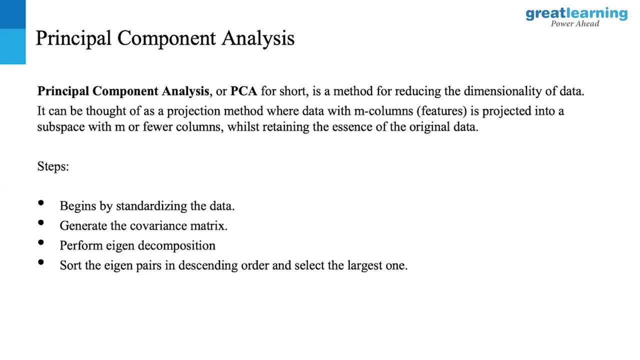 if I'm going to use a data, for example your k-means or k-n-n, these algorithms are working on. Let me give you a example. This is actually two skills которat I'm working on here. The first one is called lines, and that is let me just show you how to normalize the data with. 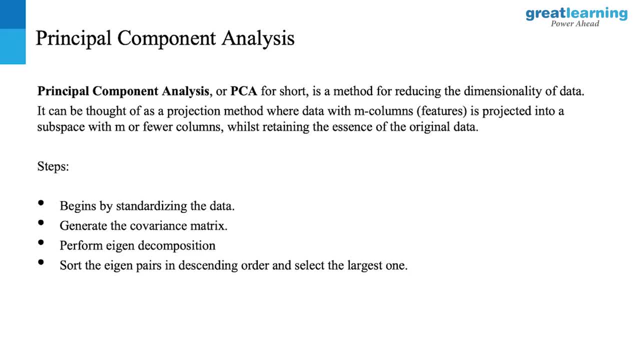 you. So this is basically Euclidean distance, basically calculating Euclidean distances. Now you're creating this since it's basically calculating religion, business. Now, in that context, I would have this data standardized as opposed to normalize. Now, where I'm going to use normalized or it kind of gives it gives you between this Gaussian. 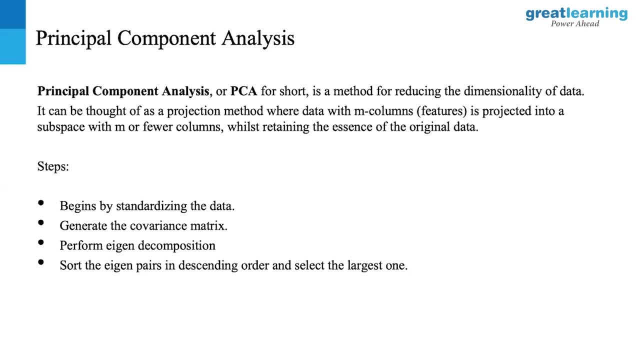 distribution range Is when my data independent values have a lot of these- to between zero to one values, and I want Mike in current column also to have this normalization values. I to one keep it restricted to itself, so that's where i'm going to use a normalization as opposed. 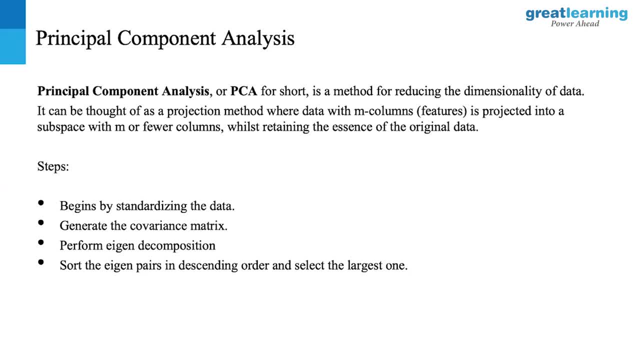 to my uh. standardization with the with any set of algorithms does answer your question with them? partially, yes, but if say i have uh, i'll say uh, two or three models which i am trying to run on a given data set and one of them uses a. one of them can basically work on a scaling, scaling factor. 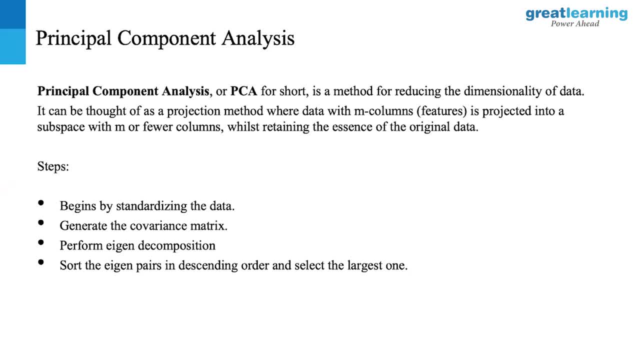 right. so once i have done scaling, now i've come on to a second uh model. so is it required to? if it's not, is it required to do the normalization again on on those features, on the scale data or on the scale data you will not normalize. so on a data that's already scaled. 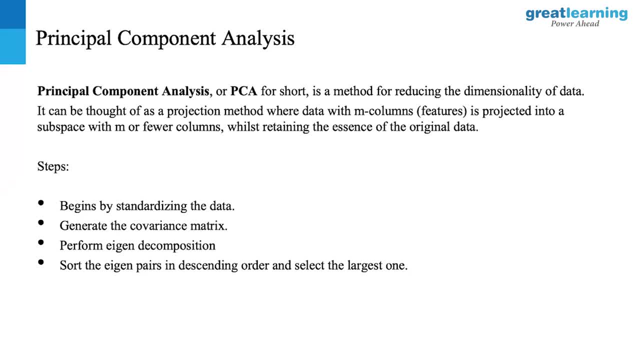 i'm not going to normalize. the reason we scaled it is: there's a behavior that we expect that it has to have a constant mean and the constant standard deviation. you have to have a constant mean and the constant standard deviation. uh, k means has this expectation and, if you notice, knn also has a partial expectation where the data 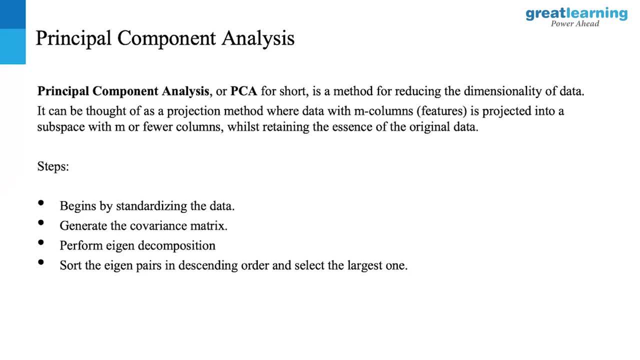 has to be in a specific format. so, uh, because the k means, or knn, is affected by variance. now, variance, and i say this, it's just basically the spread of the data, right? so, given that if i have already standardized the data, i am not going to go ahead and normalize it, that that will not. 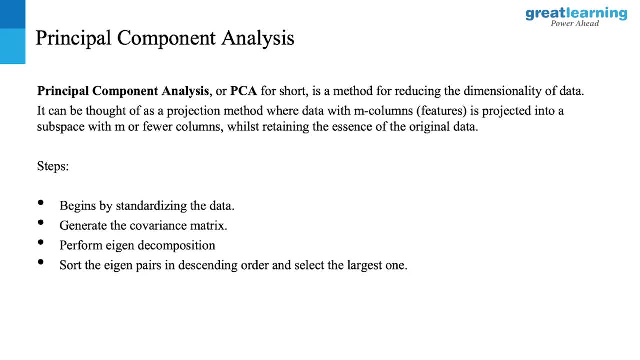 make sense in that specific spectrum. so to answer your question with probably a little more simplicity: no, i'm not going to standardize the data. i'm not going to standardize the data. i'm not going to normalize the data that i've already standardized. i might keep the raw and i 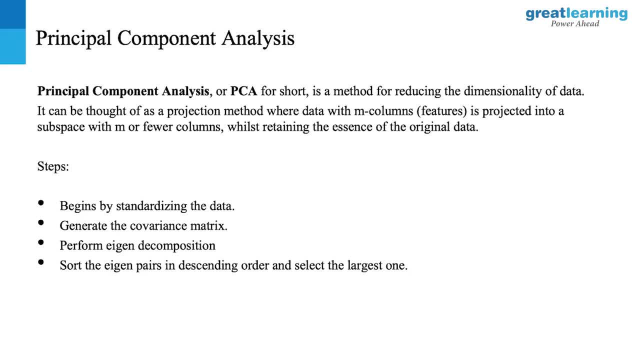 might normalize the raw data to work for that algorithm, but i'm not going to standardize. i'm not going to normalize the standardized data. okay, now i'm going to talk about principal component analysis. now there's another dimensionality reduction technique. it's called as factor analysis. 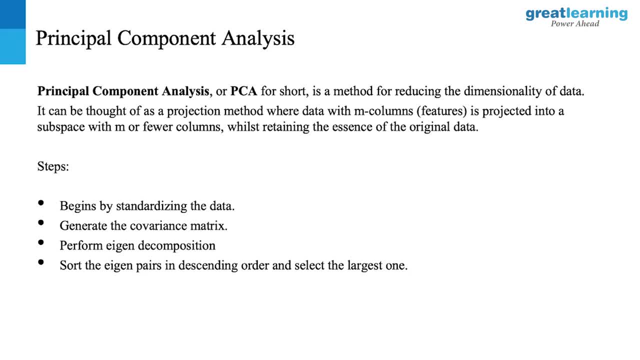 now, the prime objective of principal component analysis is- if you remember one of our questions, one of our model expectations- that the data should not exhibit multicollinearity, correct. that was one of the conditions that linear regression specified. now i also want to use this algorithm if i have too many dimensions that i'm not able to use. 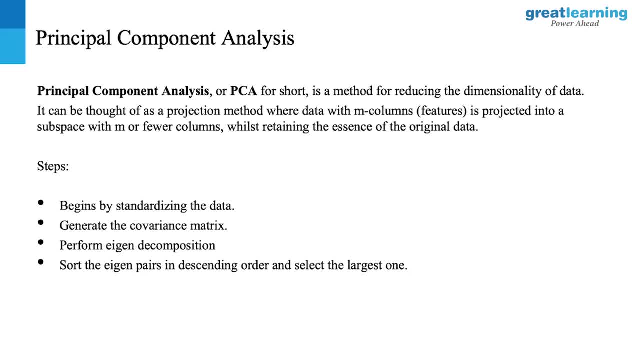 that i cannot, that i want to use but i cannot directly fit them into an equation or kind of come up with individual variables because statistically they might be insignificant individually, but in in perspectives of how these variables evolve on, in perspectives of how they help me understand my model, that's, it's going to be quite a lot now, given that i want to do kind of reduce the. 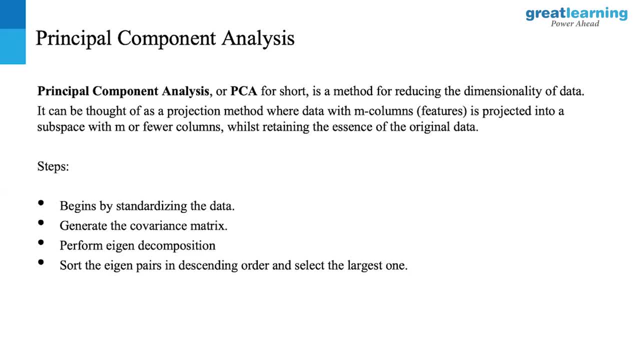 dimension. so this is a method that we call as feature engineering. one of the methods of feature engineering is featured elimination, the other is feature selection and the other is dimensionality reduction. so here i'm going to do about, we're going to talk about the dimensionality reduction. 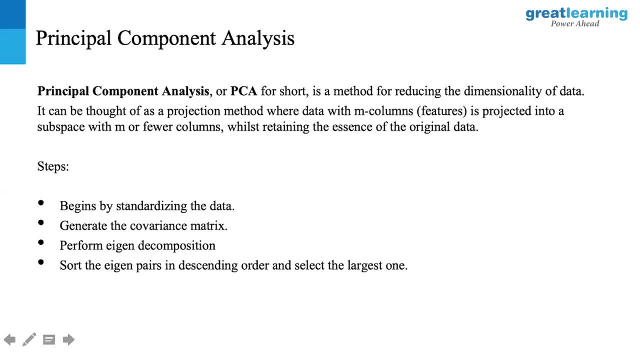 where i'm going to reduce the number of dimensions that i have and work with the subset of our dimensions. okay, so the components with pca is nothing, but it will transpose the dimensionality of the degrees and this is called distribution. the dimensionality of the region is based on the dimensionality of the area of the group or the distance between each. 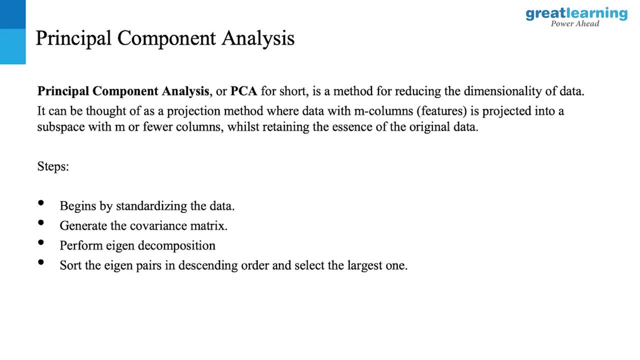 uh region. so it will be determined by the distribution of the element with the dimensionality of the area of the group, and that's what i'm going to talk about in a moment. i'm going to also explain about system validation to you again as we go into thelimitation part of generative 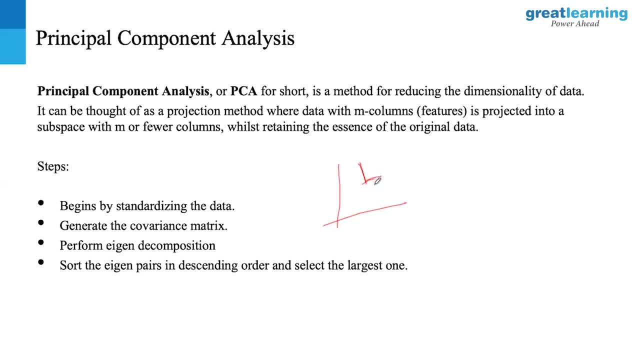 applications. if i want to do a look at the two types of statistics, it is a pretty complicated approach of posted configuration or can we just take a look at the three kinds of systems that i've discussed is the first one is called system development and the second is called system. 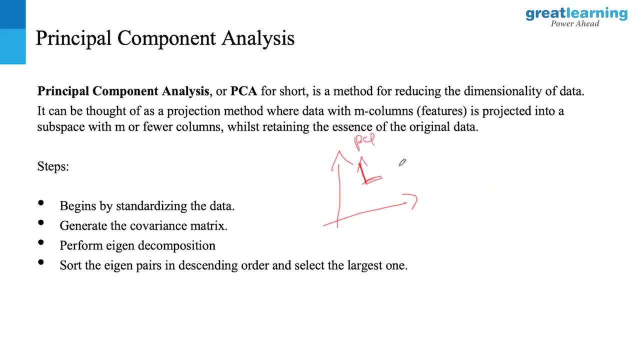 value. it is always going to be perpendicular. the pc1 is always going to be perpendicular to pc2, the principal component one. it is always going to be a component to a perpendicular to pc2. it. this pc1 will load a specific set of variables to its dimension. pc2 load a specific set of variables. 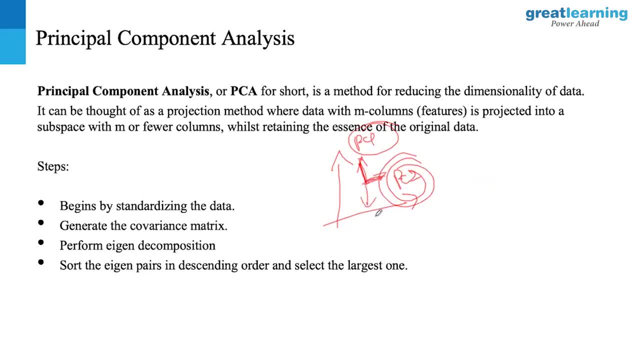 to its dimension, but they will always be perpendicular. even if i have more than one pc1, pc2, pc3, all of them are going to be perpendicular to each other. all right, and we're going to use- uh, if i want to choose a proper principal component, i'm going to find a. 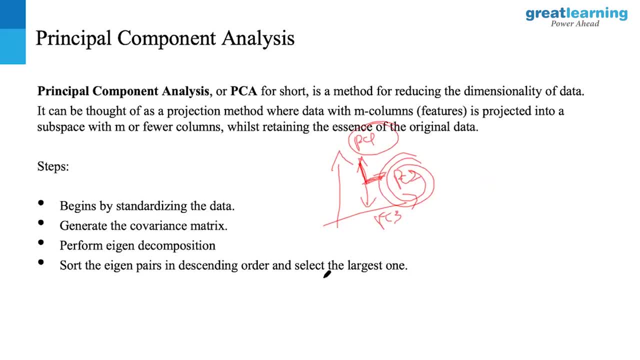 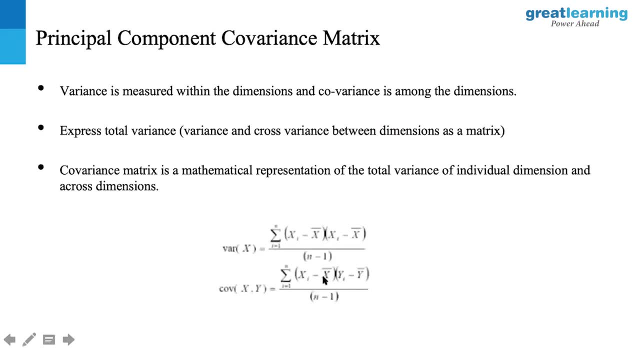 continuation of how much of covariance they were the data explains and choose the specific number of principal axes based upon that value. all right now. first i'm going to measure the variance and the uh within the dimensions and covariance among the dimensions. all right, so if i want to talk, 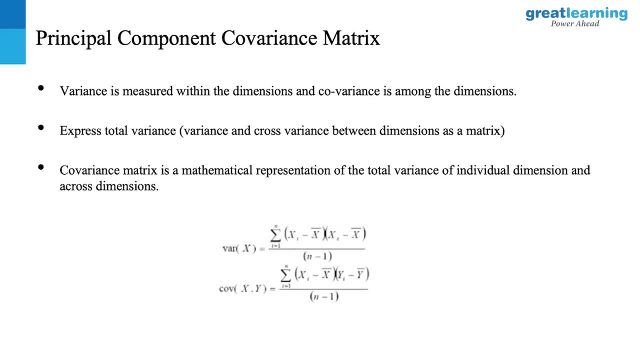 about total variance and covariance. it's a very simple formula. i'm going to talk about x minus x bar into xi minus x bar. all right, that's. that's nothing but x minus x bar. the whole square and the covariance of between two variables is x minus x. 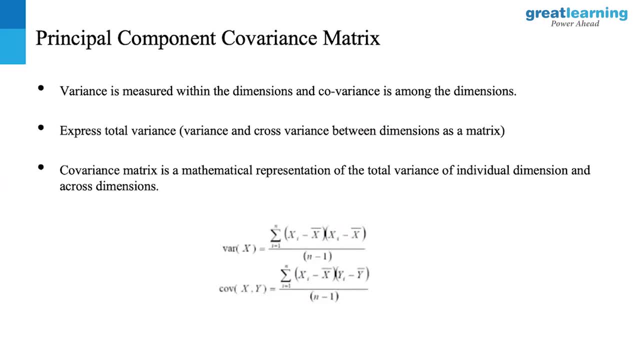 bar and y minus y bar by n minus one. so summation of all these values, it's kind of an average value, right? so the variance is how much how the data is spread across. right, the variance is nothing but how far the data is spread across. the covariance is how tight is two things knit, or? 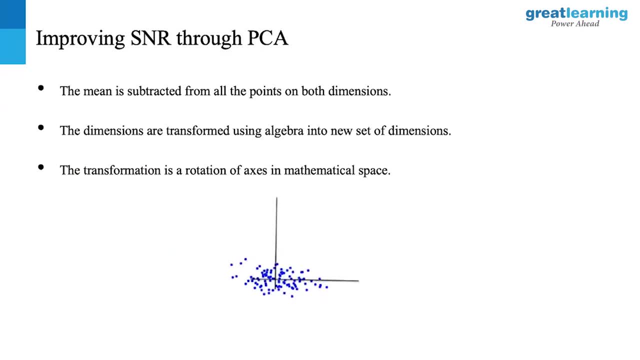 bound together, so that's called the covariance. all right, now the math behind the principal component analysis talks about calculating the zetrons, the transpose matrix. multiplying that with the identity matrix, uh, kind of a different story altogether, but in a very simple essence we're talking about placing certain set of variables on a specific principal component and facing 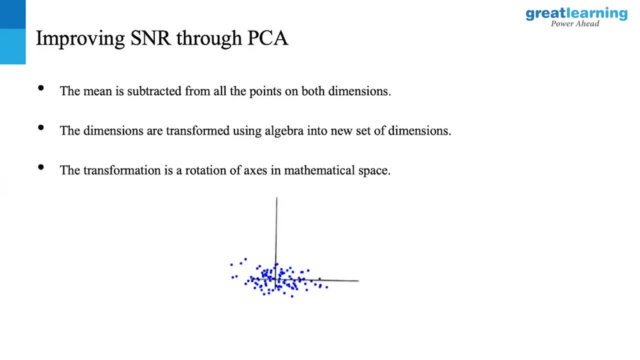 other set of variables on another principal component, and i'm going to use these components instead of using the new, instead of using the existing set of independent variables. right, and i'm going to choose this: a number of principal components i need by what we call as a 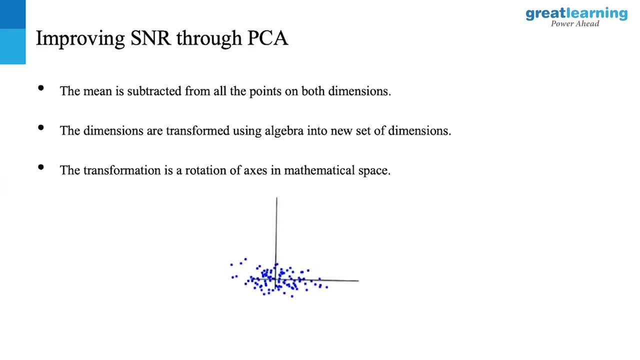 scree plot: right. so we have something called as a scree plot and i'm going to use this cree plot, that kind of. if you remember, in in k-means we had this elbow plot. it gives me, it gave me an elbow where i have to choose the number of uh clusters. similarly, in principal component analysis i have 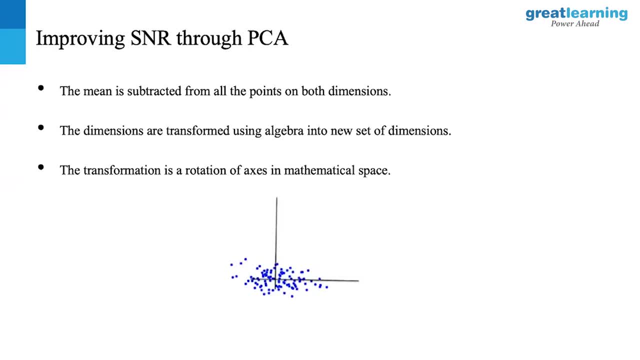 something called as a scree plot. now the scree plot is going to tell me at the elbow where i have to use to kind of get okay. this is the method i'm going to use and this is how it is going to work. the uh. this is the point at which i'm going to say the number of principal components are sufficient. 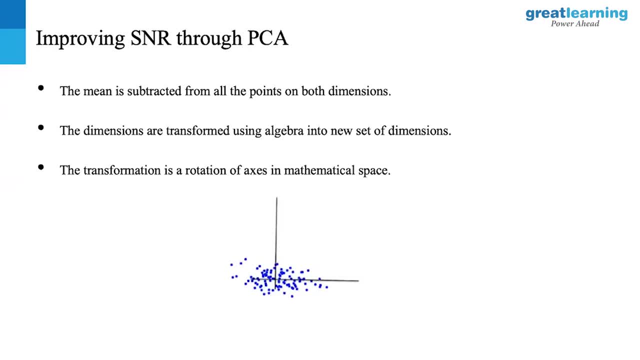 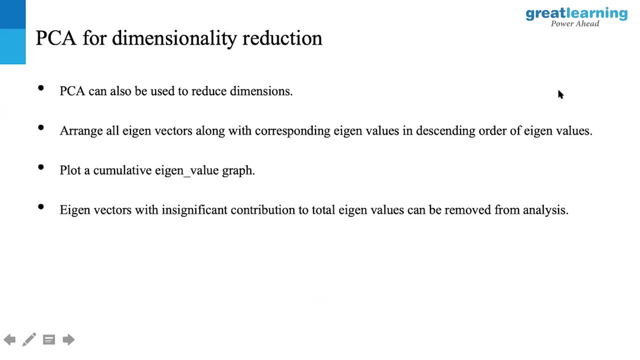 to explain the percentage of variance or the proportionality of the variance that that are these particular variables carry. i'm going to use that method to identify and say, okay, this is where i can use right. so when i arrange all eigenvectors along with corresponding eigenvalues in descending plot, a cumulative eigenvalue graph. 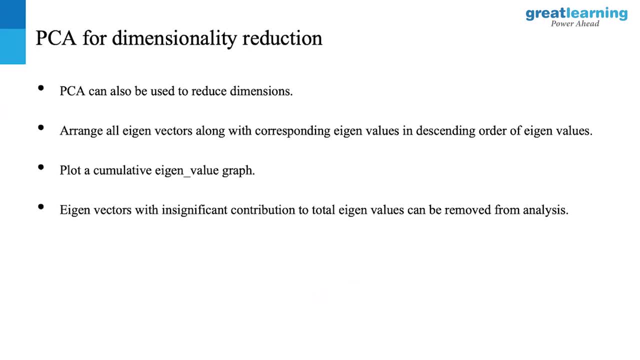 And the eigenvalue with the least insignificance can be removed from the analysis. This is what we call as a scree plan. Now you're going to find a complete elbow here, So I'm going to start with the percentage of variance. 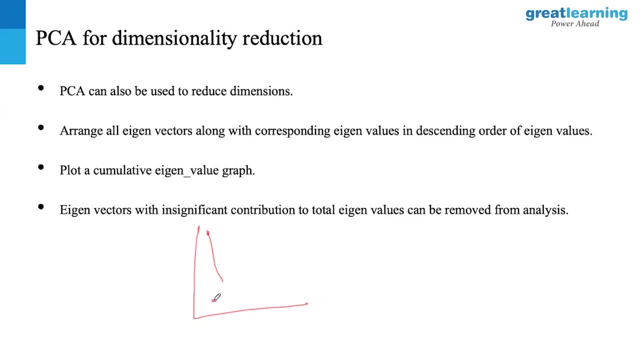 I think this graph is going to go the other way, So I'm going to start with the percentage of variance. Principal component 1 explains 90%, So it is explaining 95%. Then it goes 99.7% and so on. 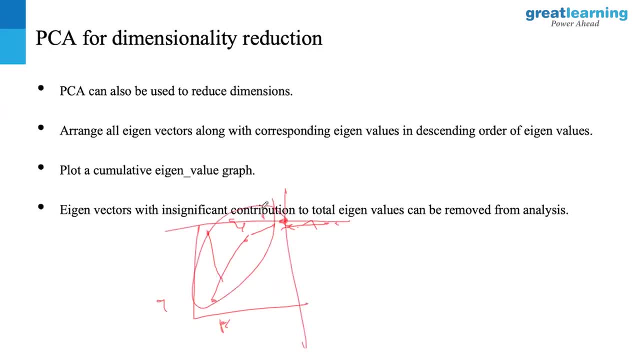 So I'm going to say, okay, these many components are enough to explain all this. I'm only going to choose n here as the number of dimensions. So number of dimensions minus 1 will be my ideal choice of principal components or maximum choice. 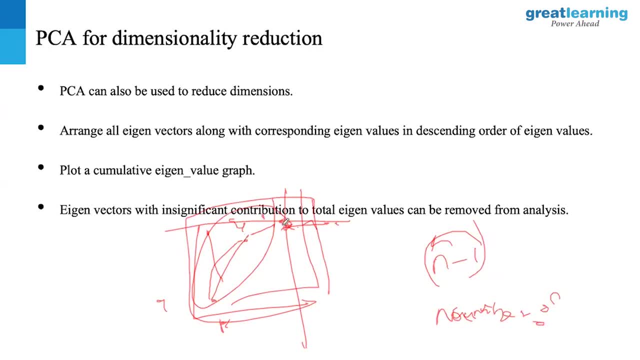 But if the scree plot is telling me that I can limit with 3 principal components, I can have 99.7% of the proportion of variance explained. I'm going to go with that. So here, the scree plot here talks about start with 1, goes, goes, goes. 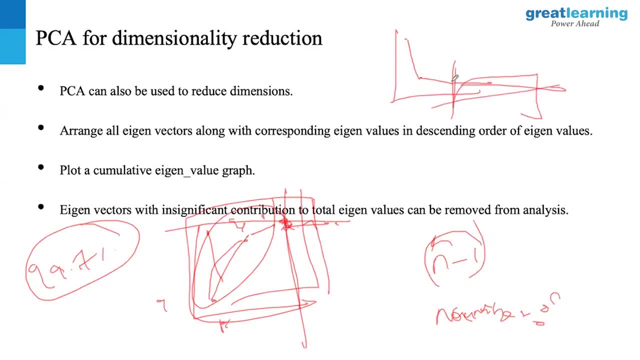 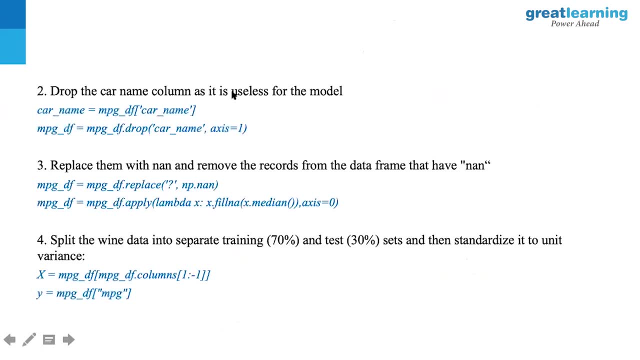 So this is the part where, beyond this, I don't need it. I'm going to discard it. I'm going to say, okay, 1,, 2, and 3 principal components are sufficient, All right. So this is what we have for the PCA. 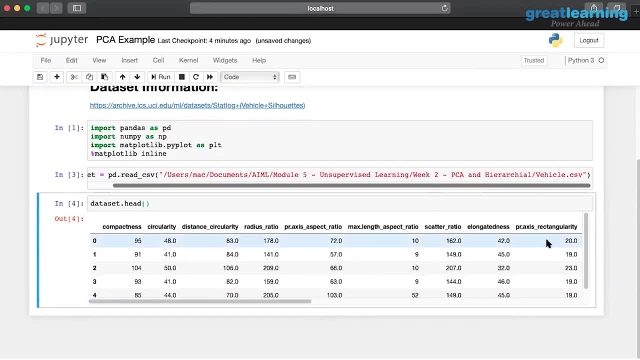 This is the data I have, So my objective is to classify it based on the silloud data. So from the silloud we have different information about scaled radius of grayish gyrations, keyness about it, The hollow ratio, the class, whether it doesn't belong to a car, van, bus or whatever it is. 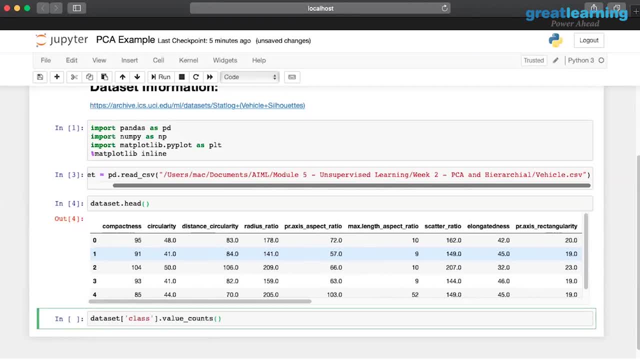 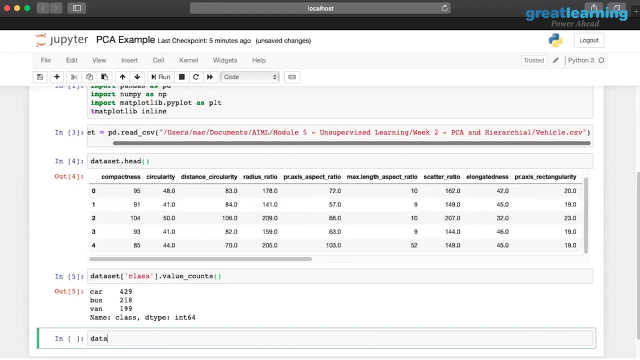 So if I say this is about so, this is what I'm essentially going to tag into a car, bus or a van. Now, if I look at this, I'm going to say this as well, I'm going to add this attribute as well. 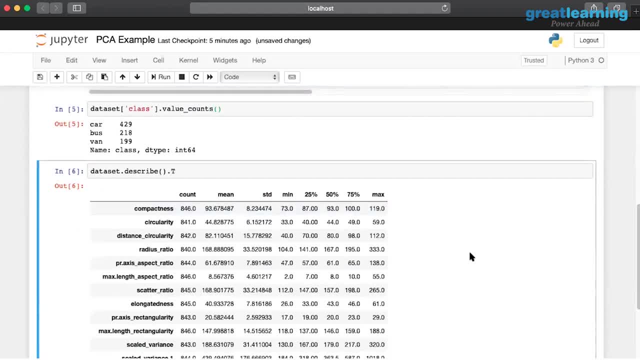 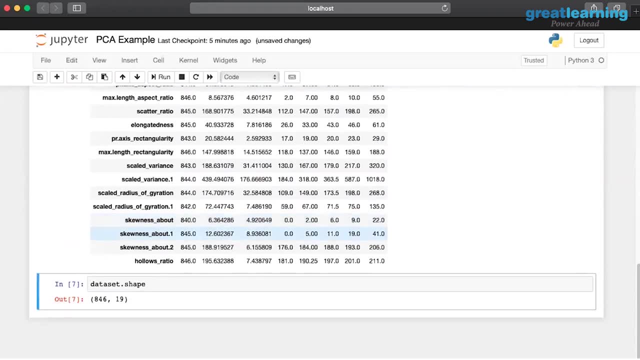 Let's now describe the data All right. So we have quite a lot of features. We're going to say shape, Identify, features. We have 19 features And we have 847 inputs. that we have All right. Now what are the types that we have? 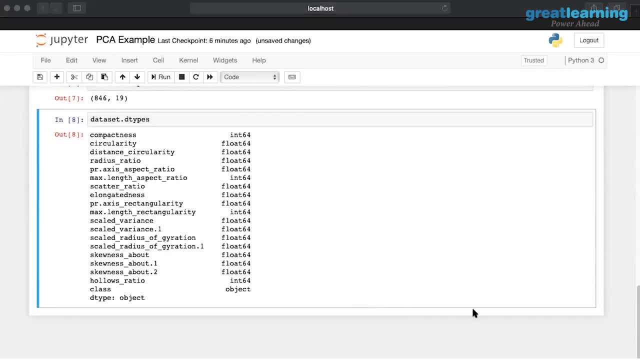 Barring class, everything else is either an int or a float object. I'm just going to talk about a very simple aspect. So it's going to talk about a number of records I have in each bus, car or van. We already looked at the class value counts. 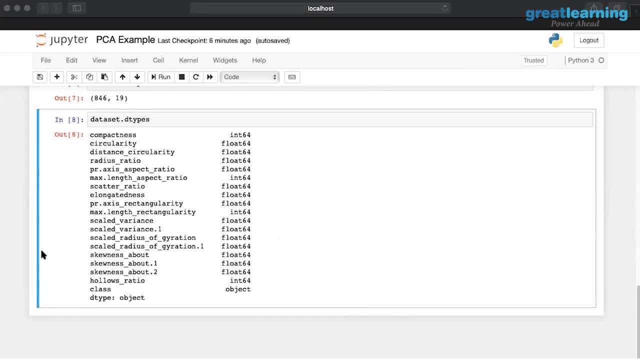 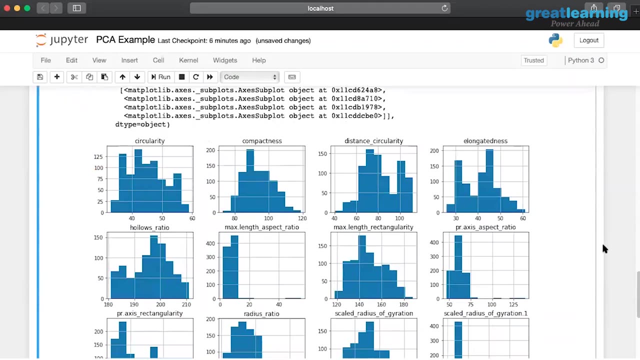 It says how it depends on the work. What I'm going to do is just do a Very simple, maybe histograms to look at and say, okay, this is what I want to visualize, All right. So I'm just going to look at a very few simple visualizations and look at them to see, okay, how's the data distributed? 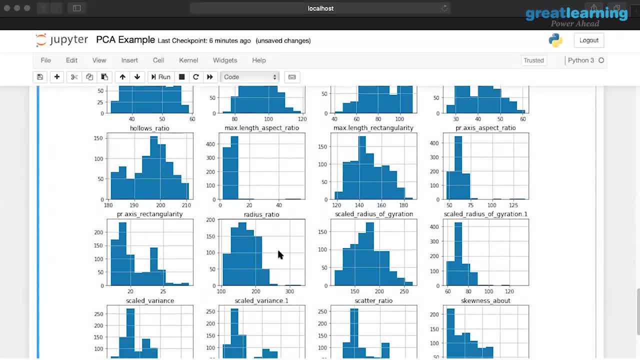 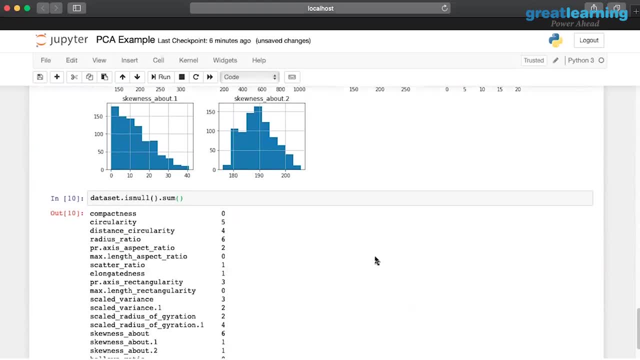 What's the kind of skew the data has, And the reason I'm coming up with this is I want to find out if there are variables that are correlated to each other. I want to first understand the data. Now, if I talk about it, this data has missing values. 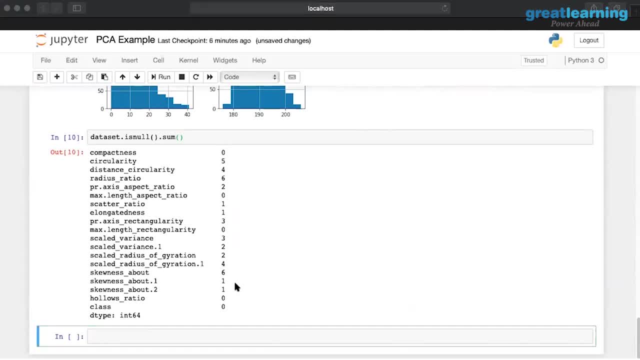 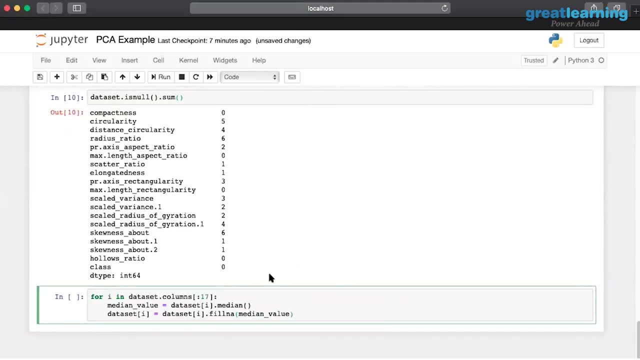 The data definitely. The data definitely has missing values And I am going to treat the missing values by using the median imputation. I'm going to take the median value and I'm going to impute the data and say, okay, the reason I'm going from for up to till 17 is nothing but the 18th column is your. 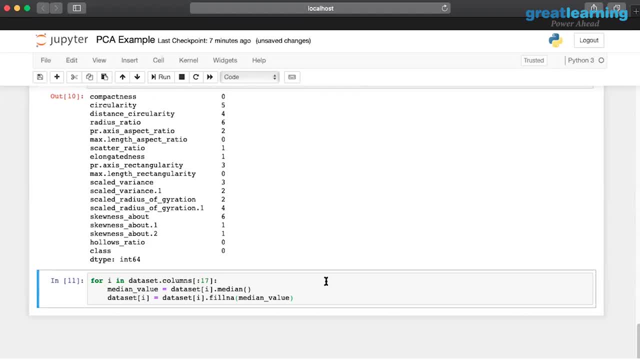 The value of 18 here is your class. If I have 0 to 17,, it basically means from 0 to 17,, which is still hollow ratio. So if it has a missing value, if I'm going to talk about a null value, 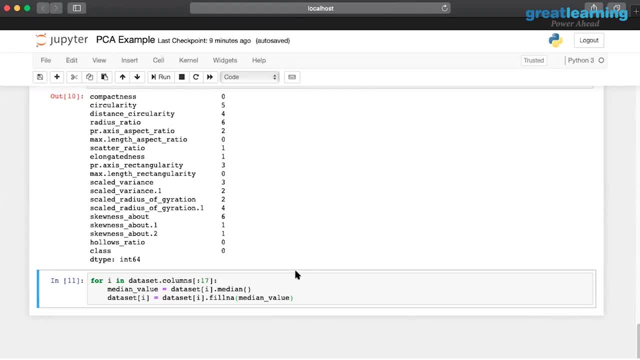 I'm going to talk about a missing imputation. So here I'm imputing with the median value. Now I'm going to. It's going to talk about no missing values. So once I don't have a missing value, I am going to first plot a point. 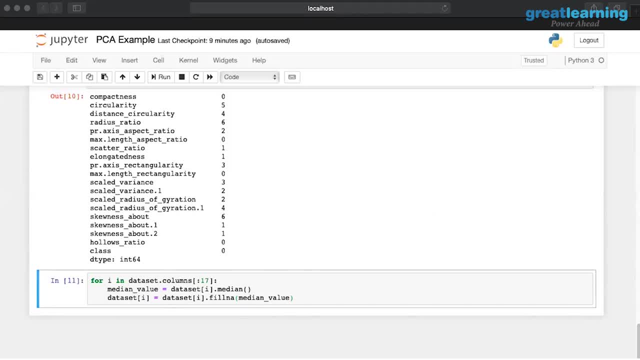 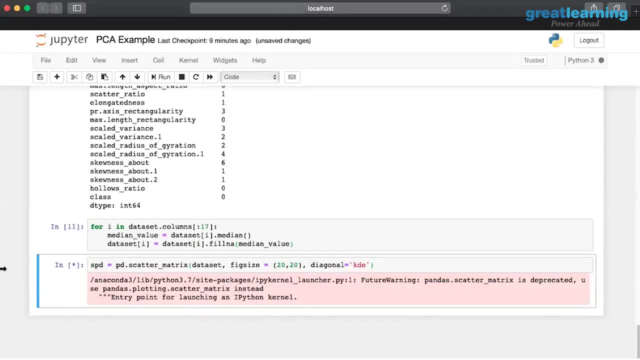 I'm going to just look at how the data is set up for each other. That's going to tell me some kind of an interesting perspective here. Now, if you notice, if you notice this particular scatter matrix, it's going to give you an interesting look. 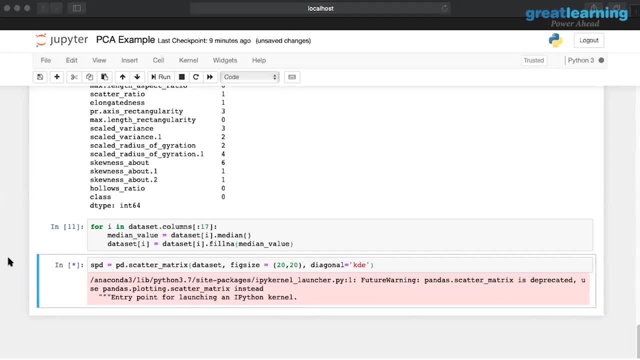 I can either do a scatter matrix or I can also do a pair plot. Either way, this is what I'm going to get, But, if you notice, I'm going to draw your attention to the fact that almost all the features are going to be correlated to each other. 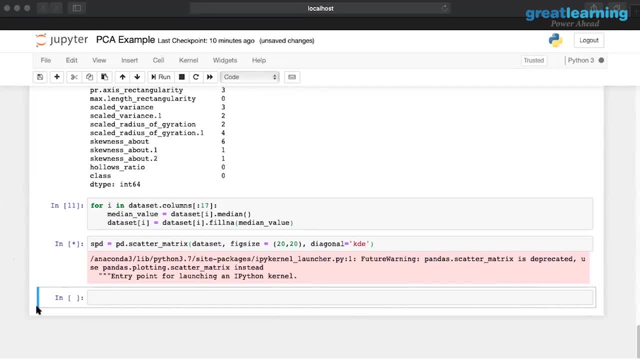 That's something that you're always going to see and that's going to be an interesting look to have as well. Tell me you said on the WhatsApp. you said that missing pi is one of the libraries Right Which we use. What are the other ones which are available? 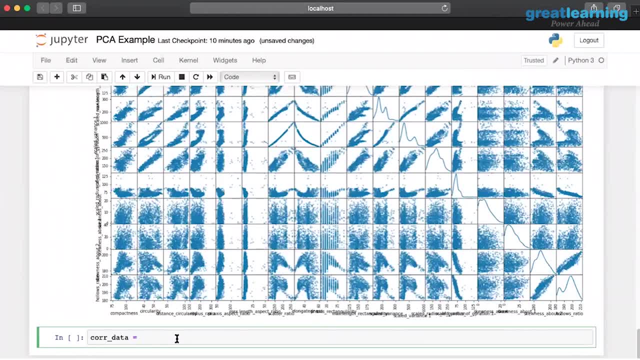 I don't remember that off the top of my head, Nitin. I can share the link with all of you on the group as well. I'll put it up on the chat. Sure, Because I just checked. the missing pi, I think, takes out the first column with the minimum missing values. 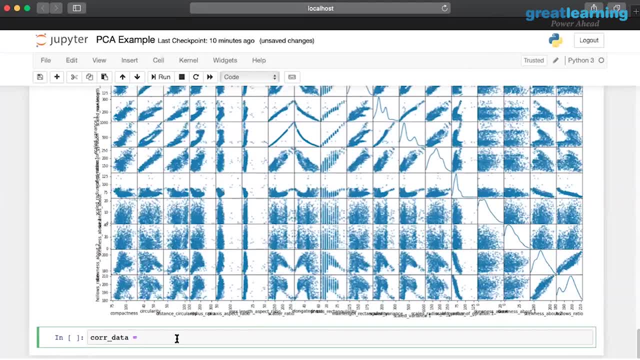 And first it fills with the mean and then it uses the random for a stop on the top of it. Yeah, So the reason is the random. Any values cannot be handled. So Python does not handle any value as it is, as an object. 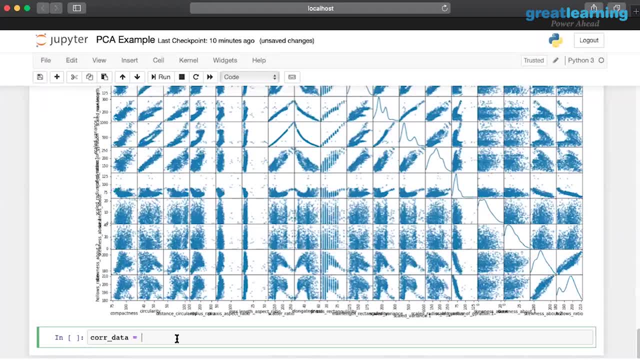 It kind of takes some effort on that context So it fills a mean. then it runs the random forest imputation. I'll look into the algorithm, probably share more insights about it to you, But right now, yeah, that's essentially how it goes. 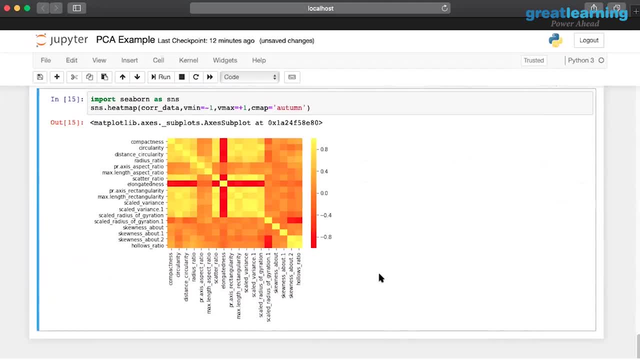 So you kind of will find this specific aspect here. Remember I told you there is a big amount of correlation to almost all the independent features, to itself. If you notice, that's a no-go for some of our algorithms And that's something that we have to be worried about. 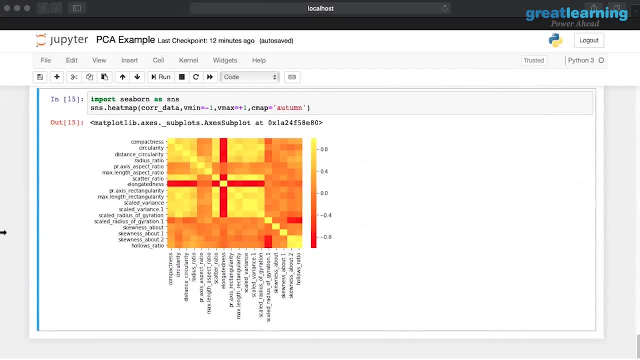 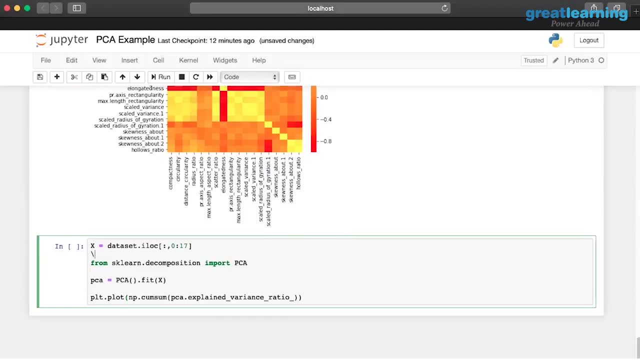 So replacing Using a dimensional detection technique here would be the most appropriate solution to solve this specific problem. Right, All right. So here we're going to implement the PCA, We're going to take fit and we're going to just plot the implementation. 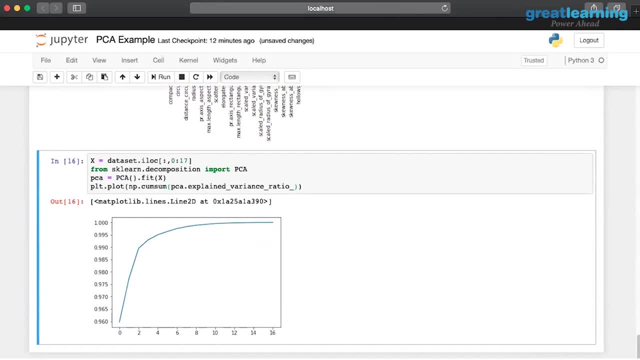 So now, if you look at it right, if you draw your attention to the screen here, you will find that at 10, you have the highest ideal explanation. So at A6, you have what? for six principal components you have 99.5%. 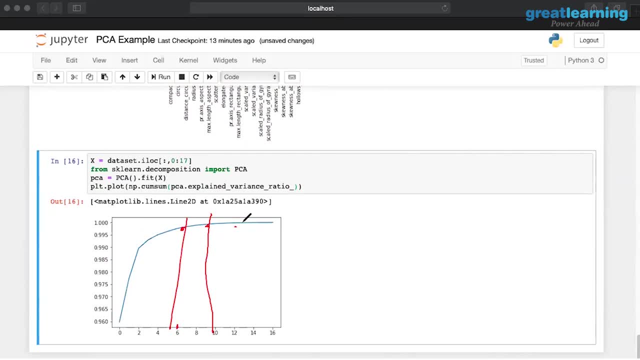 At 10,, you have 99.7% And 12,, you have a lot more. So you can just print it also and see how it works. But that's the idea. So when you run this cumulative sum with the principal component, analysis explained variance ratio. 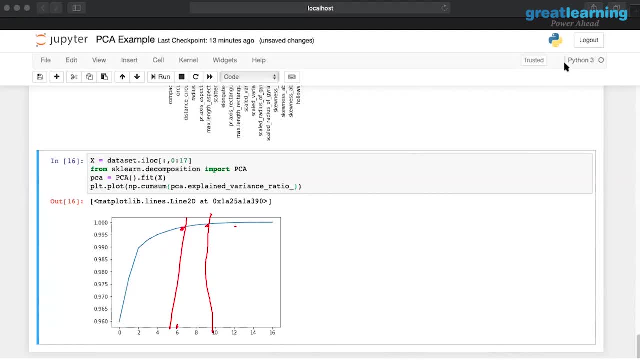 you will find how many number of principal components are required to replace the 19 variables. Ideally. here the PCA is telling me that I have 10 variables And I want to replace it by. And if I replace it with 10, I am getting about what 99.7% of the original information retained. 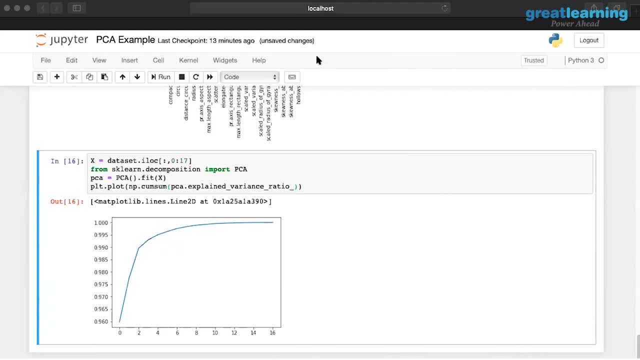 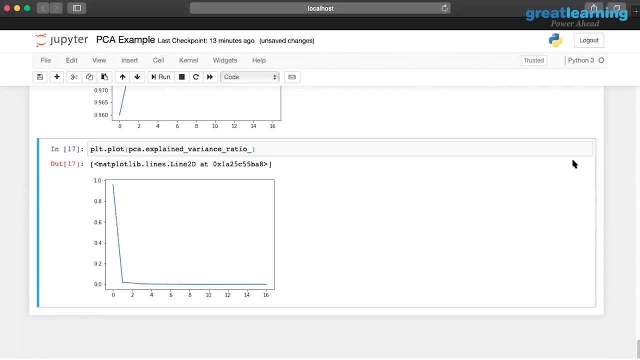 And I'm going to use that. So that's the ideal way of looking at this. If I don't use the cumulative sum, it's just nothing. but the ideal is going to be a scree plot. So this is what we call as a scree plot. 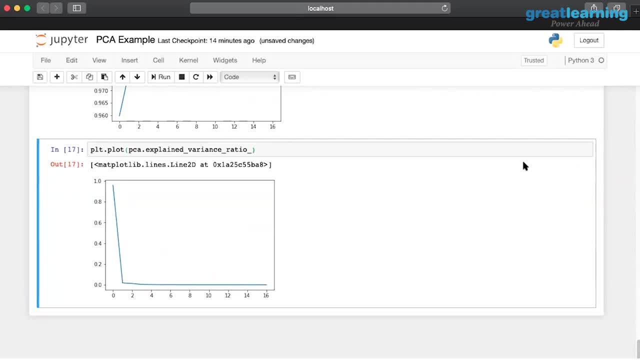 So either you can use a scree plot or the cumulative variance ratio. So with this right, with the scree plot, what you're going to identify is where do I cut it off With the? So you hear it says two or three is the ideal solution. 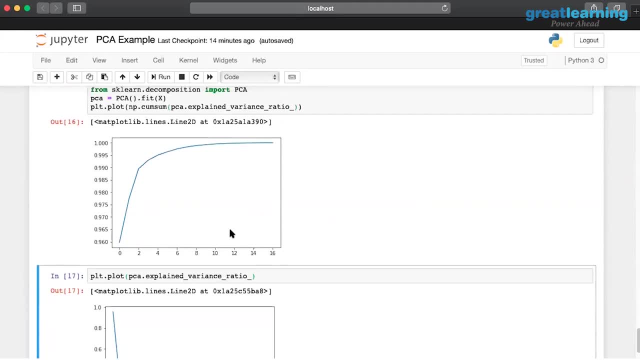 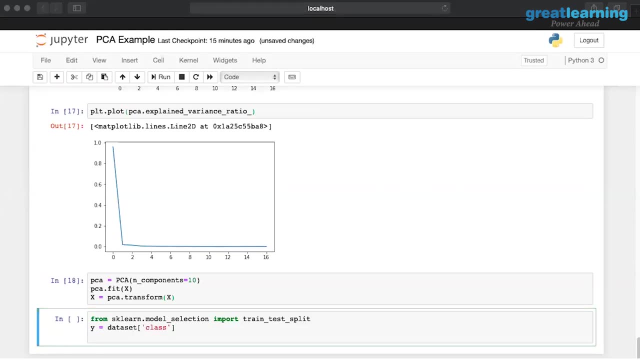 But in essentially with the cumulative variance explained ratio. here I'm saying that okay, 99.7% is ideal. So I'm going to go with 10 principal components. Can you just explain this again? Difference between the two. 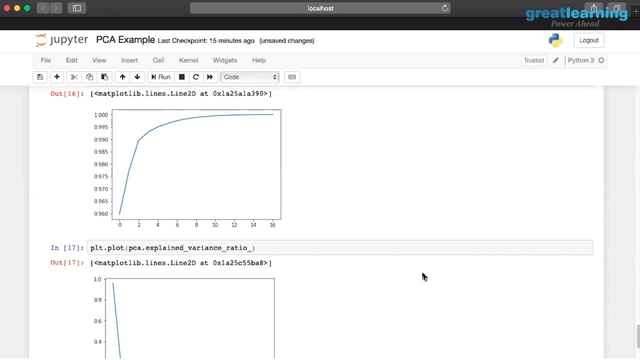 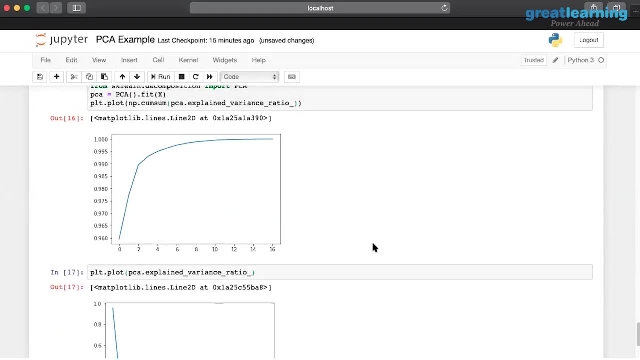 Yeah, So here, the number of what you're going to look at is the scale is minute, So you're not going to be able to understand the difference here, But ideally, the objective that you're going to look at, right. 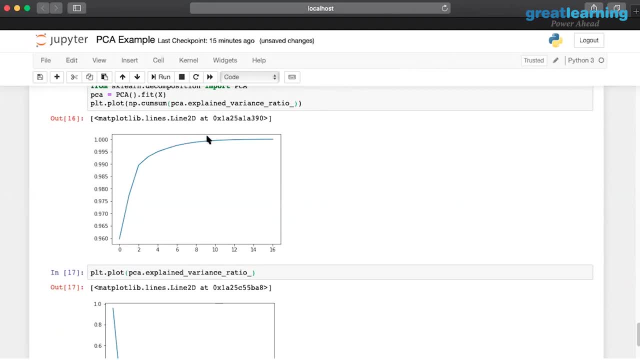 The ideal objective that you're going to look at is to have the highest degrees of principal, highest degrees of variance, explained with the lowest number of principal components. So here I say 10 is good, If you notice, with two components I'm only able to explain 99%. 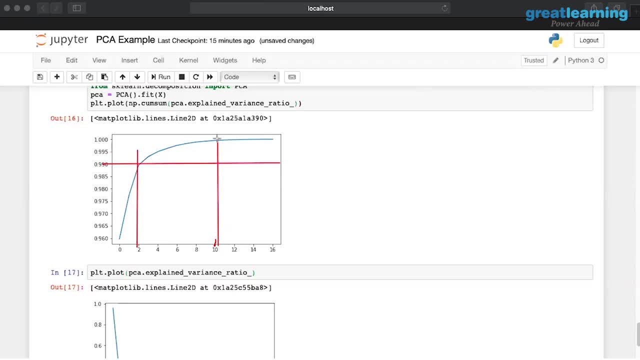 So the 99% I have here Now with this I'm going to talk about 99.7%. So ideally I'm saying that, okay, 99.7% of the variance is captured with 10 principal components. 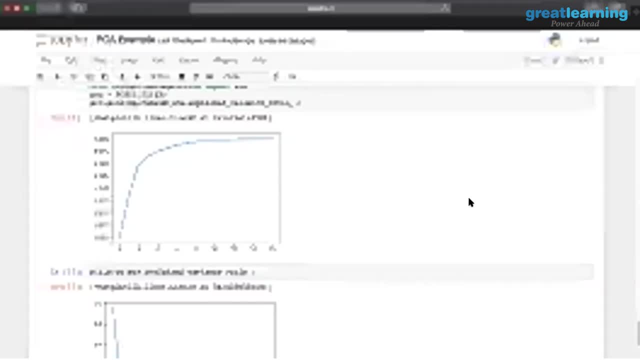 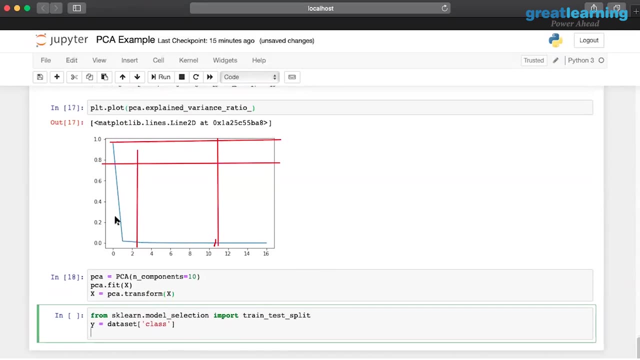 If I talk just about the scree plot. the scree plot is what we use here to say, okay, the number of principal components that require that are required, right. So remember we talked about the eigenvalues to sort and say beyond which I'm going to discard the number of components. 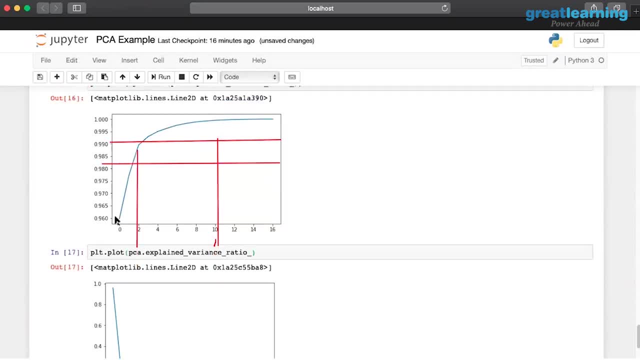 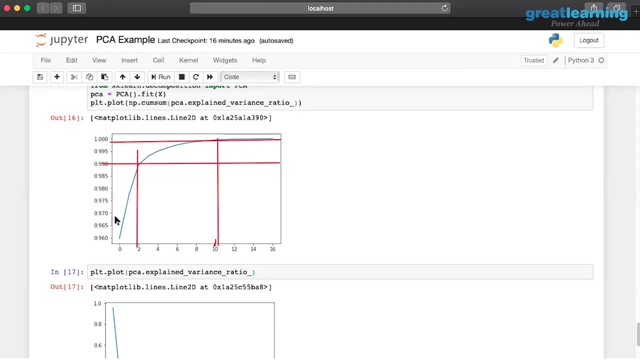 This is the discarding of the components. This is used to discard the components and this is used to identify the ideal number of components that you want to use. That has the highest variance ratio explained. You're not going to be able to use one without the other. 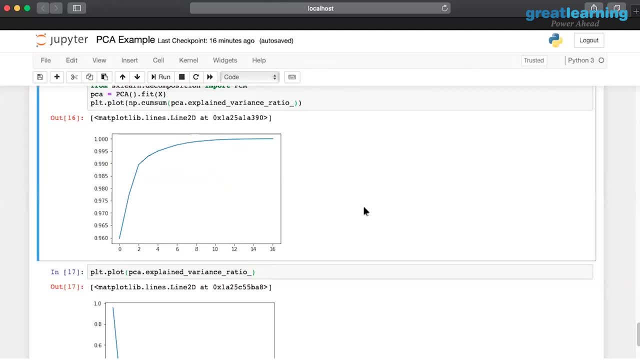 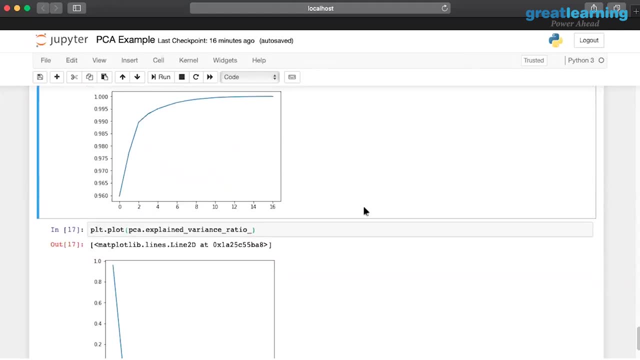 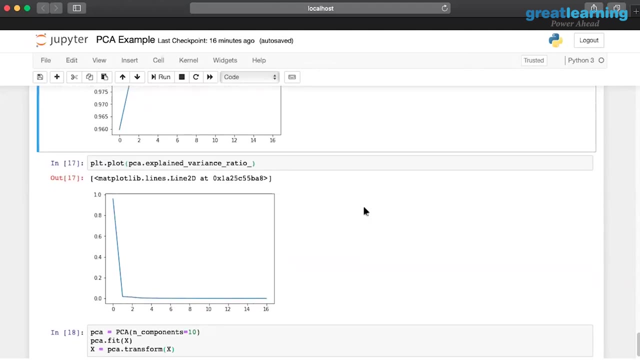 Does that clear the question? Yes, One more thing. Through PCN, we have already converted the variables into a Gaussian variable and independent of each other. Correct. So now why do we want to remove any of the components and lose information, even if it is 0.01%? 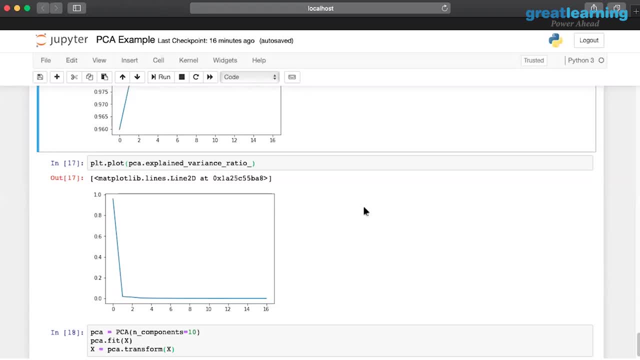 Okay, that's a fair question, right? So the reason we don't go with all the principal components: If I take and load my entire set of principal components, or the axes, what you are going to get right is the exact data set, is the exact variable of the data set coming back into you? 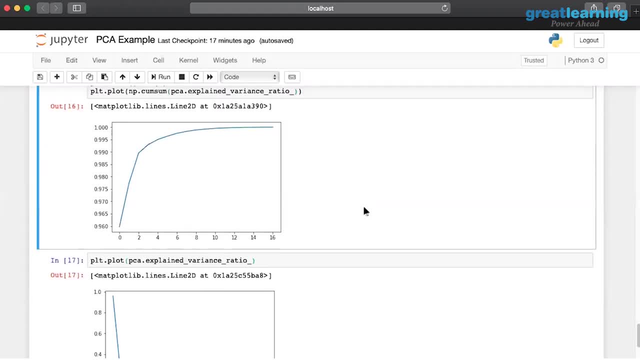 So you want to select or give up this cutoff point that says, okay, I have the maximum variance explained. No, just because I'm transforming it. if I reuse all the variables again, I am going to end up with the same data set over, which kind of defeats the objective that I have with the principal components. 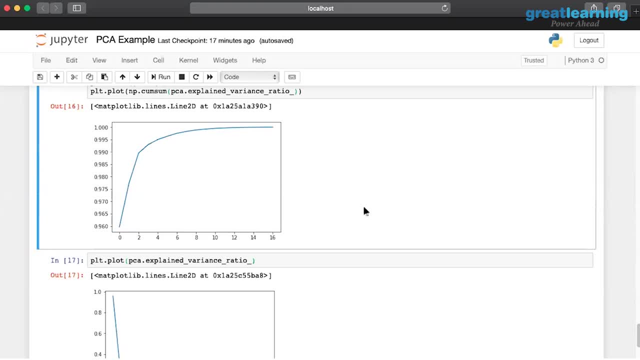 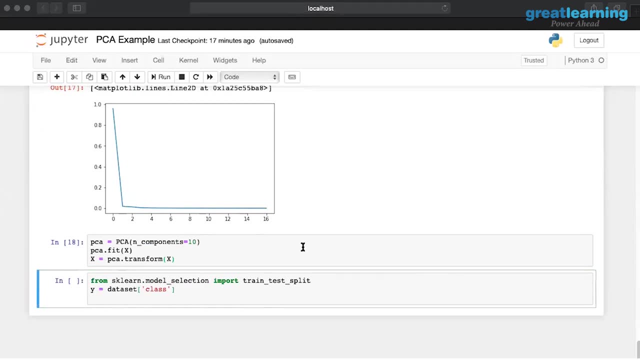 Does that answer your question? Yes, If I suppose we don't remove components over here, just in case, understand that it will give me back the same data set, Right? So if I don't remove over here and suppose, after that suppose, can I use a linear regression model after this: 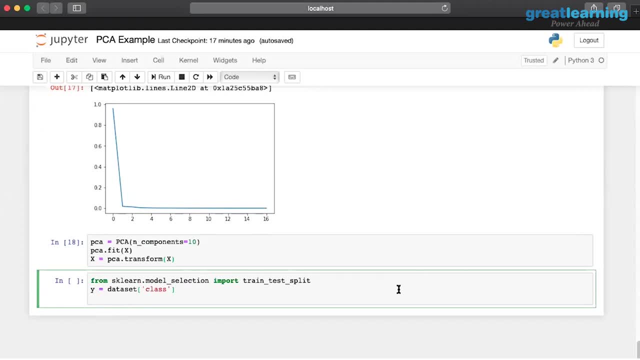 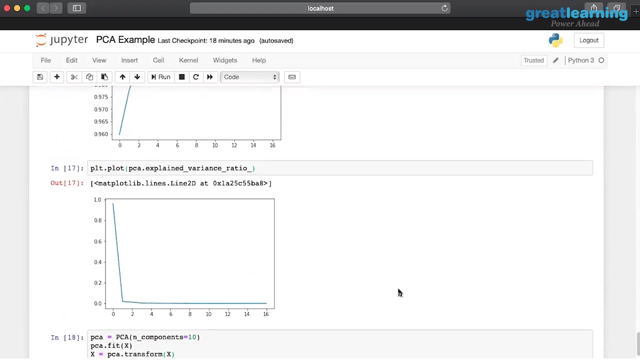 Yes, you can. So if I use a linear regression model, there's an AIC and the BIC values which Correct, So won't it help in that case, As in using all the components? Yes, So won't AIC and the, because it rates on the best model fit with the least values. 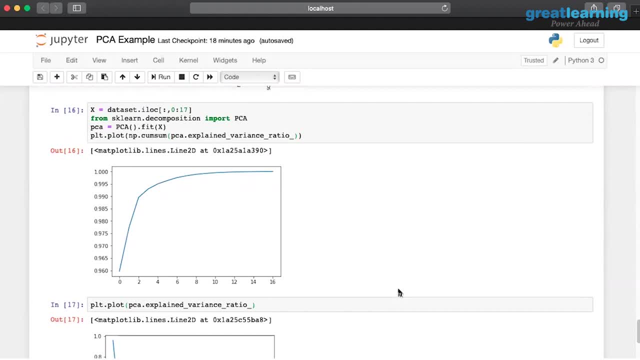 Okay. So when you're using a stepwise regression, you're going to choose the ideal features, right? So there is where the AIC will have a major play. So when you're taking a stepwise regression, we say, okay, the step is basically: 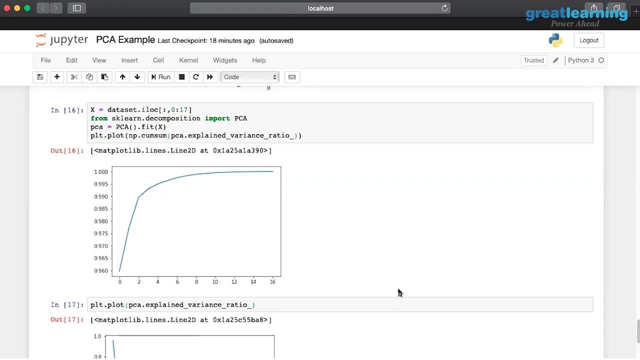 So you're iterating to add or remove variables. You want to do a forward selection or a backward elimination. You want to drop or add variables based on the information value that it kind of carries. So AIC being the lowest is what we'll choose. 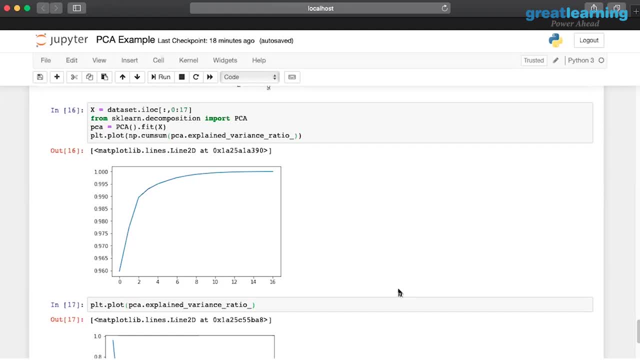 Now the variable within it that has the highest AIC, that kind of inflates the AIC, will be dropped. That's a stepwise regression concept. Now, if you're going to use this data set right, I'm going to say I want only 10 components and I'm going to fit this out. 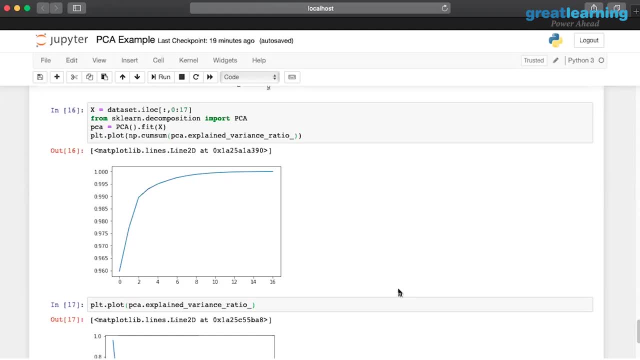 So your question that says: Why don't I use all 10 to let the model choose the best set of features, correct, Ideally, that will not be the correct solution here, Given that we just kind of went through the basic ideas. 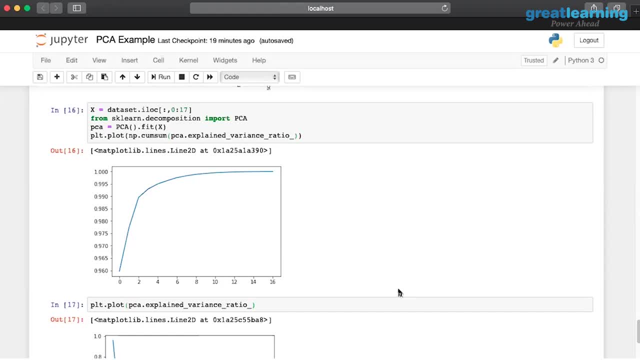 I want to use the ideal number of components. If you understand the math behind it, it's just basically transforming the data. The principal component, analysis, is kind of setting up data and transforming them into different axes. Now, if that is the case, right, I'm going to transform a data. 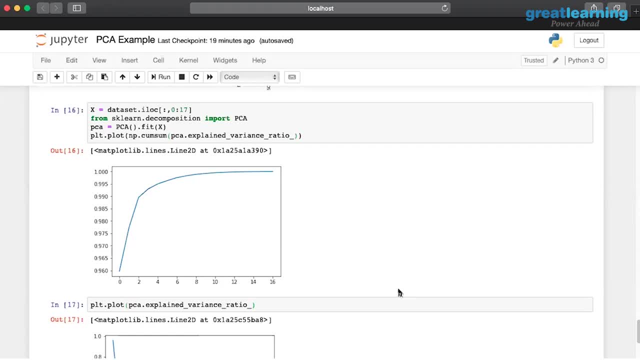 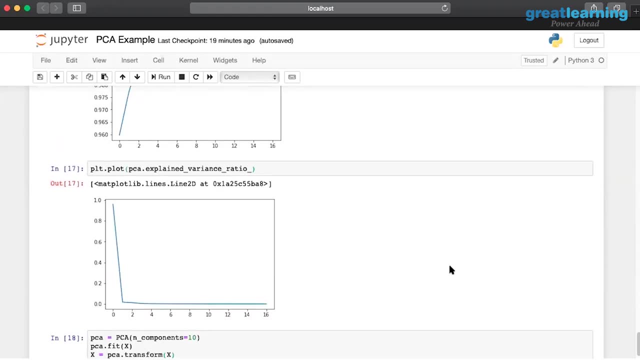 And I'm going to use it in the model and let the model choose the ideal selection. That will not make a more relatively rational sense context, Because your model selection, the feature selection, you can't just rely on AIC. We are removing the multicollinearity between features, transforming the variable into a different dimension set. 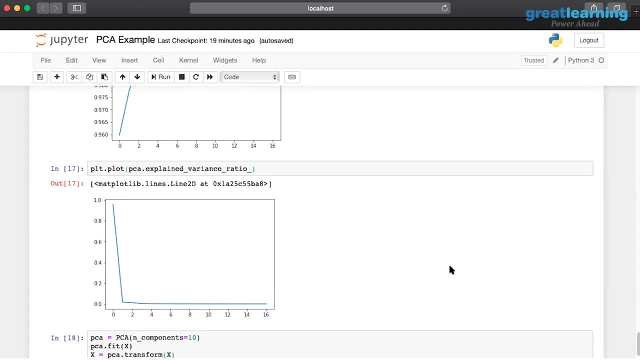 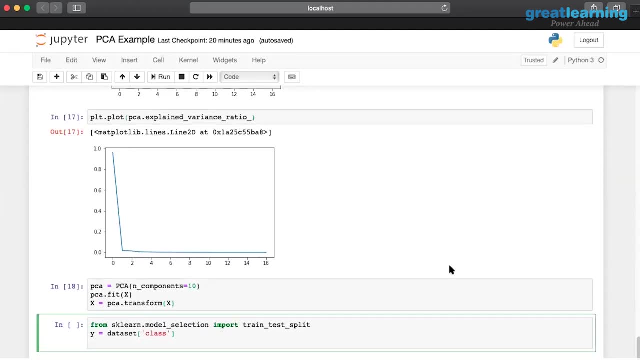 and then using that aspect So that, ideally, is not going to be a job that you're going to leave completely up to the linear regression, I'm going to use the PCA to say, okay, this makes, This does not make sense, this does not. 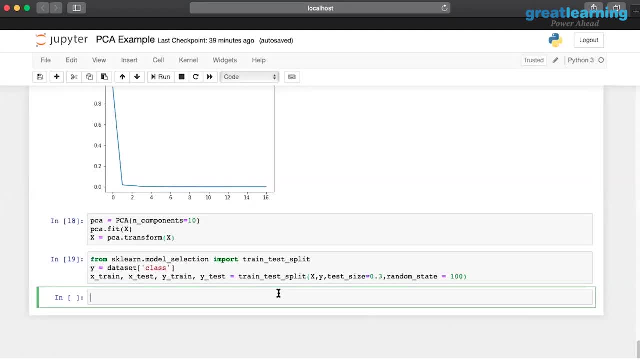 So that's how I'm going to limit it and go by. What I'm going to introduce you to is a method that we call as the grid search method. Now, the grid search is to help me identify the best set of optimal hyperparameters. 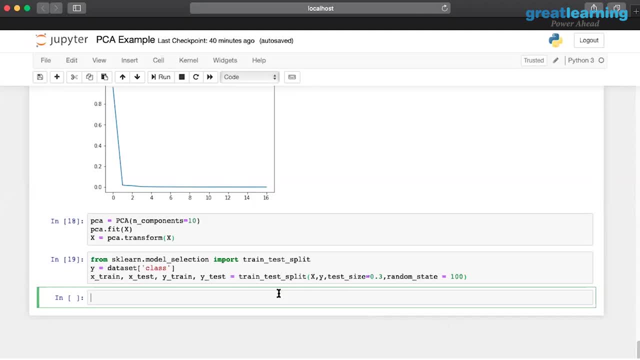 Now, this is not particularly to the feature engineering part, but this is to help you build a better model. Now, this is also a way of finding the ideal solution, or the algorithm essentially is used, which, whenever I'm using an algorithm, I'm going to find the best possible hyperparameters of this algorithm. 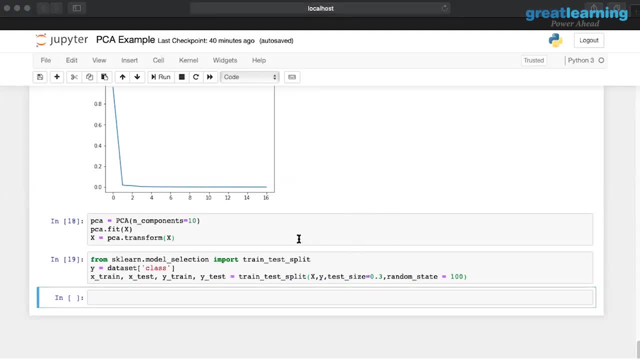 Now, given that, let's say, I want to import my support vector machines, Now what I'm also going to import and fit this model. So I'm going to say: grid underscore params equal to Now. this is what I have. 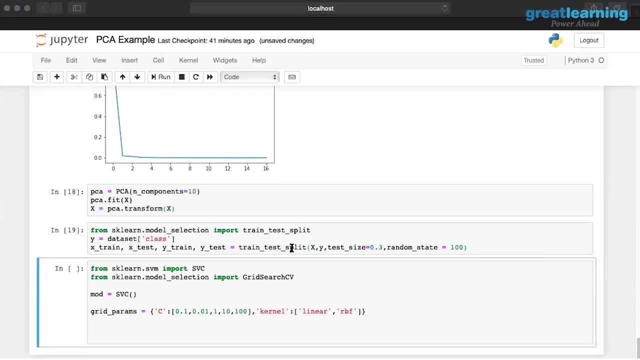 So, using this, I'm now going to create a grid search model right now. Okay, What does this stand for? 0.10.. Okay, Remember, the cost is near. No, no, not that value. My question is: are we searching only on these values? 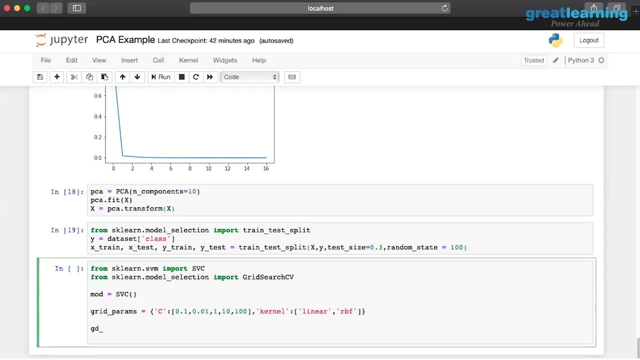 Yes, we are iterating over these values to get the best possible result from this sort of a grid search, But then again we are not taking into account every value. So how do we know that these are the only values that fit the best model? 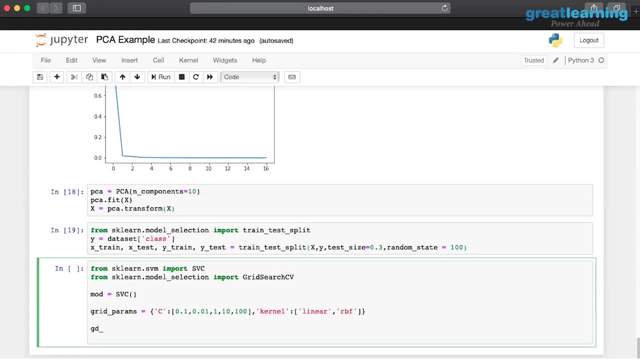 Okay, So basically it is about exploration. So this grid search when you're talking about it, right? So the objective here? So the objective here is, I am going to try, among all these values for the model, as an input to the model. 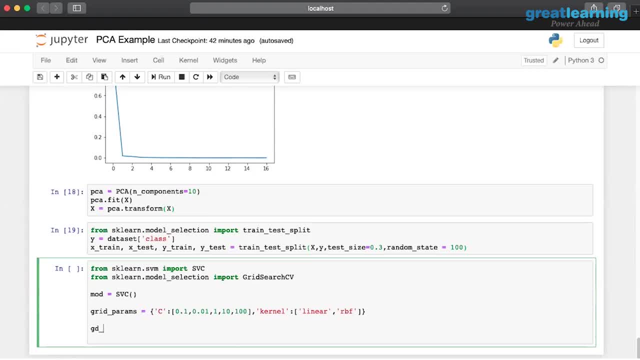 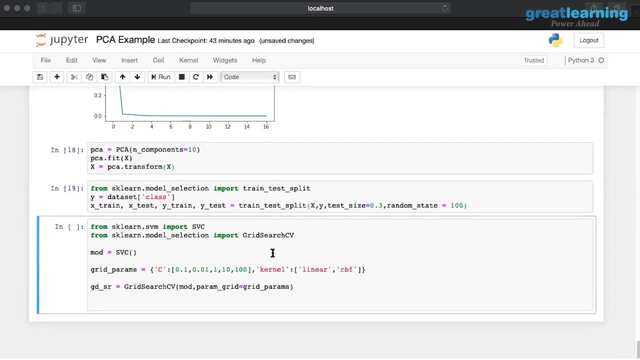 And that's going to come back and say: this algorithm, this particular result, has the best solution possible. So that's how it's going to essentially work. Okay, If you want to print the entire grid results, you can always do that by making verbose equal to 5.. 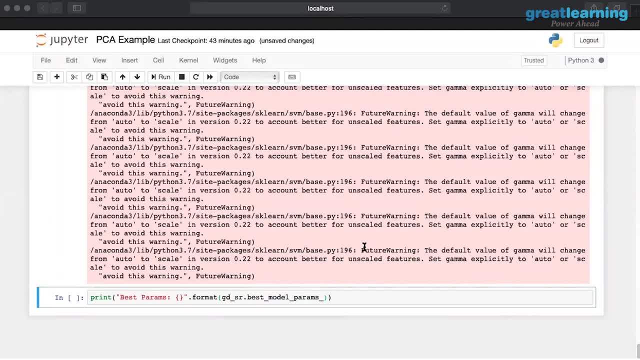 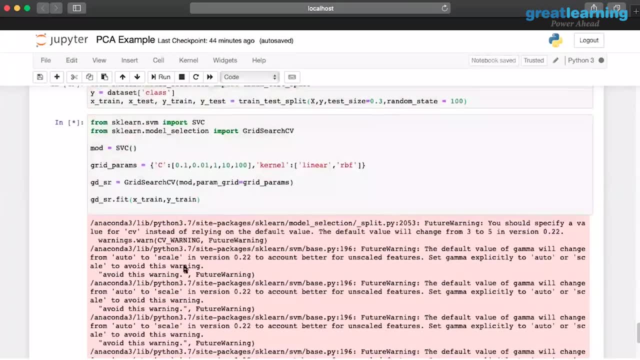 That will print it. I can print the best model. Gamma was also part of this, Yeah, So just an example here. Nitin, I'm just setting up an example that shows what are the ones that you can optimize. So if you take random forest, you have a lot more parameters. 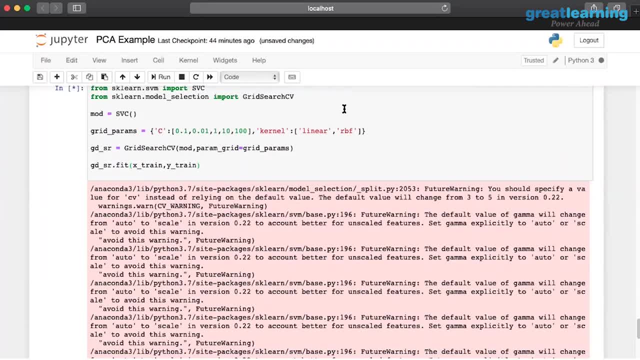 You have min depth, max depth, You have this criterion, You have the bootstrapping, So you can choose any one of these parameters. This is just a showcase to see how do you do a grid search per se. Gamma is also a factor that will affect. 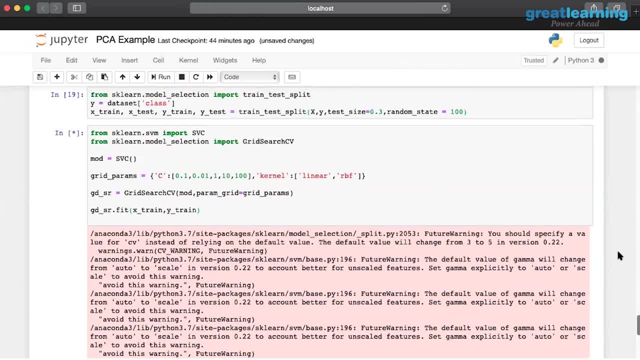 Yes, definitely. it will affect my RBF more than my linear, So the gamma can also be used. If you want to change or tweak the parameters, yes, you can. This is just to show you how to work around with it. 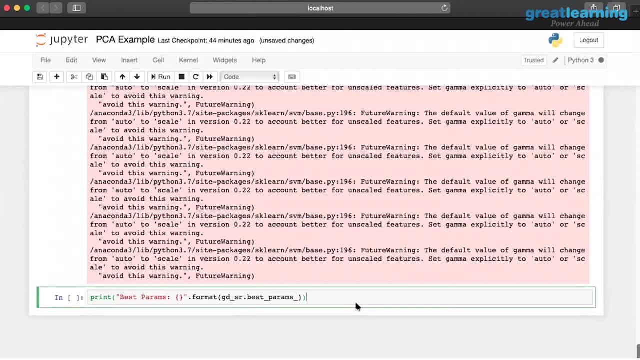 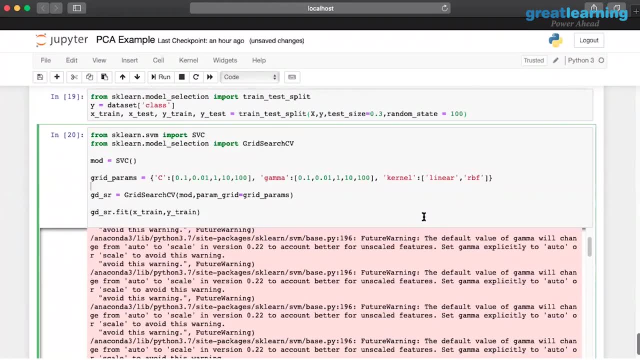 So, if it is not, can you use gamma also in slides, just to know how to go about it? Can you explain the grid patterns once again? Okay, Yeah, 0.1, 0.01, what is this? Okay. 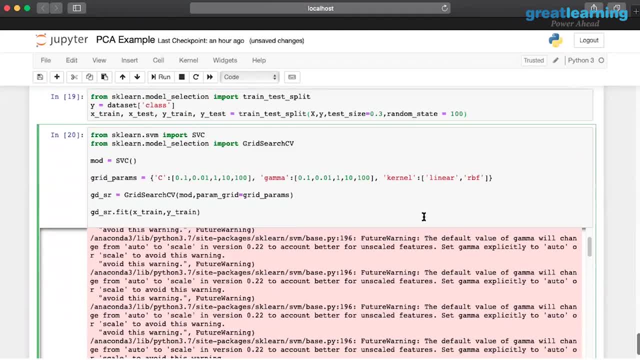 So it's basically for, if you know, if you understand that we have this support vector machines right. So in support vector machines you have three parameters that we can tweak. One is your cost parameter or C, which will give you either a soft margin classifier or a hard margin classifier. 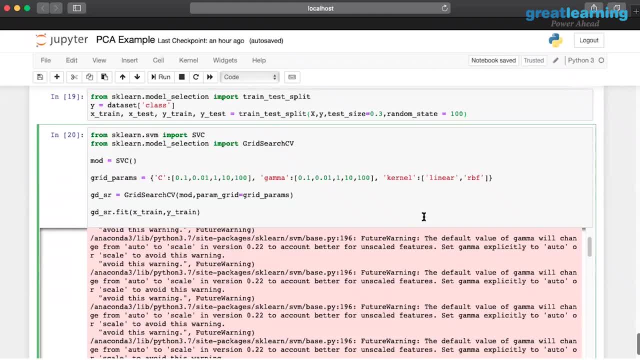 The other factor is what we call as gamma. That's basically how much of your kernel does it fit over fit or under fit your current curve? And then we have the linear and then we have the kernel type. So if you have linear, radial, RBF and polynomial, 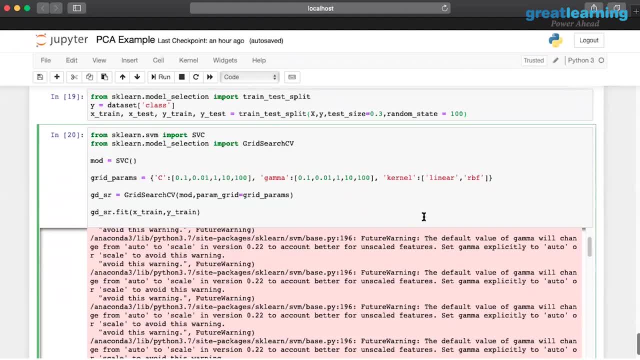 So what I am trying to do is now, what will happen right now is the fact that it will try for 0.1, 0.1 and linear, 0.1, 0.01 and linear again. So it will try, for it will do a permutation combination of all these parameters to the final algorithm. 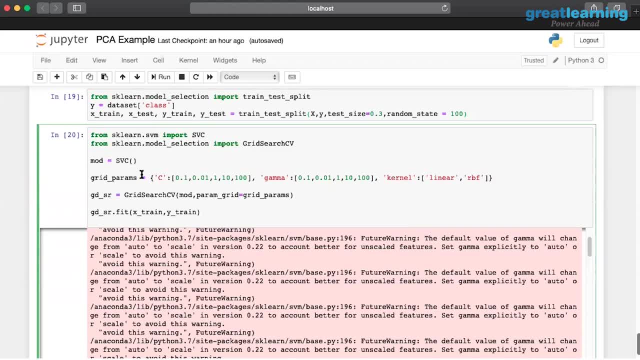 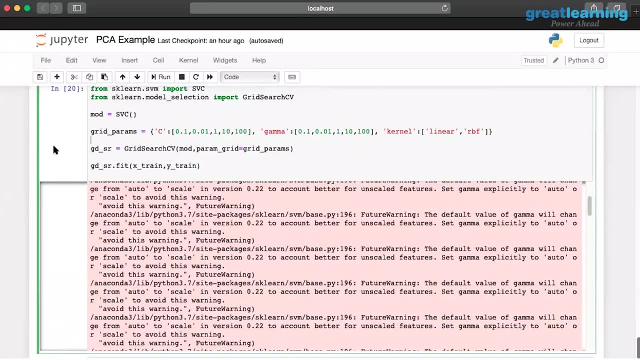 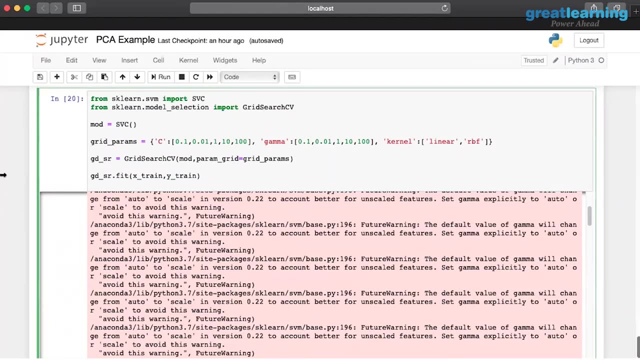 Okay, So it will try all the combination of all these algorithms and come up with the final model that has the best result in terms of accuracy and score. But somehow this again is kind of a manual intervention over there, Right? So ideally it's up to us to some point to say: 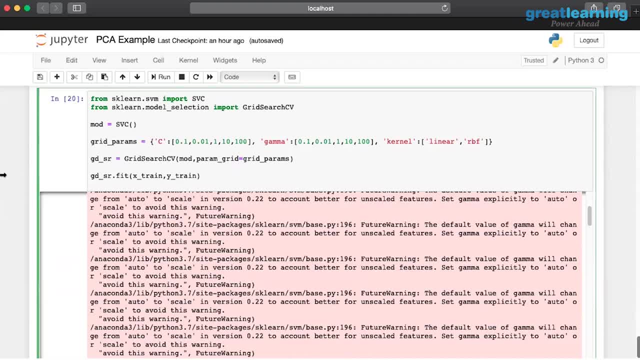 okay. the other option that you can do for SVM is you can go from 0.01 all the way up to 100 between increasing values in 0.1. So you can always do a step in that manner. So that's going to take quite a bit of time to run. 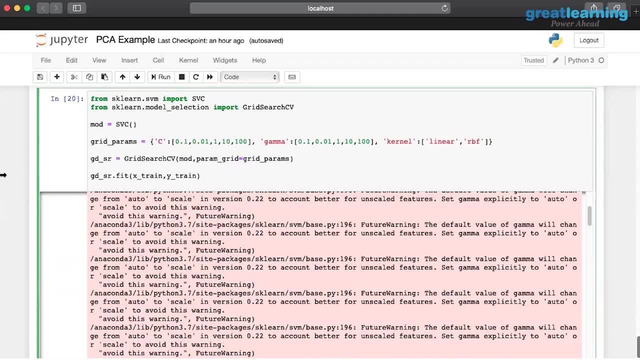 but ideally we kind of set benchmark values and we go about it. This may not try for every possible value there, So if you try, if you look at that, you will have 0.1, 0.01, 0.05, 0.03.. 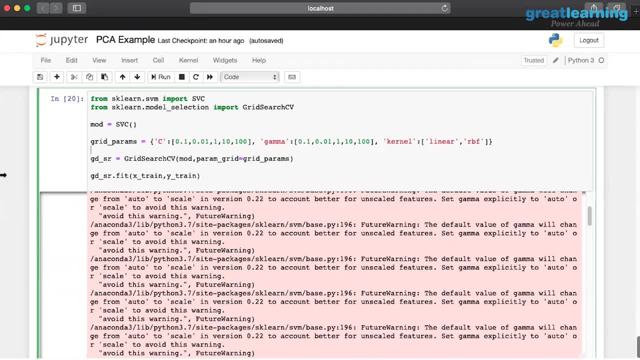 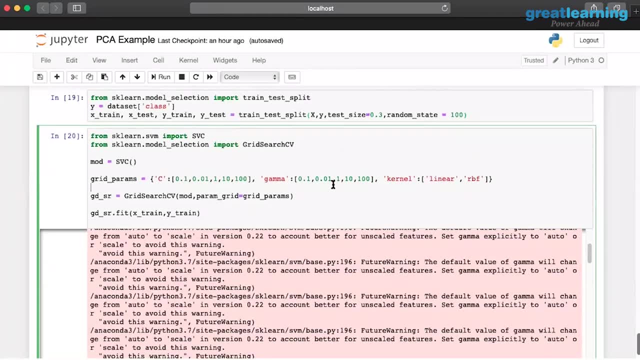 So you have multiple values that can ideally change your equation. So it is up to the user to see if you want to try it at that level, at that granularity. So this I might not run this out right now, but if you run this you'll understand this. 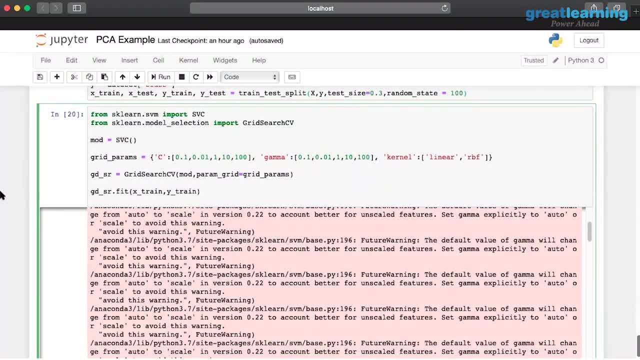 It's going to take quite a bit of time because it has to run. I don't know if my machine can support this high intensity, but yeah, the idea is, if I run all these combinations, it will take some time for the model to execute. 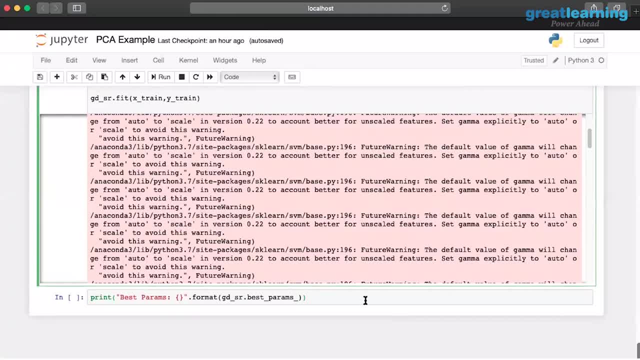 and then they come back with results And once you have, you print the best parameters by saying that, okay, this is the best parameter. This is what I'm going to finally build my model upon, And that's how it's going to essentially work. 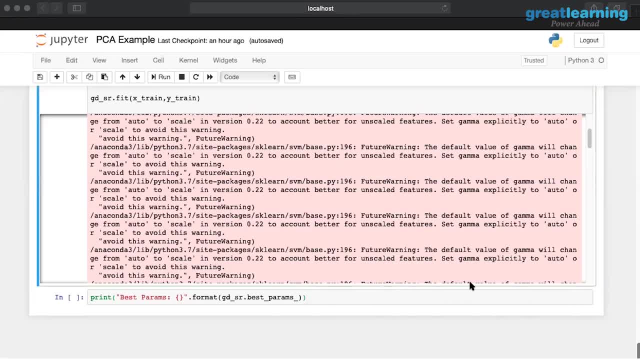 All right. You'll also have this cross validation score where you're going to create a careful cross validation and you're going to find the best cross. You're going to see if the cross validation is actually helping you do a better job in this context. 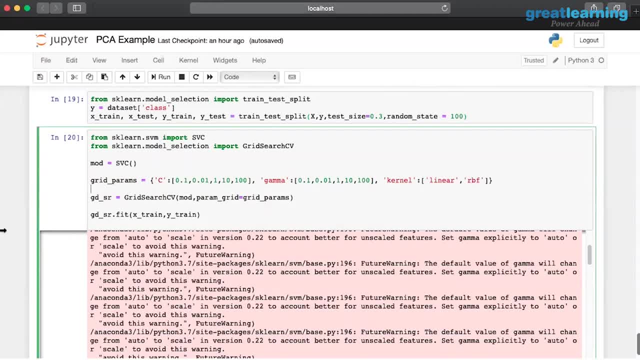 Okay, So if I start running this right now, it's going to turn for quite a bit of time. If you want, you can remove some of Sorry C values, If you can just see it. Sure, sure, sure. 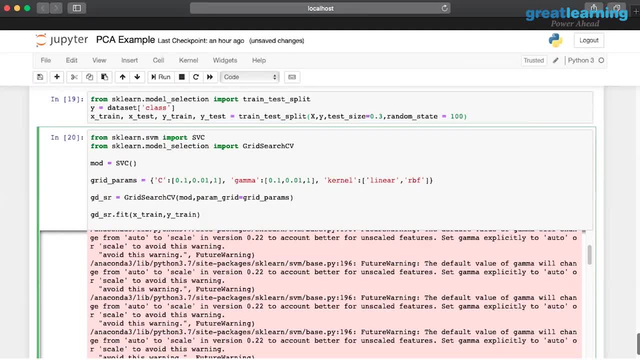 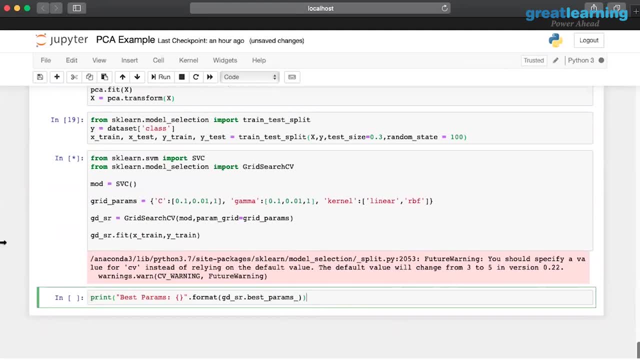 You can remove gamma. if it's taking time, No issues. Yeah, I think I'll probably leave it and let's see how much, how long it's going to take for running. So once you have the results right, you're going to have this grid search. 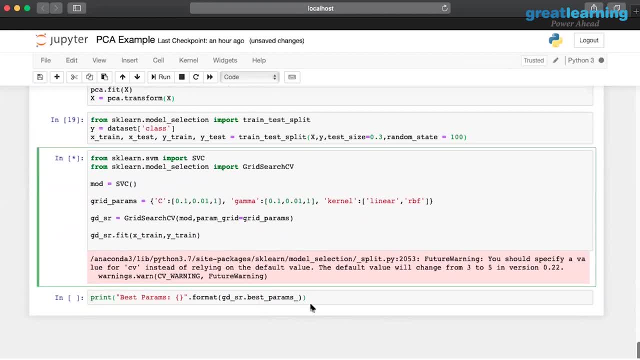 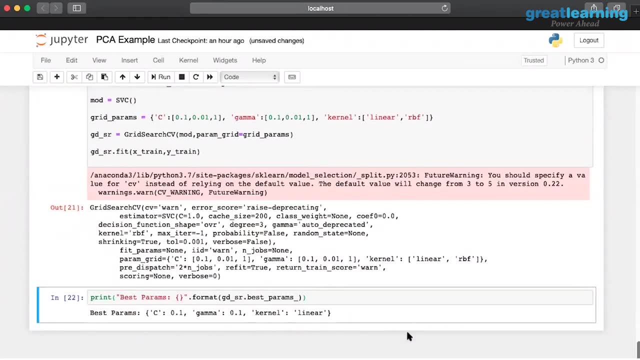 You're going to have this GDSR that's going to carry the results to test the best parameters and best score. Yeah, it's done Now, if you notice, this apparently seems to be the best solution for the current data set. 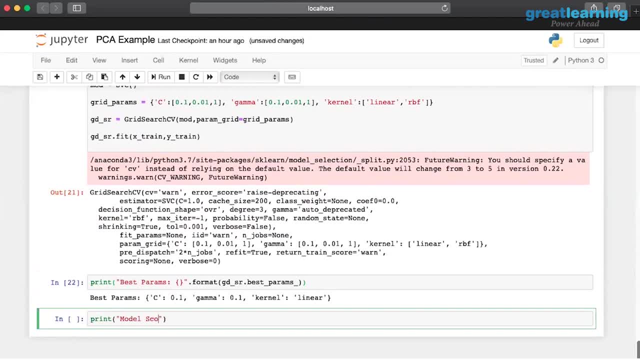 Now, if you want to know why, you can always print the model score in terms of accuracy and then find out. why does it mean or why does it say that this is the ideal solution? So you're getting an 87% accuracy in the result. 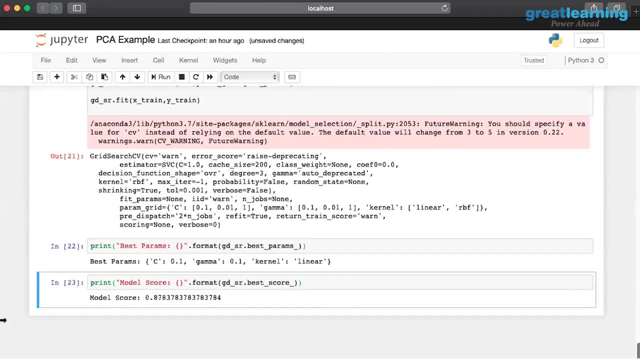 That is the reason it's saying that this is the best parameter for the score. This is the same as the accuracy score, which we Yes. So whenever you execute a model, you have this accuracy score right. You use the matrix dot score. 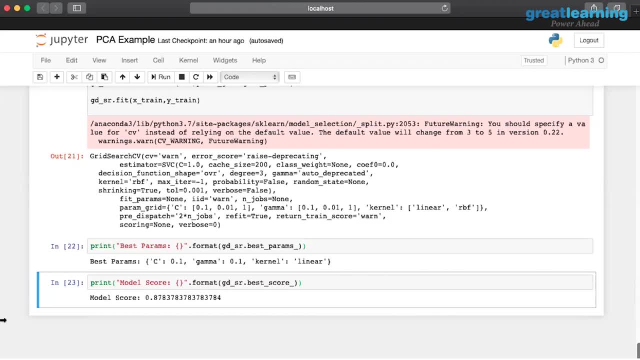 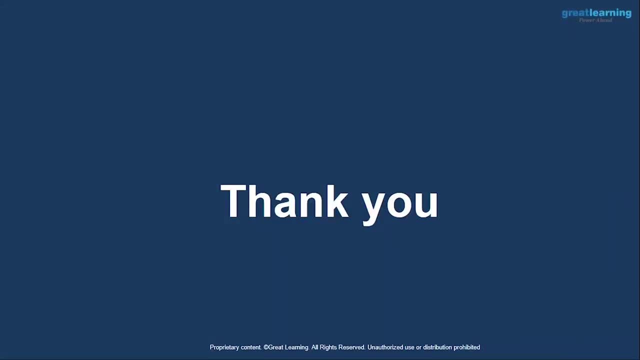 or model dot score. It's the same as that. Yeah, Yeah. So this is how you run a grid search per se. In this tutorial, we have learned about what is unsupervised learning, what is machine learning and also what is clustering. 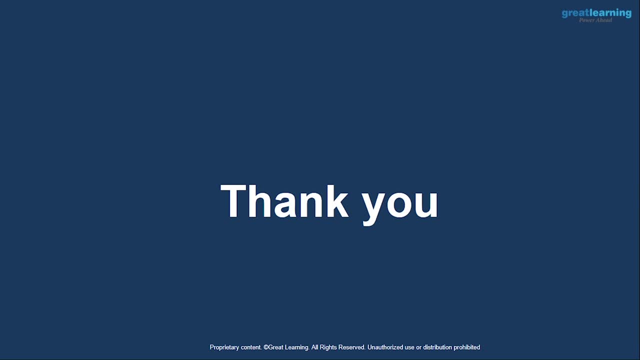 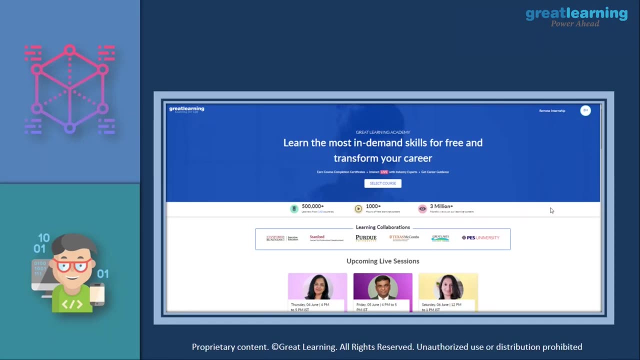 what is PCA techniques. I hope you like the video and do let us know in the comment section what else you want to learn from us. And also let me introduce that Grid Learning has came up with a brilliant idea that is Grid Learning Academy, where you will get almost 80 plus free courses.